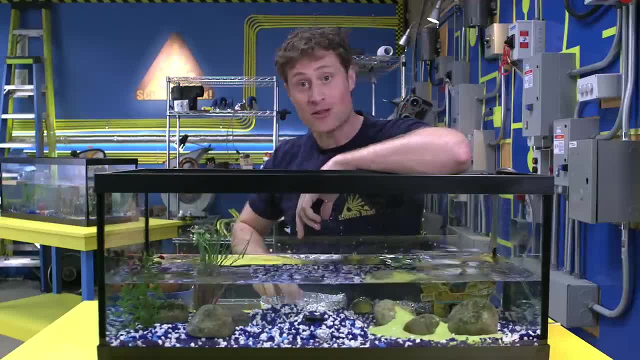 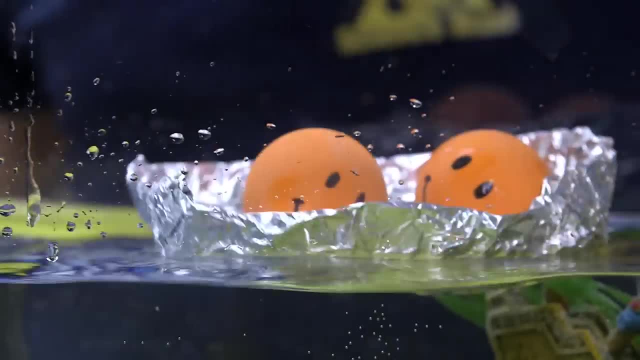 Tinfoil is metal and well it sinks. But if you fold tinfoil into a boat, shape, it floats. And boats don't only float themselves, but they can hold people and people. In fact, there's container ships crossing the ocean at this very moment. 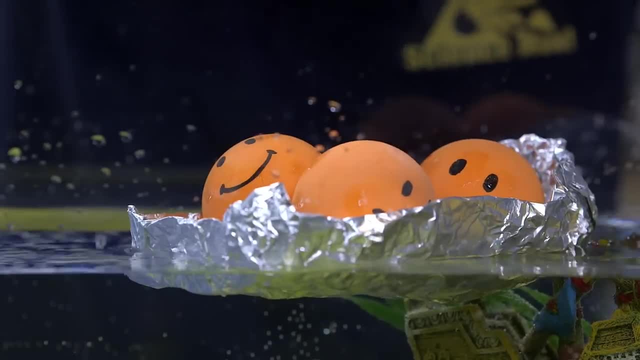 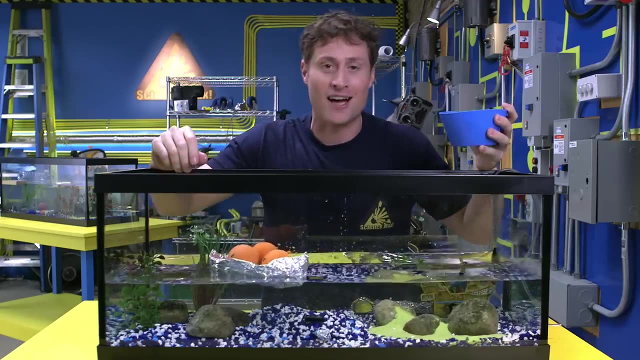 that are holding thousands of tons of cargo, and they're all made of metal which doesn't float- it sinks. So how do boats do it? Are they magic? No, of course not. Boats are science, And here you can be science maximites. 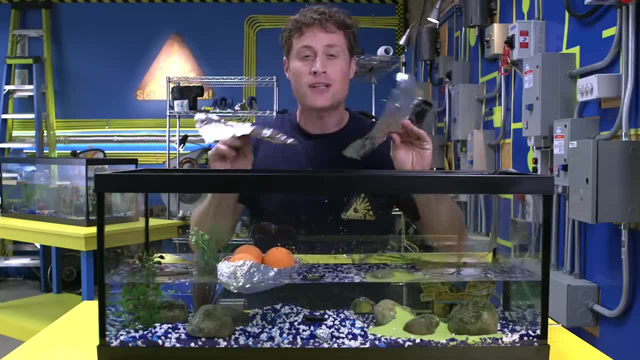 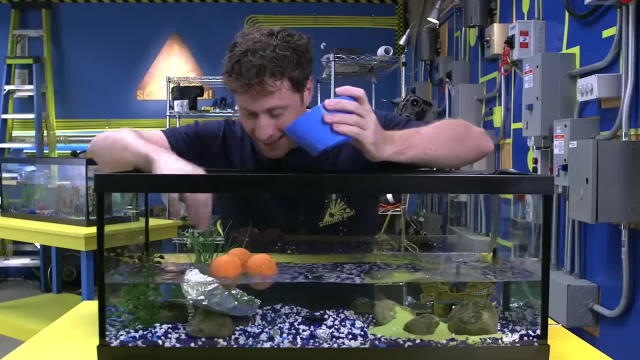 Get some tinfoil and cut it into the same size pieces and fold a couple different shapes of boats and see which one can hold the most weight before sinking. And now it's time to max it out. But before we do, 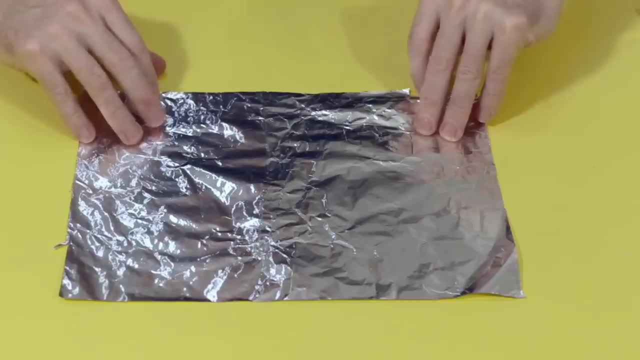 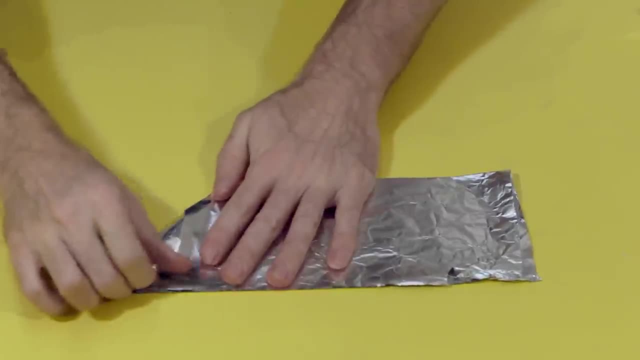 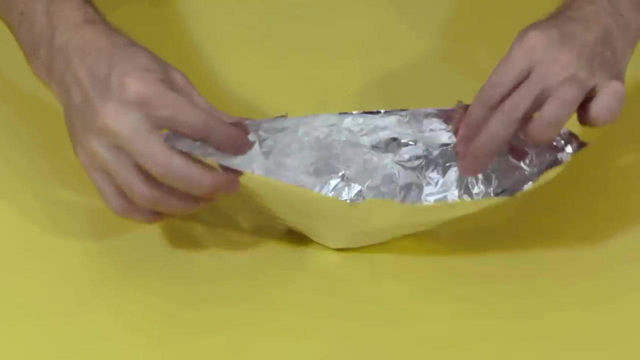 here's how you can fold your own tinfoil boat in less than 15 seconds. First, take a square piece of tinfoil, then fold it in half. Fold one corner down and the other corner down, then open it up and ta-da, you're done. 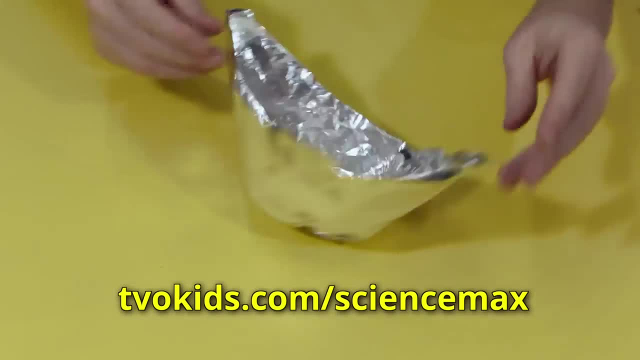 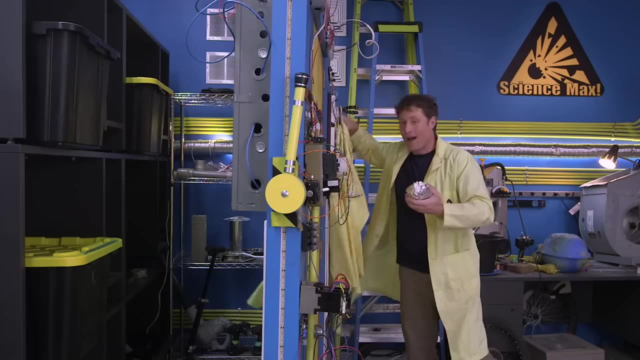 If you want instructions on how to fold a more complicated boat, go to our website. I have a feeling I'm going to need a few extra lab coats for this experiment. Like I was saying, let's max out the tinfoil boat. 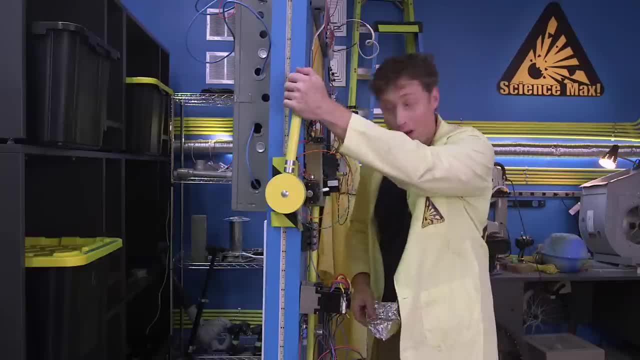 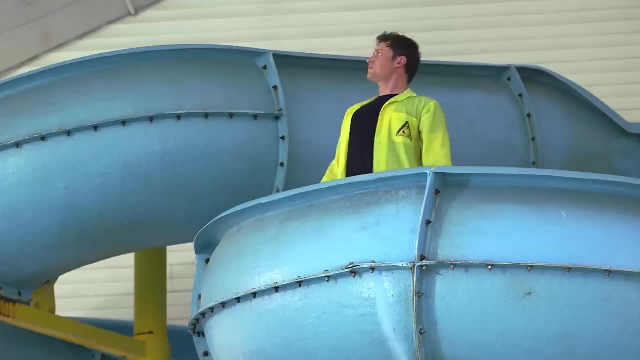 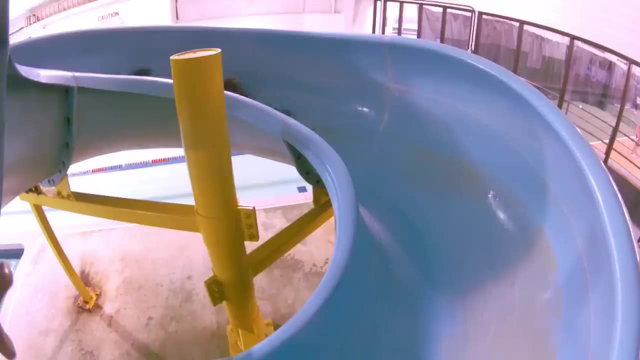 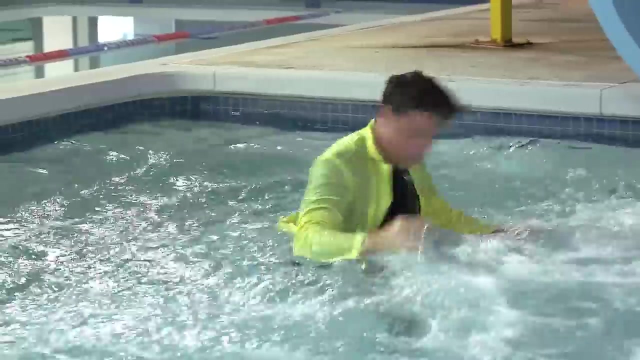 and find out a little bit more about why boats float. Okay, well, I'm here at an indoor pool, Which is not. I wasn't expecting to be in the pool just yet, but this is where we're going to build our giant tinfoil boat. 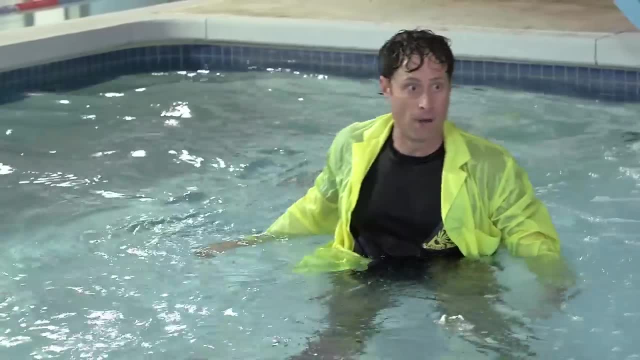 so why not Hoosnia? Oh, Phil, you're wet. I yeah, I thought I was going to come in over there, but I came in on the water sled. I think I had the coordinates wrong. Anyway, this is Hoosnia. 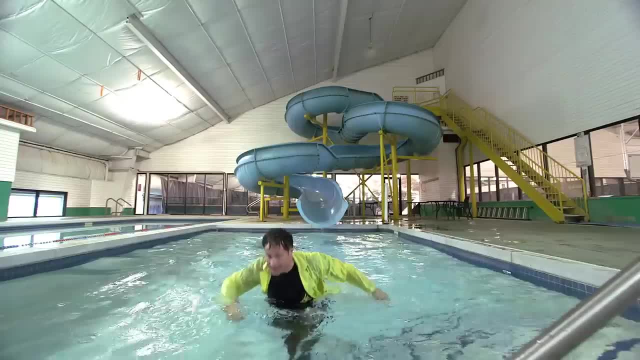 and she's from Let's Talk Sea and she's going to show you how to fold your own tinfoil boat in less than 15 seconds. So let's get started. Okay, I'm going to start with the first step. I'm going to start with the first step. 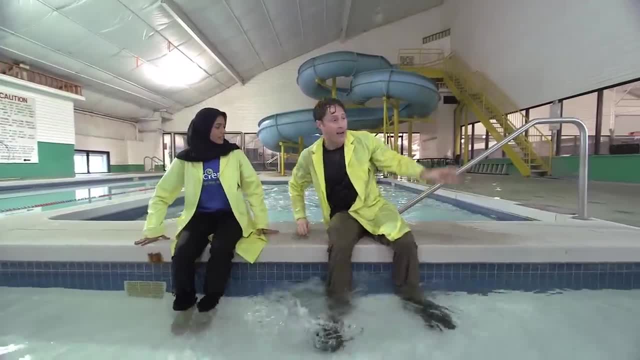 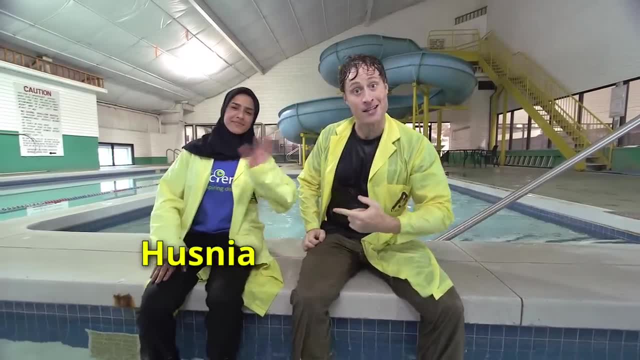 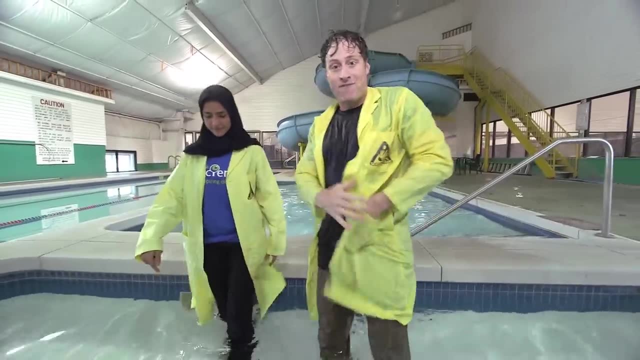 I think I had the coordinates wrong. Anyway, this is Hoosnia and she's from Let's Talk Science, which is all about science, education, right? Yes, Just like us. So you're going to help me max out the tinfoil boat. 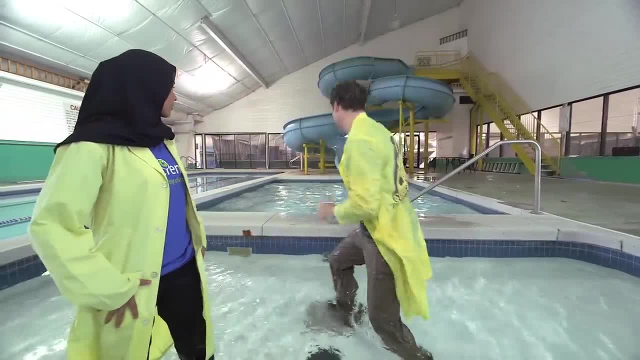 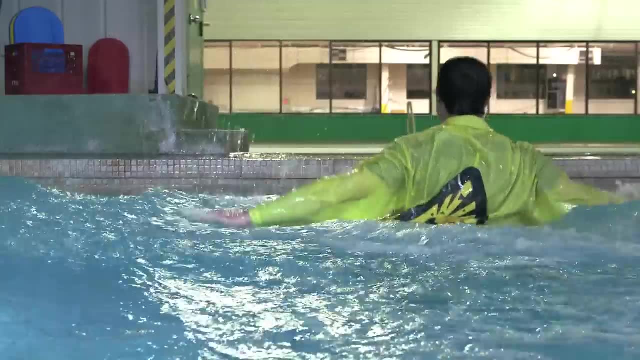 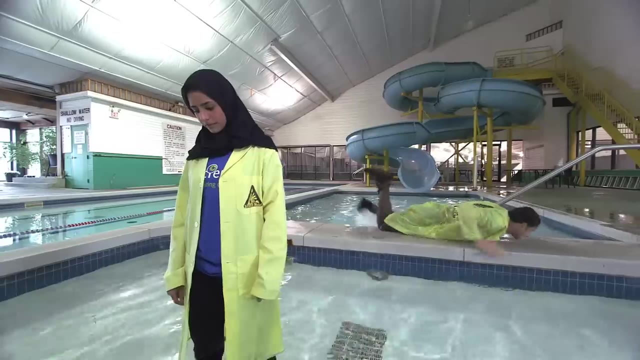 I think I dropped it in the water. hold on, Whoa, You're where There? Here it is, ha-ha, ha-ha. the tinfoil boat. The tinfoil boat, Phil, this is a boat. 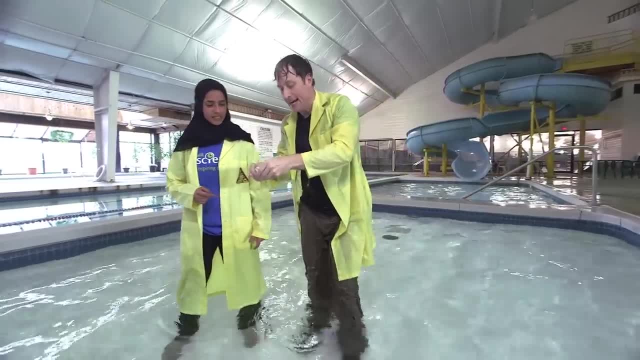 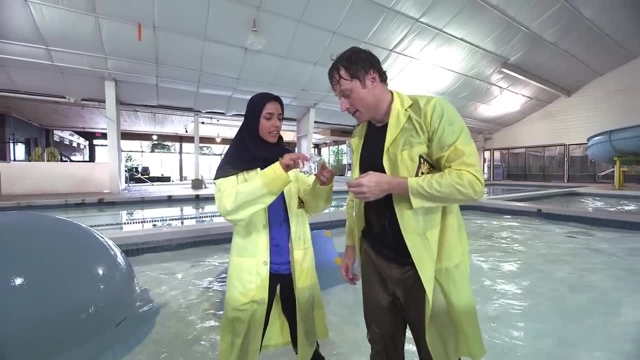 Well, it looked a lot better before I came down the water slide, but that's the idea. and then we make it bigger. What do you think? I don't think it's gonna work, Phil. Well, why not? Tinfoil is very thin. 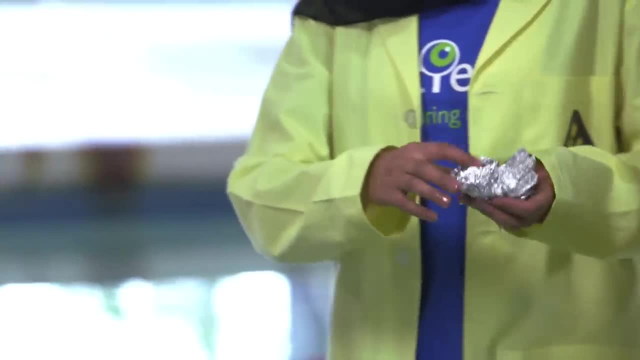 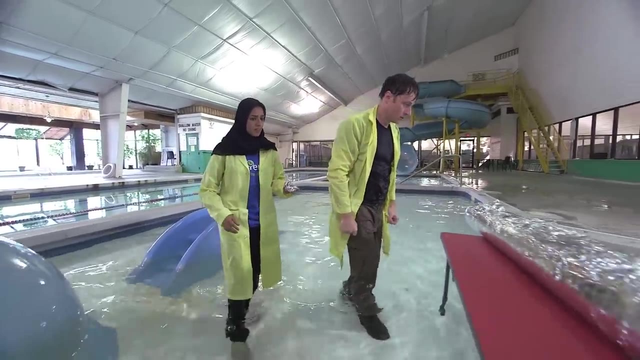 and it might not hold the shape of the boat. Well, I still think we should use tinfoil, though. Why? Well, because the small experiment with the tinfoil and I bought all of this tinfoil. Then let's do it. 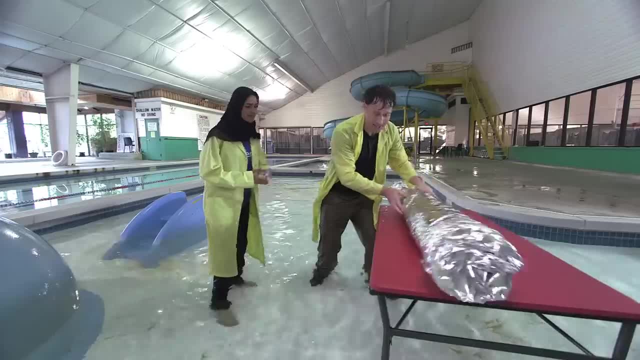 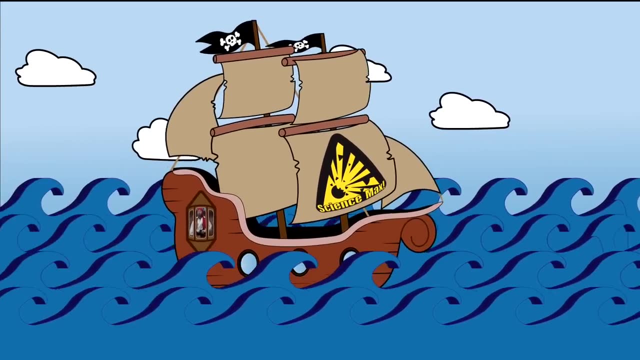 Tinfoil. Okay, high five, I will. I'll take the tinfoil and you take that, and I'm gonna have to dry off at some point. Welcome to Shipbuilding for Pirates. I'm Swubby and I've built some of the finest pirate ships. 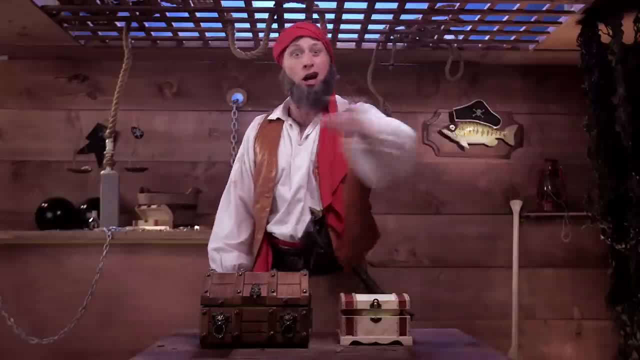 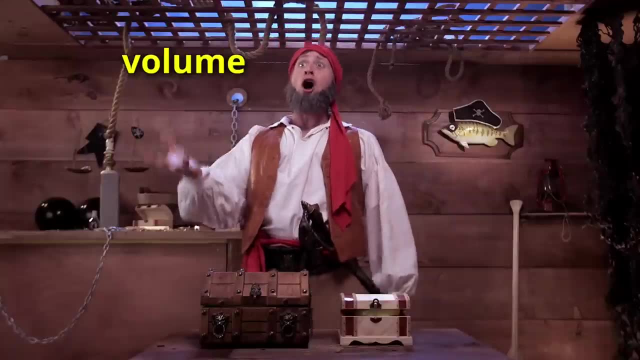 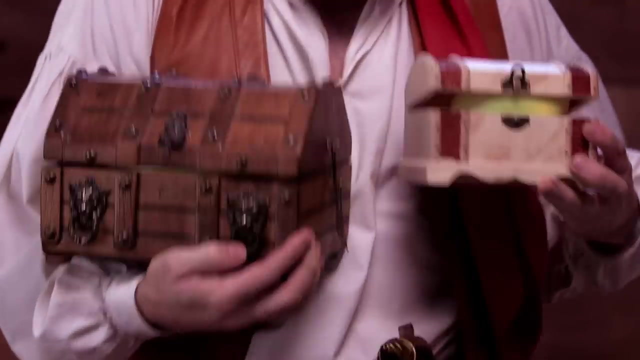 for some of the finest pirates this side of the Caribbean, and I can teach you to do the same, But first you need to know your basics. Massive And volume. Let's start with volume, But not that kind of volume. Which of these two chests do you think has more volume? 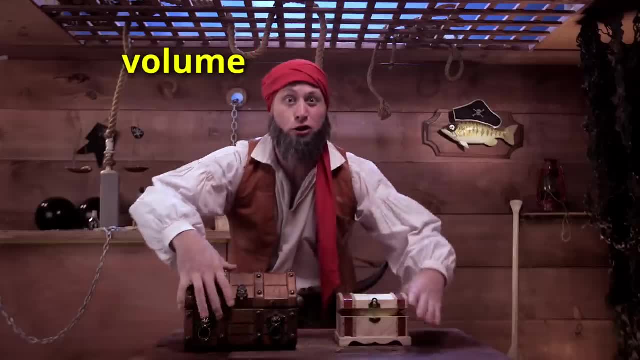 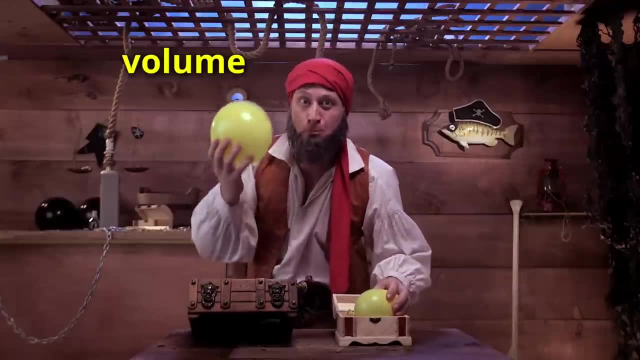 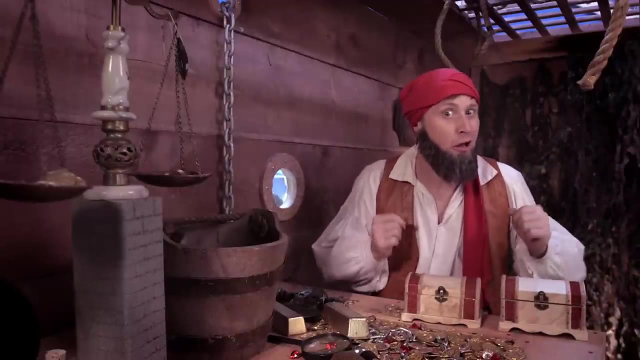 Right, this one here. Which of these two balloons do you think has more volume? Right, this one here. Volume is how much space something takes up. Which of these two chests has more volume? That's right, they're the same. 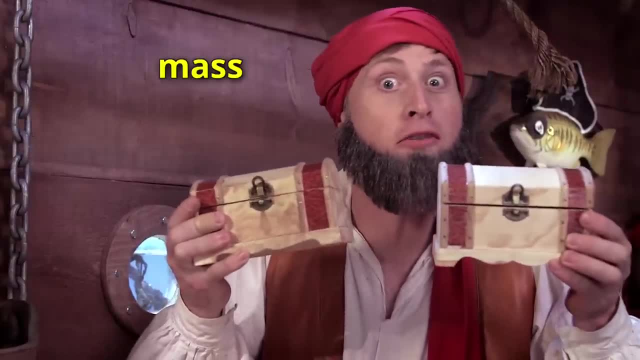 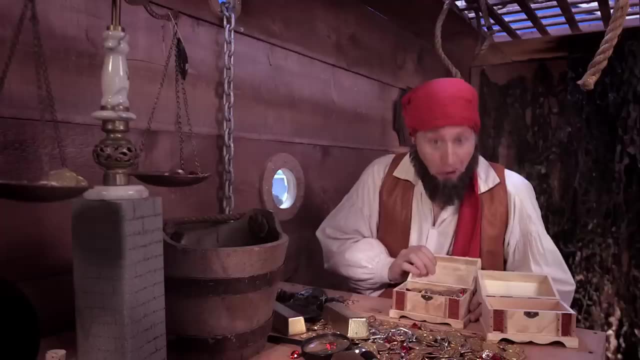 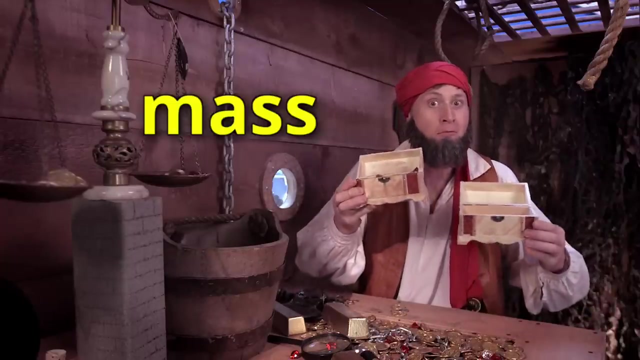 But which of these two chests has more mass? Which is heavier? Hard to tell, isn't it? But what if I told you that this one was empty and this one was full of treasure? Oh loonies. Now which one has more mass? 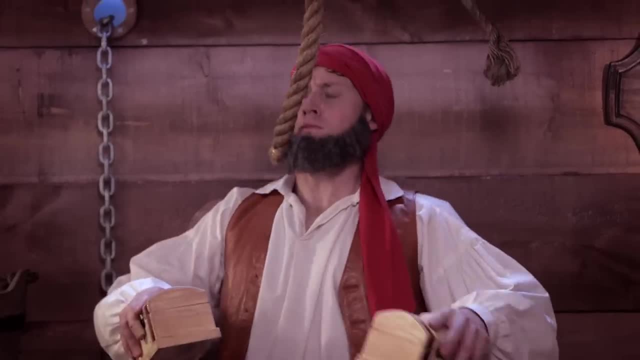 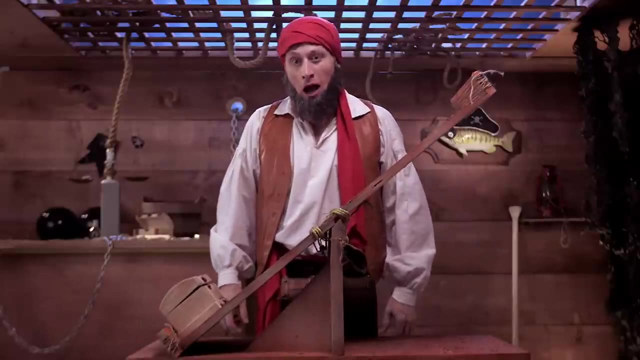 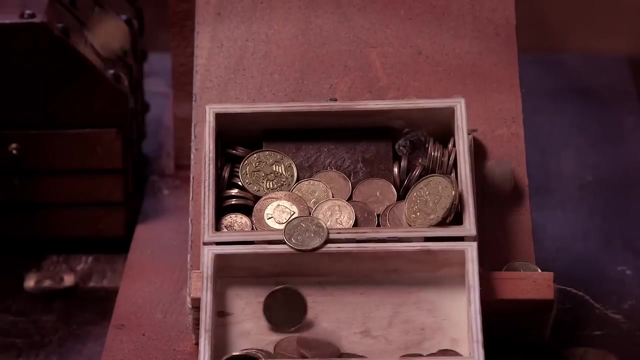 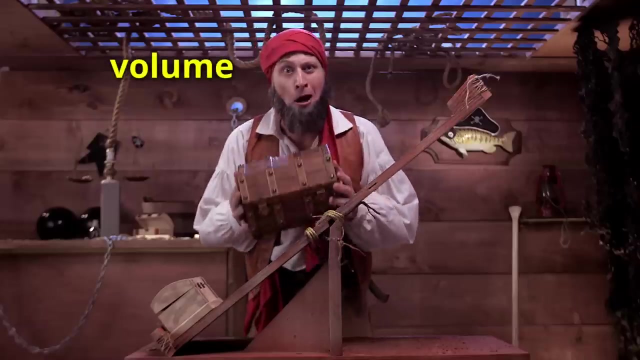 That's right, this one, These two chests have the same volume, but this one has more mass. This chest has more volume than that one, but this one- my loonies- that chest- does not have as much mass. Volume is how much space something takes up. 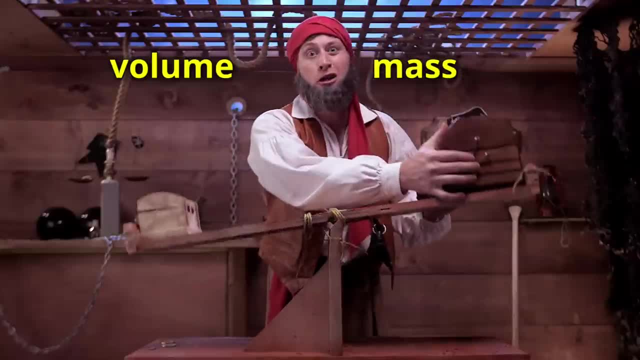 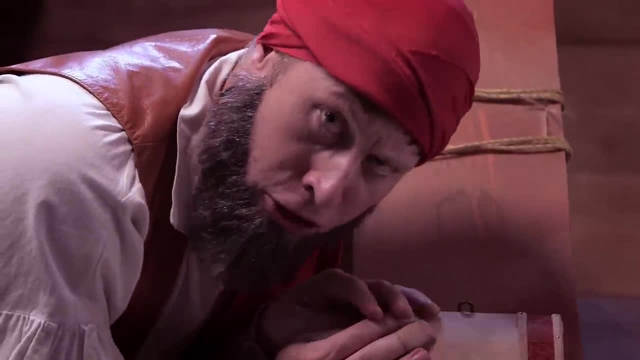 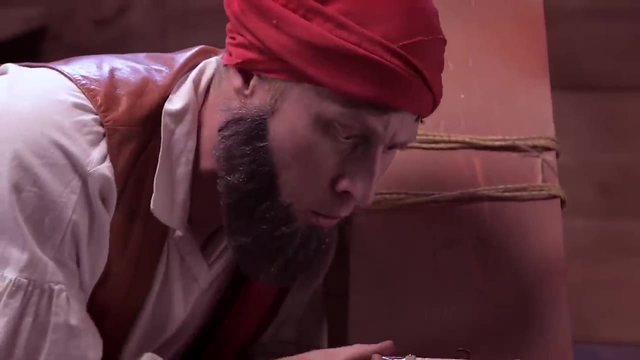 and mass is how heavy something is, And when you look at them both together, you're looking at density. Join us next time on Shipbuilding for Pirates, and then we'll look at how volume, mass and density work together to make something float. 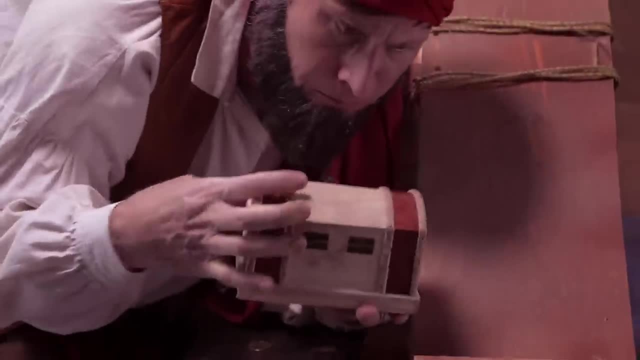 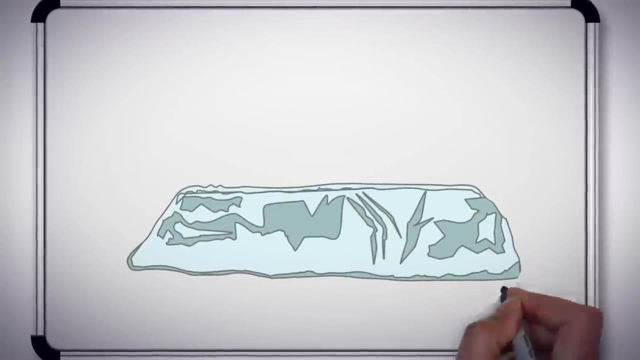 Oh, my precious, precious loonies, Are you all right? my pretties. They can't talk so I'm not sure what they're saying. So Hoosney and I get to work constructing a large tinfoil boat. 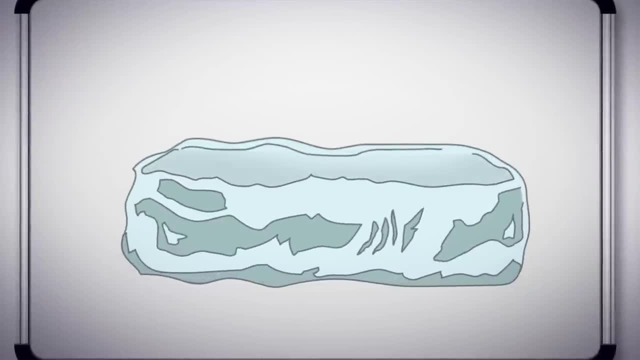 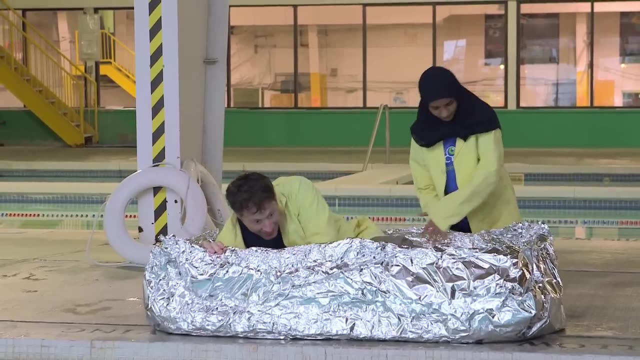 Our first design is just sort of a square folded together out of a very large sheet of tinfoil. Simple, but can I ride in it? Ha ha, ha, ha ha. There we go, A giant tinfoil boat. 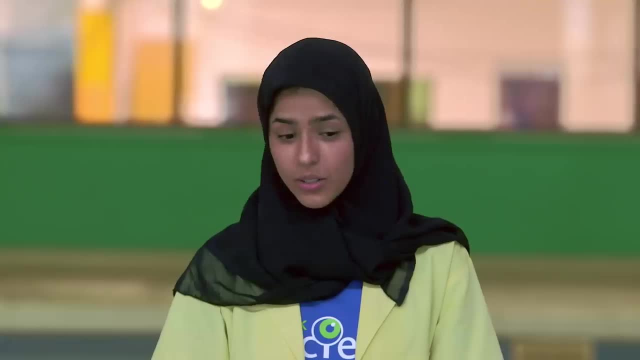 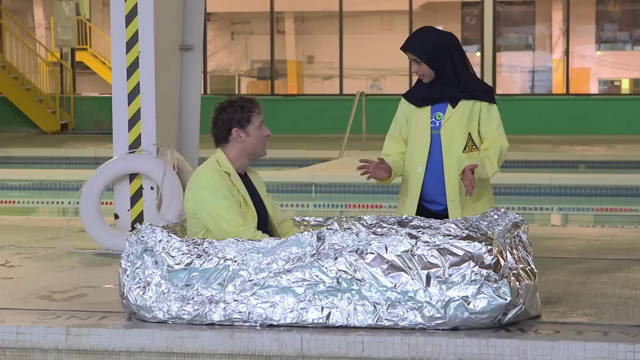 Just my size. Woo-hoo-hoo-hoo, I don't know if it's going to work. It's too thin. You think it's too thin? I feel like, yes, Well, what should we do? Do you want to test it? 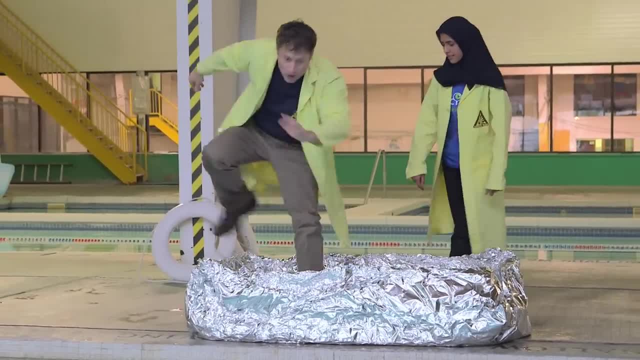 Let's test it. OK, good idea. So here's the most important question: Do you want to test it or should I test it? No, no, no, you test it. All right, here we go Putting it in. 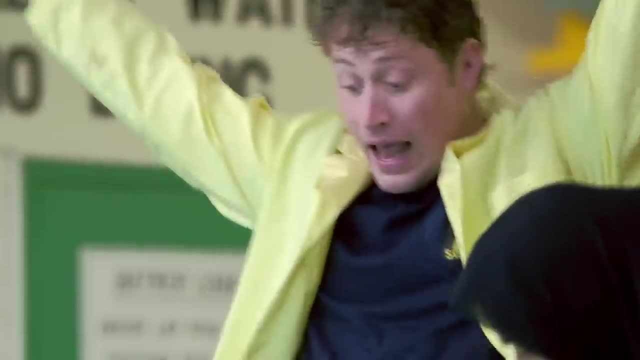 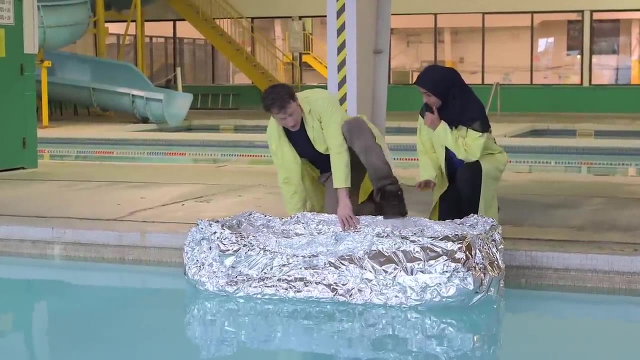 First test: does it float on its own? Yeah, Floats on its own, no problem. If I just get in very carefully, Then it will work fine. See if I'm careful about how I get in. No, it's fine. 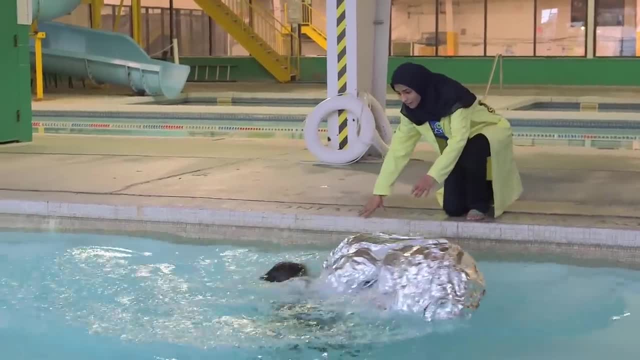 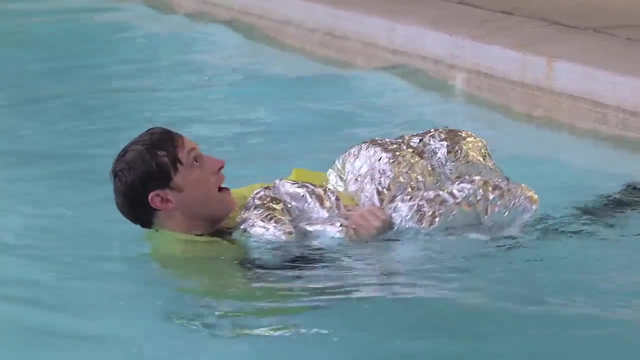 See, if I just get in like that: Oh Phil, Phil, are you? OK, Wait a minute, Wait a minute, It's sort of. it's sort of. no, that's just air. You know what went wrong? 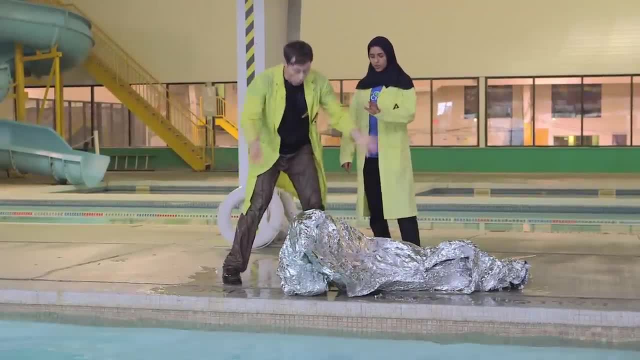 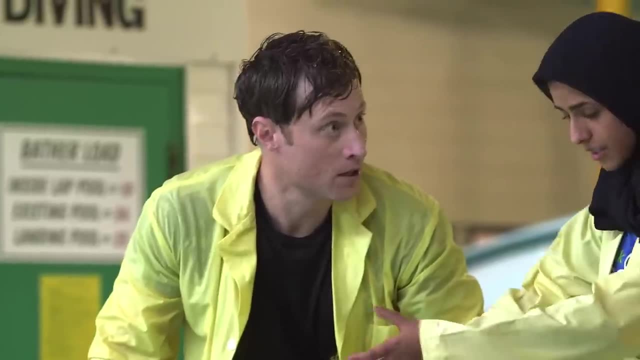 It wasn't boat shaped. I think if we make it look more like a canoe- because canoes float- if we make it look like a canoe, it'll work great. No, no, no, no, Phil, We need some support. 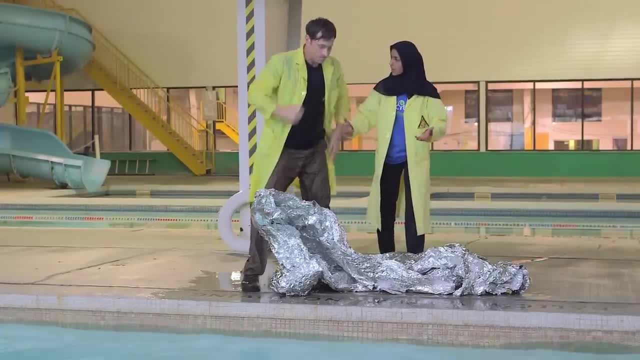 If we add a couple of structures in between, then we add support to it. I'll tell you what let's make: a boat like I want to make and a boat like you want to make, and we'll see whose is the best. 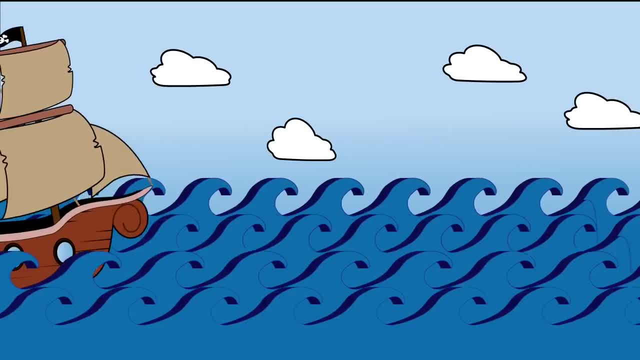 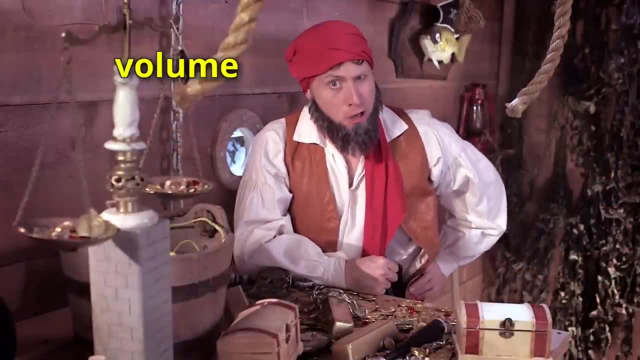 That's a good idea. OK, let's do that. All right, let's do it. Welcome back to Shipbuilding for Pirates. I'm Swobby, and now we know what volume means, what mass means, and that together it can tell you something's density. 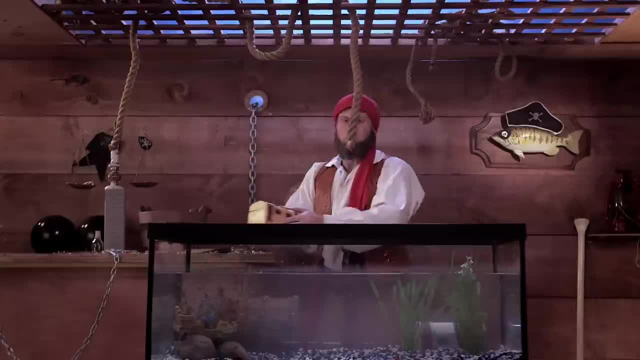 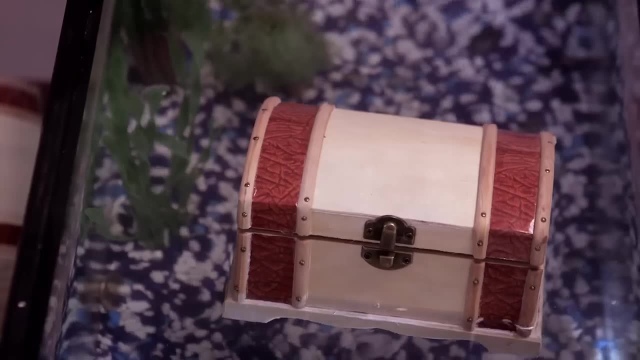 Now let's find out why things float. Let's, Let's say we're out to sea and my treasure chest gets swept overboard. Oh no, But it's all right. It floats because it pushes enough water out of the way. 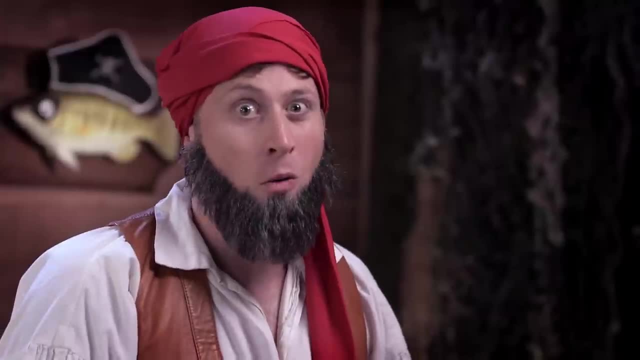 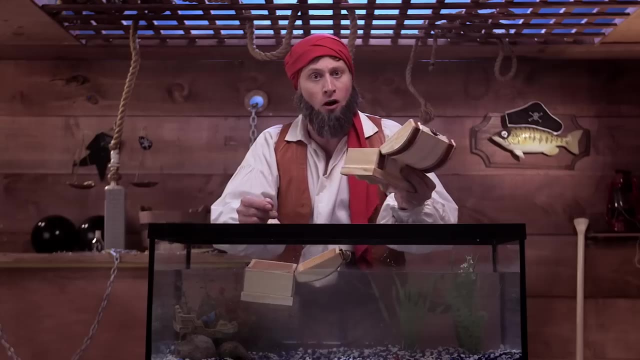 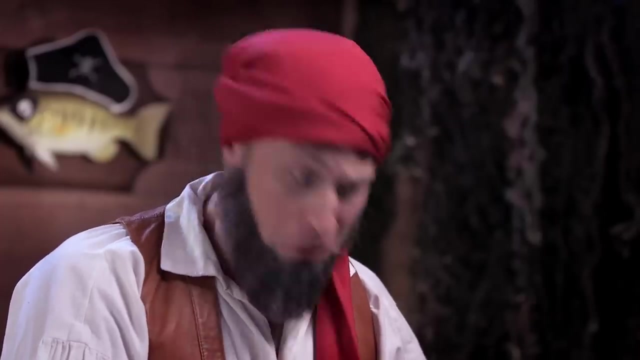 displaces it to carry its mass. But what if my treasure chest had more treasure in it? Well, we're giving it more mass, but not more volume. Too much mass and not enough volume, and it will sink. Oh no, my loonies. 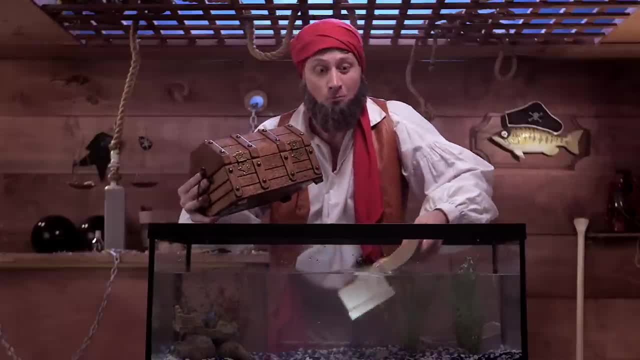 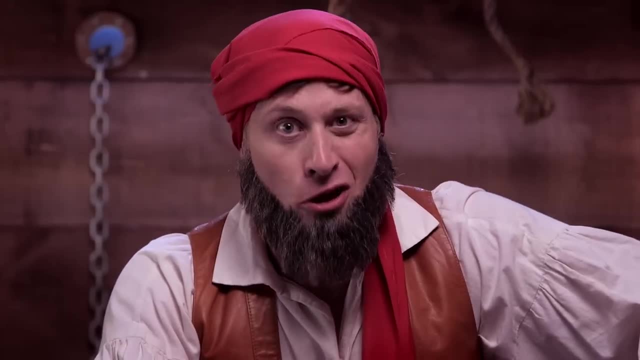 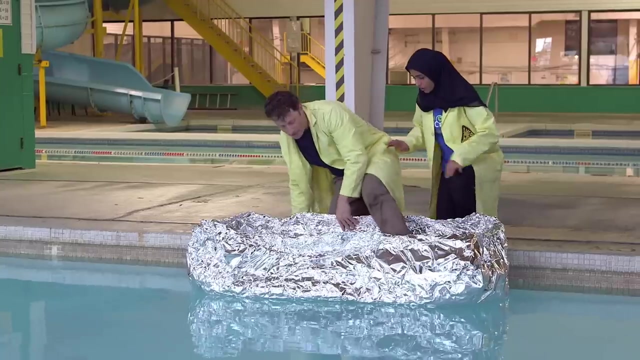 You need more volume if you want to float more mass, And that is why things float. I'm Swobby, and thanks for joining me on Shipbuilding for Pirates, So the first version of the tinfoil boat didn't work out too well. 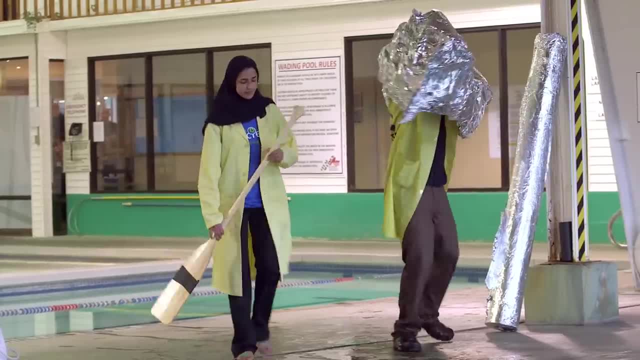 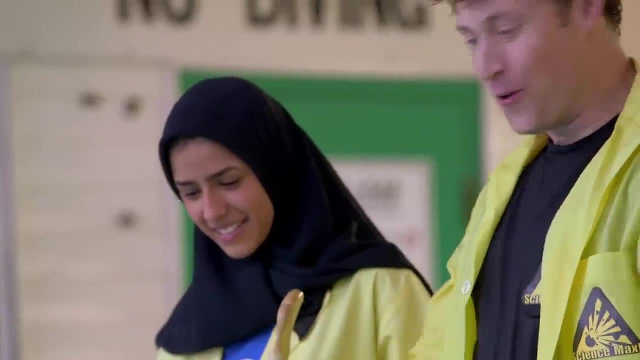 Like that. But my idea is to build a tinfoil boat more like a canoe, to see if a different shape makes any difference. Tinfoil canoe- Very Canadian, Very Canadian. The canoe part. anyway, I don't know about the tinfoil part. 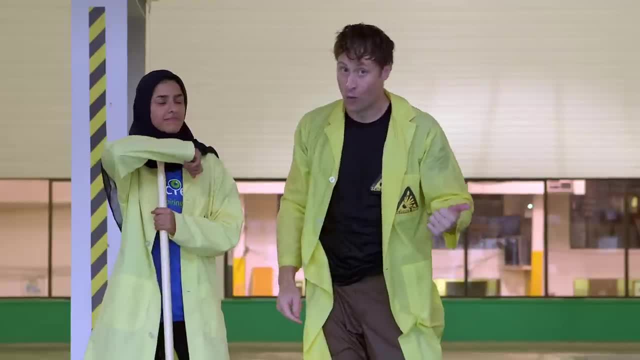 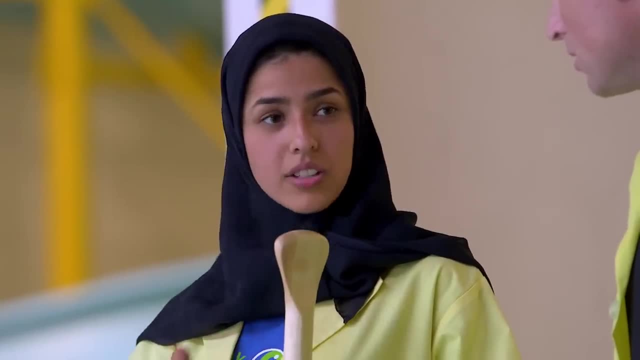 So Husni and I had a bit of a disagreement of why the last boat didn't work. I thought it was because it wasn't shaped enough like a boat, So this one looks like a canoe. What I thought is that it requires some structure. 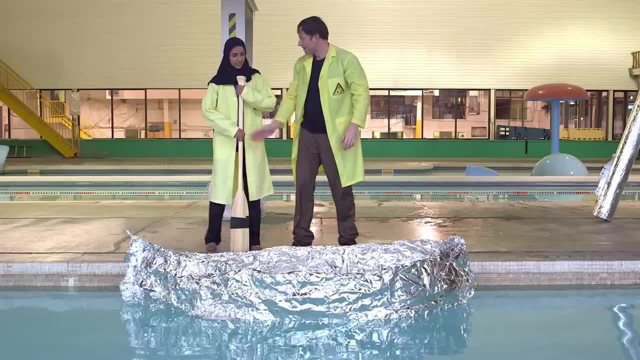 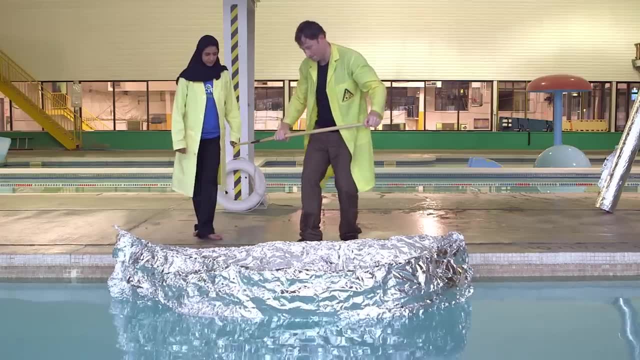 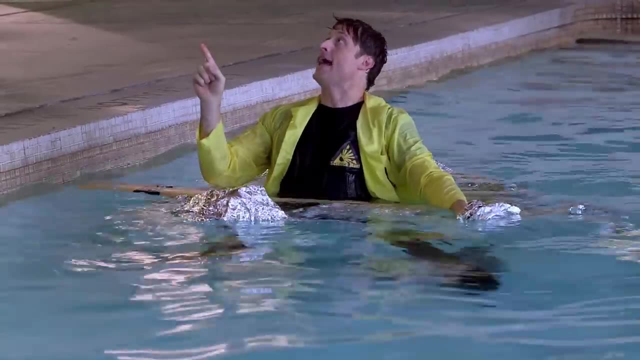 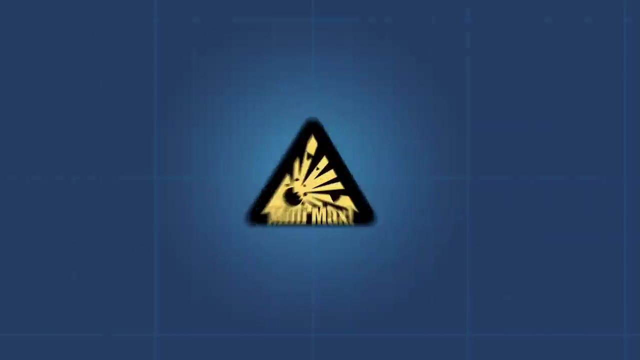 Structure so that it wouldn't fold together. That's right, And we'll see how it goes. All right, All right, here we go. Did it work? No, OK, Your idea. next, Mini Max. Did you know it's easier to float in salt water? 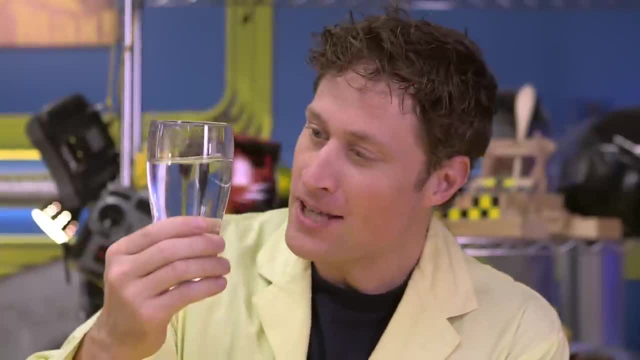 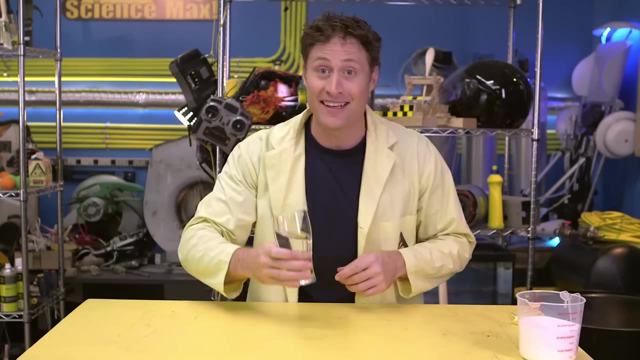 like in the ocean than it is in fresh water, like a lake or a pool. That's because not all liquids are created equal. They have different densities. This is fresh water, or it doesn't have anything in it, And this is sugar. 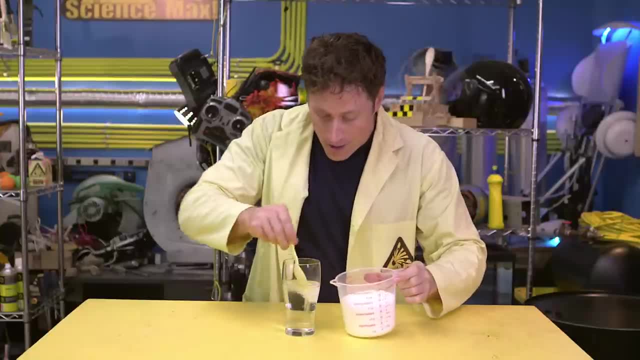 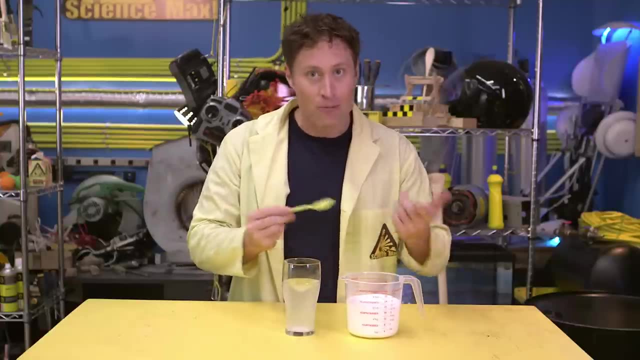 If I was to put one scoop of sugar in this water and stir it around until it dissolves. now this liquid is more dense than before I put the sugar in. Here's an experiment you can do at home using liquid density. This glass just has regular water. 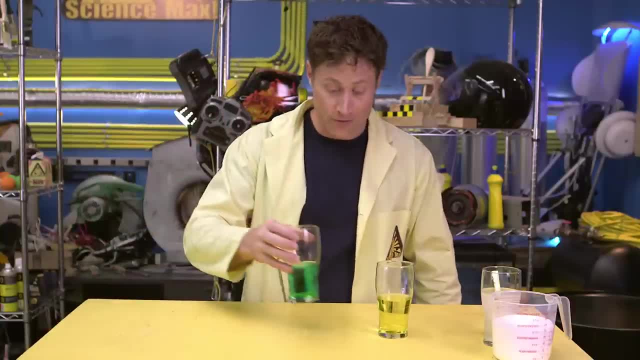 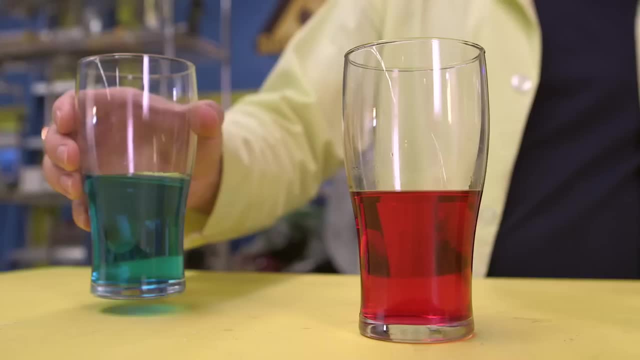 with yellow food coloring in it, This glass green food coloring and half a cup of sugar in it. This one has a full cup of sugar in it And this one has two cups of sugar in it. Now, when you do this at home, you'll definitely 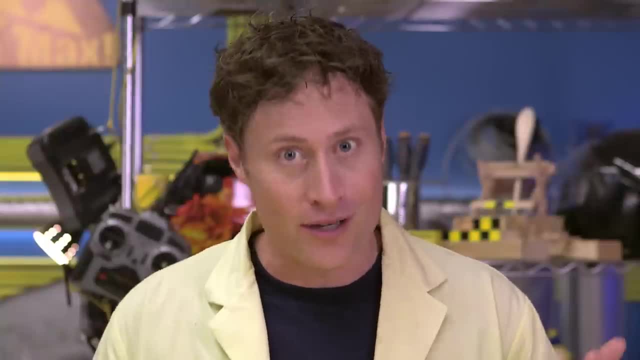 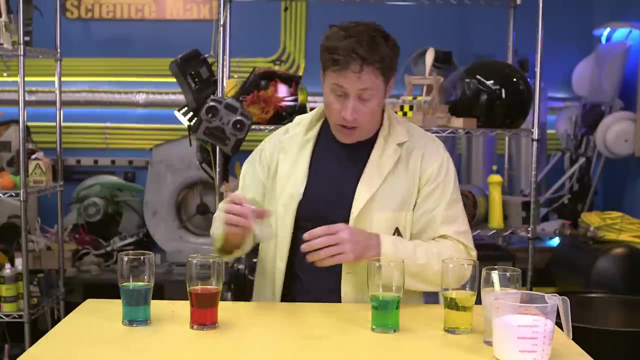 want an adult to help you because you have to heat the water. if you want to dissolve that much sugar in one glass of water, I'm going to put them all in one container. You can do this at home, And when you do, I suggest you use a very small container. 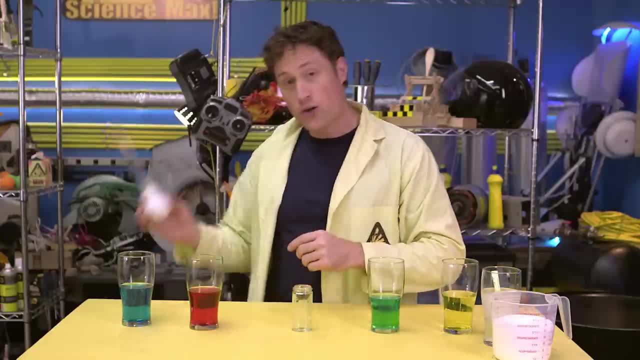 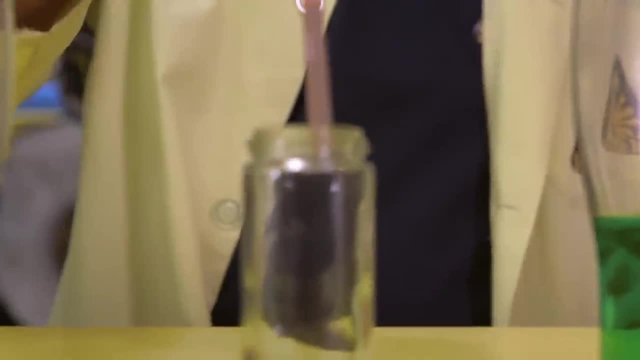 because you have to be very careful when you put the layers in. You can use a turkey baster or a straw. When you put your finger on top, the air pressure will hold the liquid in and you can just drop it in. But these kind of take some time. 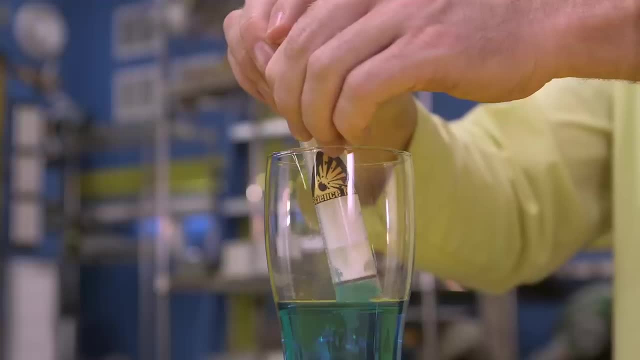 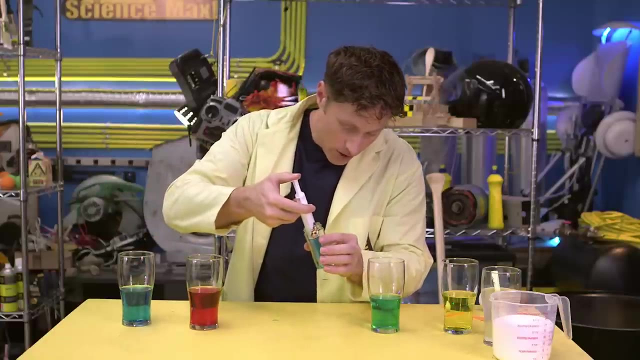 so I'm going to use the syringe of science. I'm getting ready. I'm going to use the most dense liquid first, because that's the one that's going to want to be on the bottom. I carefully put it on the bottom of the container. 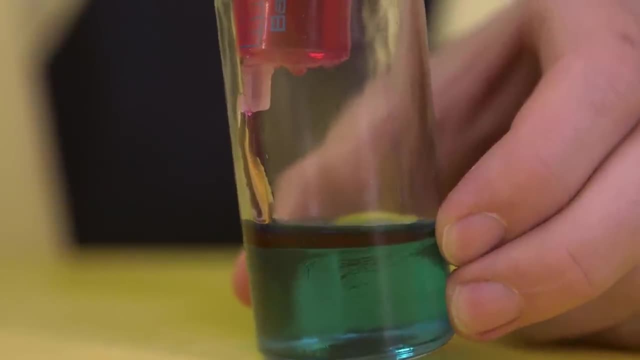 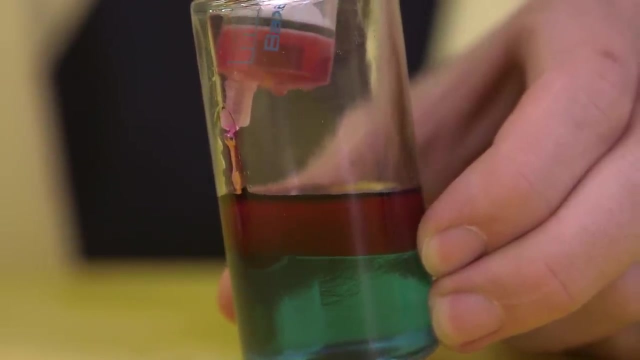 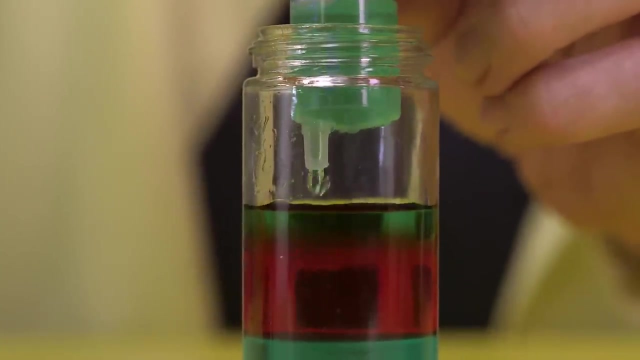 The next layer. be very careful. You'll see that the red and the blue aren't mixing because they have different densities. The blue is heavier than the red. We'll add the green And you can see even when it drips into the red. 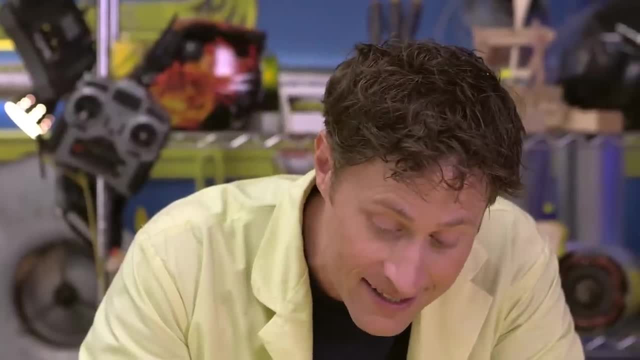 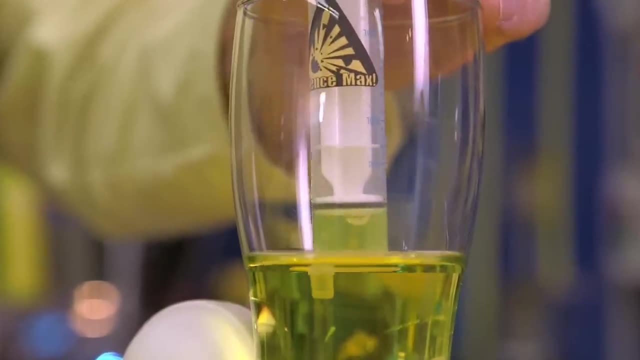 it comes back up to the top because the green liquid isn't as dense as the red liquid, And the denser liquids push the lighter liquid up. And now we're going to add the yellow, which of course has no sugar in it at all. 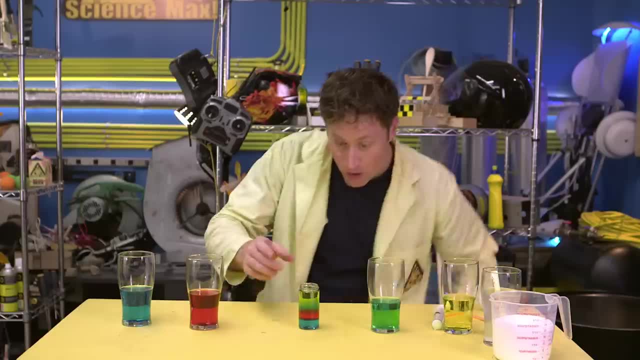 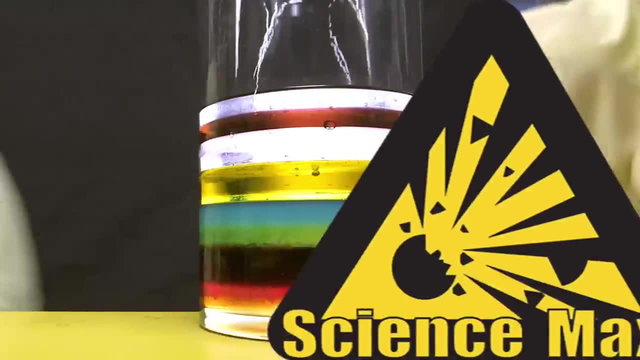 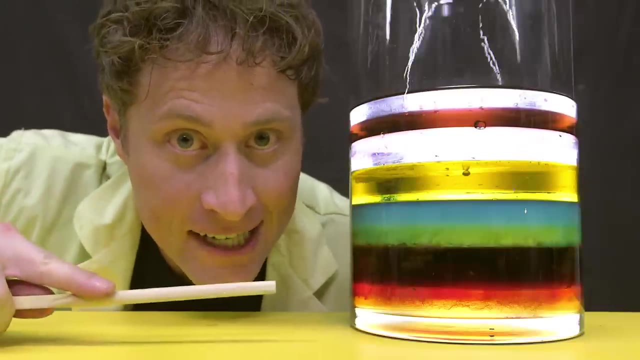 And there you go. All the layers stay separate. If you put it on a light, you can really see it. Liquid densities: Now let's max it out: Ta-da, The longest length of liquid layers, 12 liquids all organized by density. 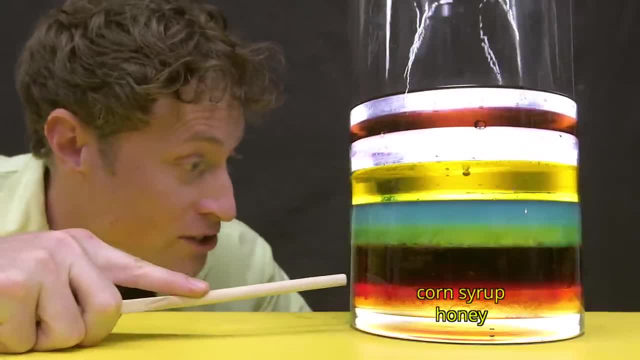 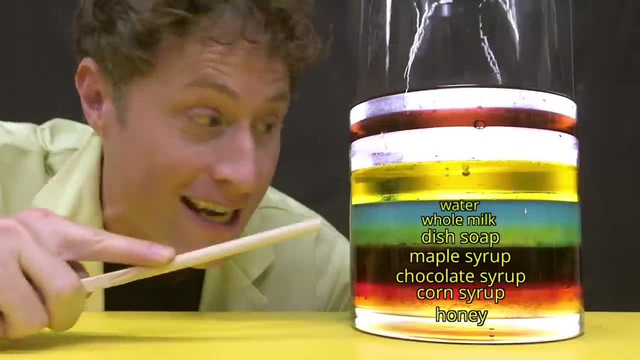 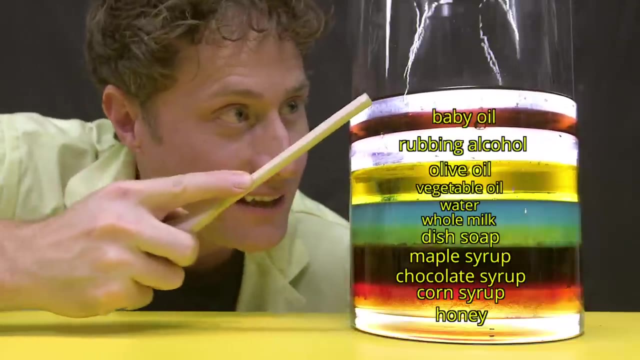 Starting from the bottom, we have honey, corn syrup, chocolate syrup, maple syrup, dish soap, whole milk, water dyed blue vegetable oil, extra virgin olive oil, rubbing alcohol, baby oil and lamp oil. Liquid density: 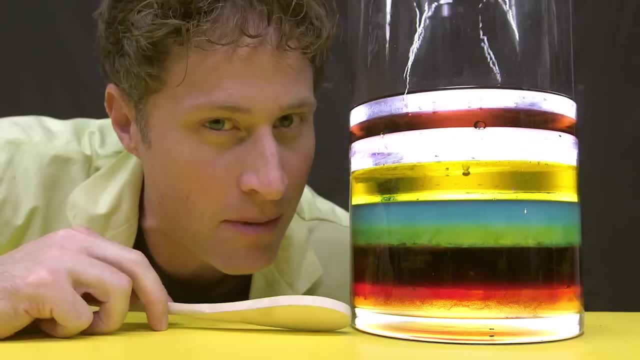 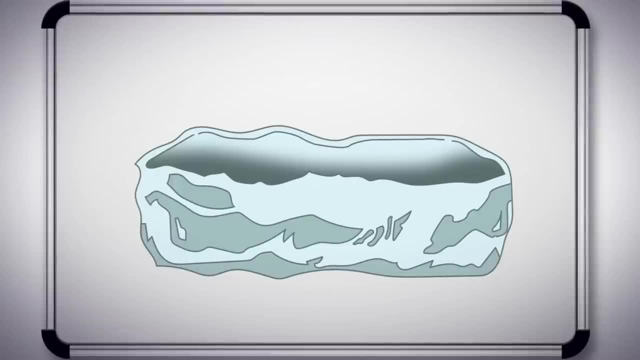 I really, really want to mix it up, but it took me a long time to make this, so I'm not going to. Our first two attempts at a tinfoil boat haven't gone so well. Huznia's idea is to make a tinfoil boat. 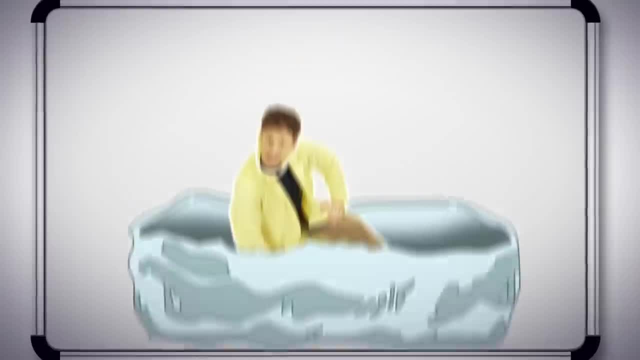 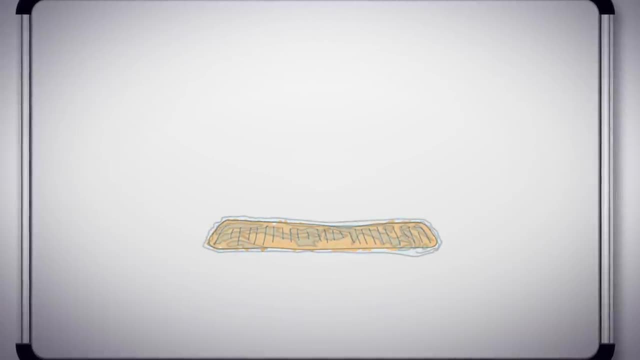 and add some more structure, because the tinfoil just wants to collapse when I get in it. So we start with a large piece of cardboard on the bottom, Then we wrap the tinfoil around it and shape it into a boat. After that we add some supports across the top. 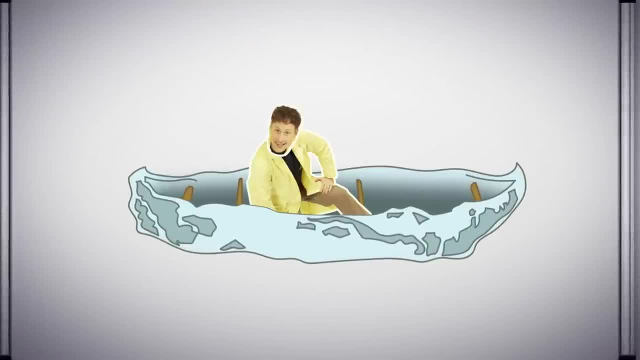 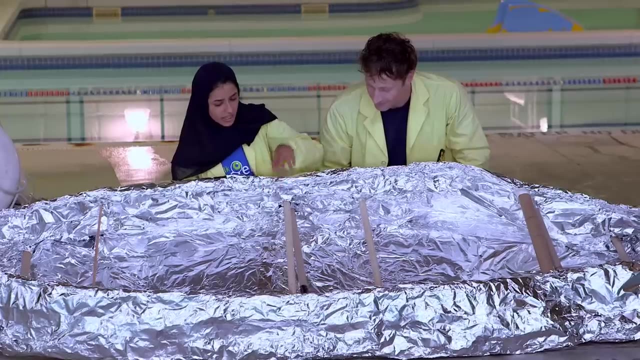 to stop it from folding in. when we add my weight to it, This boat feels a lot stronger than the one I was doing. I told you: So how does all of this work? So we got some support using broomsticks and then some cardboard paper. 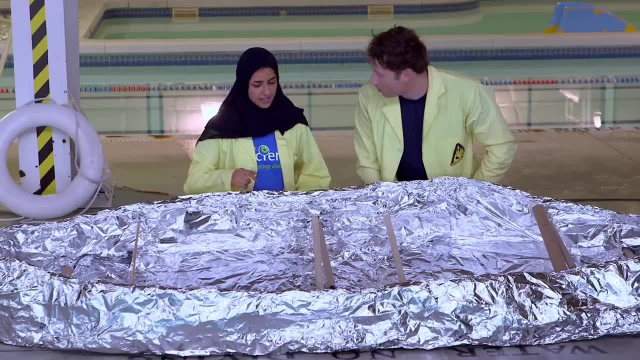 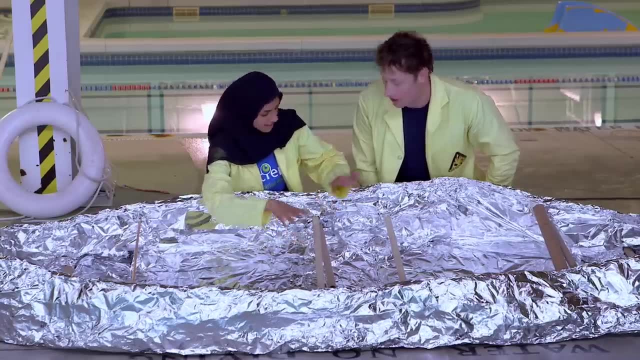 and then underneath we have cardboard. And so how will all of this help the boat not sink with me in it? Right, The broomsticks will prevent it from folding this way and you won't sink. The cardboard will prevent it from folding this way. 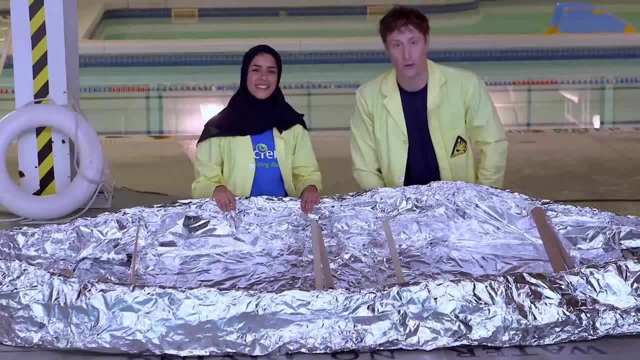 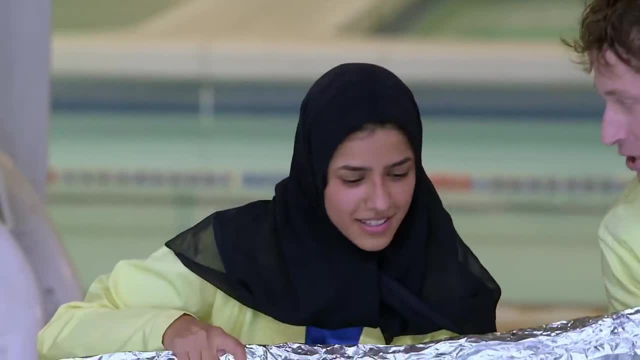 and you won't sink again. Not sinking is my favorite thing to do in the tinfoil boat. All right, so let's try it. Let's do it. Are you going to get in this one? I'll tell you what, Phil. 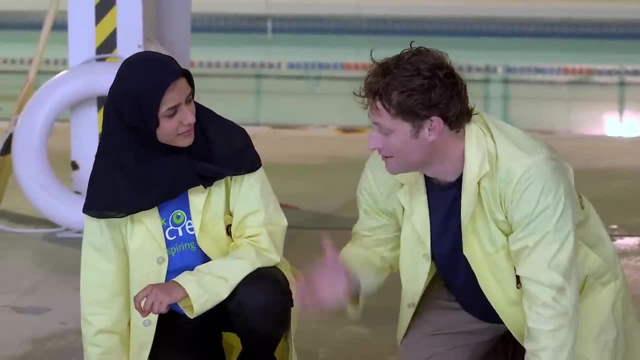 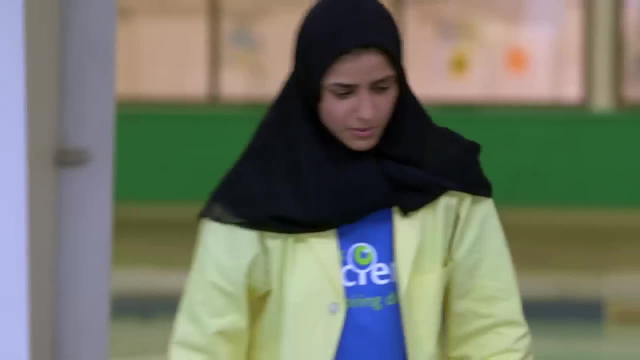 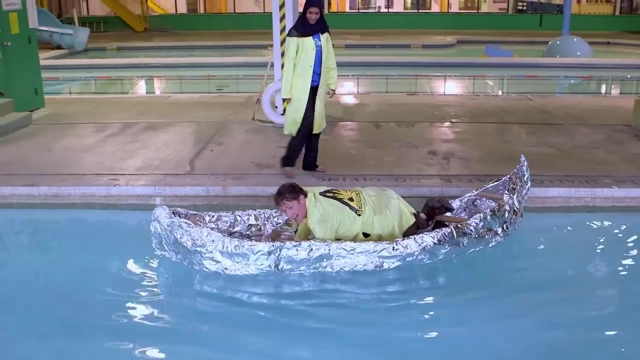 If you get in and you don't sink, I'll go after you Deal, All right. All right, here we go. It's sort of working, Oh no, Oh no, water's coming in. It's sort of working. 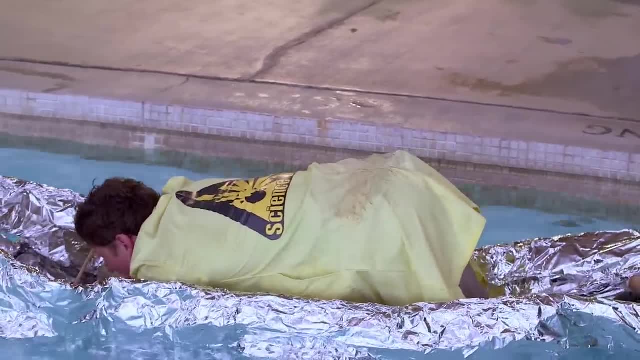 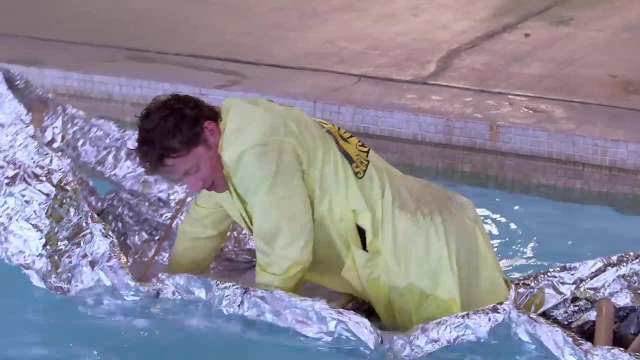 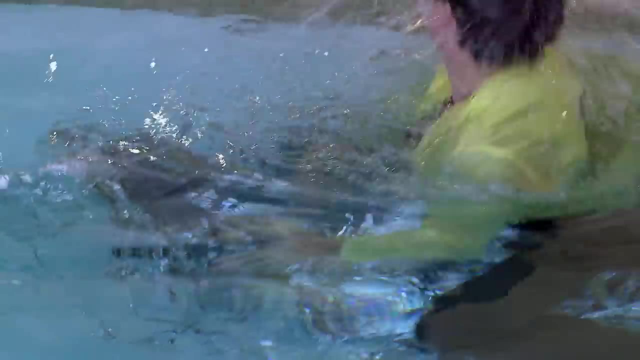 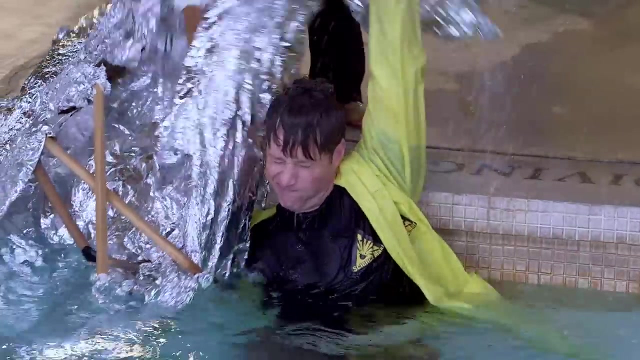 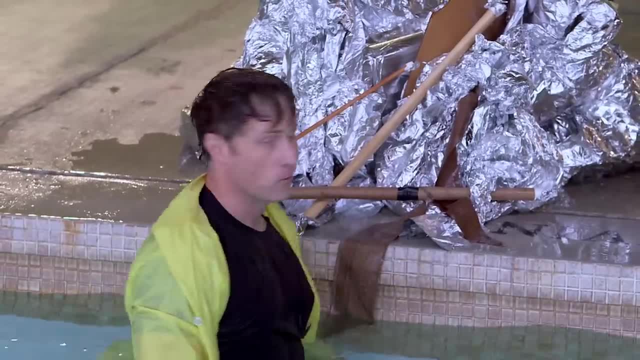 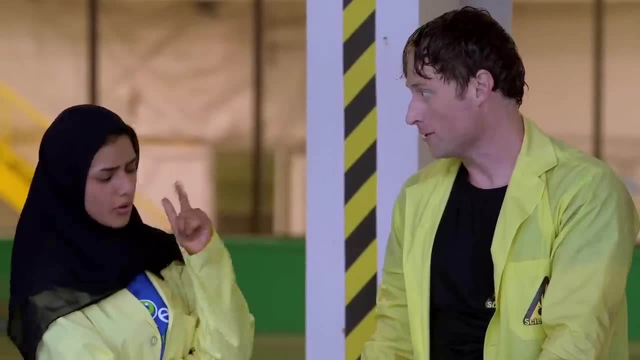 of water. I don't know if fixing it is in the cards. I think we're going to have to build another boat, Mm-hmm. So what do you think we should do? Let's add more structure, More structure. Oh yeah. 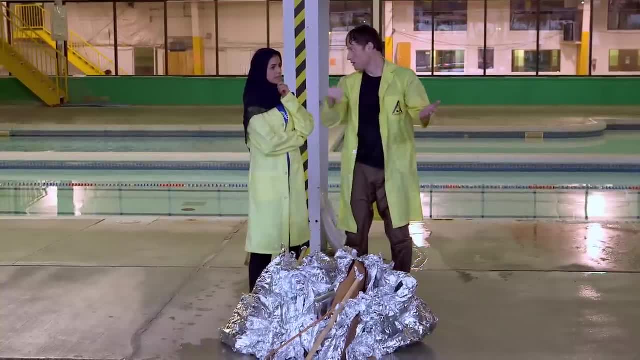 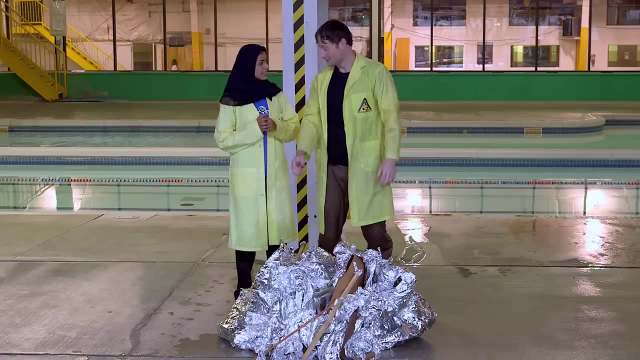 What if we add, like a metal rod around the outside, and maybe some more metal rods and ribs, and we wrap it all in tinfoil and you think it'll work? Let's give it a try. Let's give it a try. 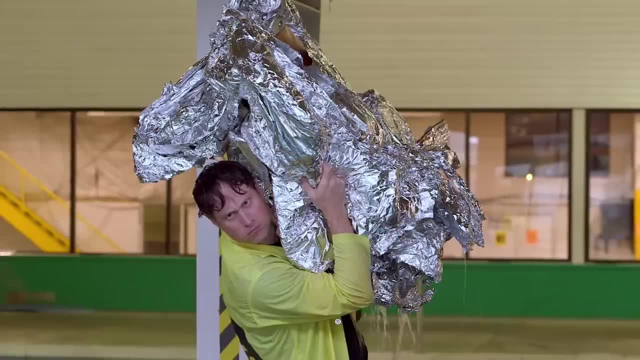 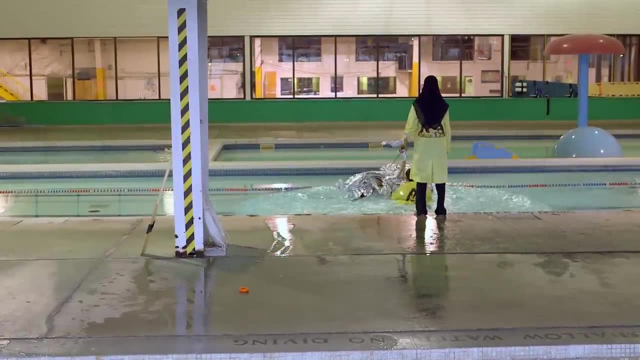 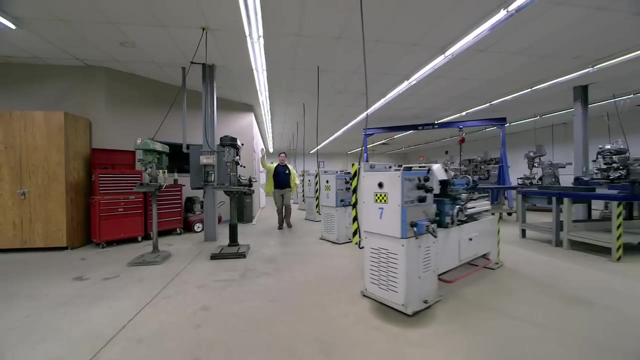 Don't worry about it, I've had this. No, I'll get it. I'll get it. Are you sure We're good? All right, All right, Good, I'm going to get you back. Who wants to do an experiment with diapers? 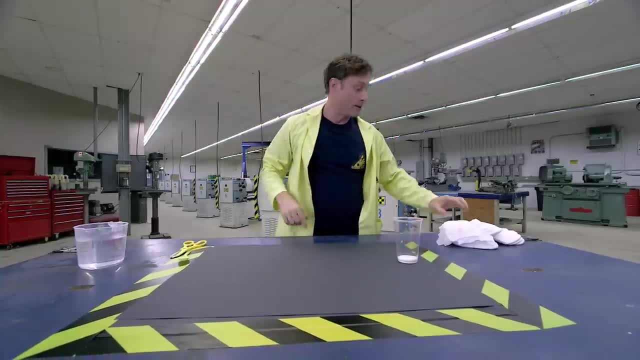 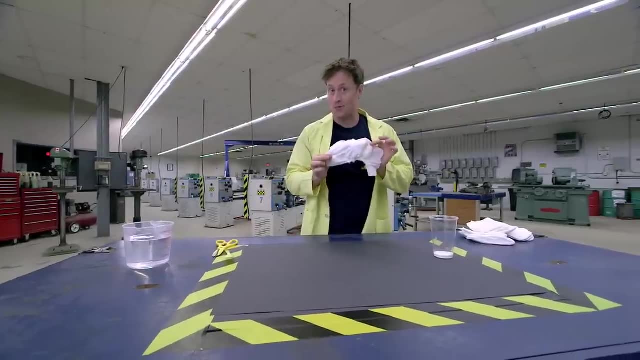 Oh no, I'm serious. You may have a little brother or sister at home, which means you probably know where you can find some diapers. But there are two things you need to remember. First, ask an adult if you can use the diapers for your experiment. 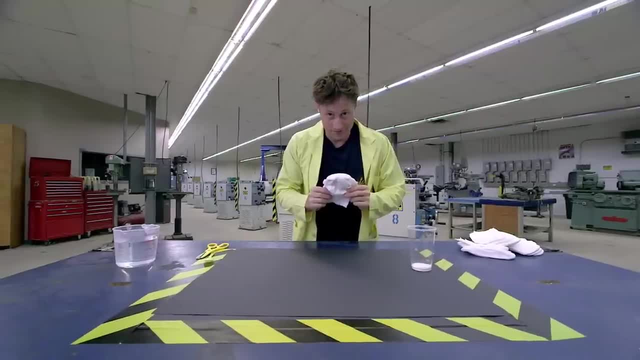 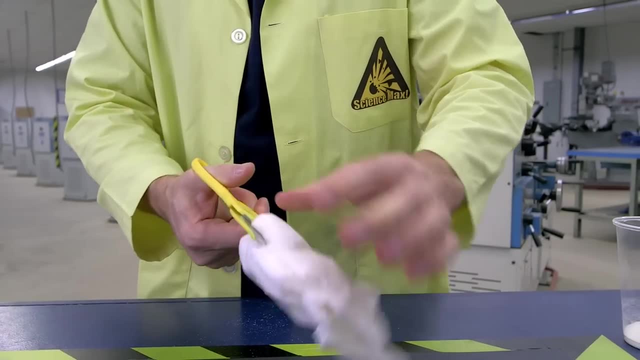 And two only use unused diapers. Okay, Okay, So take the diaper And if you cut it, be very careful. Be very careful. maybe get an adult to help you Over some black construction paper like I have here. 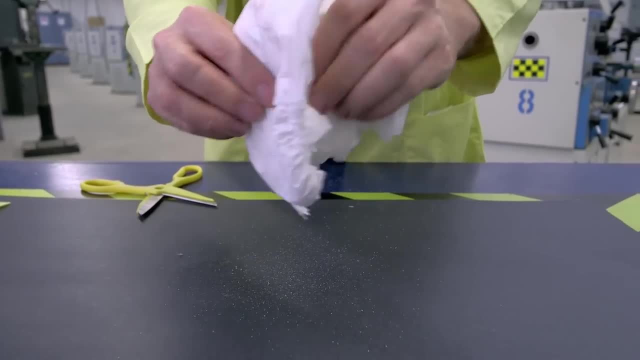 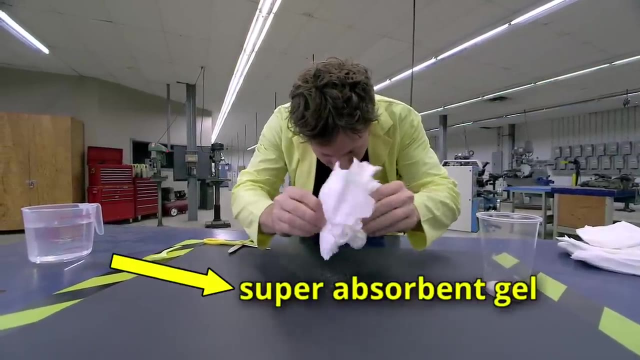 and you shake the diaper over the construction paper, you'll see that there's a little powder that comes out, And this is the secret ingredient. This is super absorbent gel. What it does is it soaks up all the liquid, and diapers are full of them. 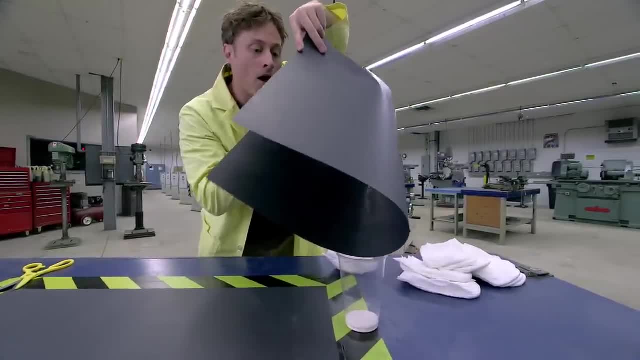 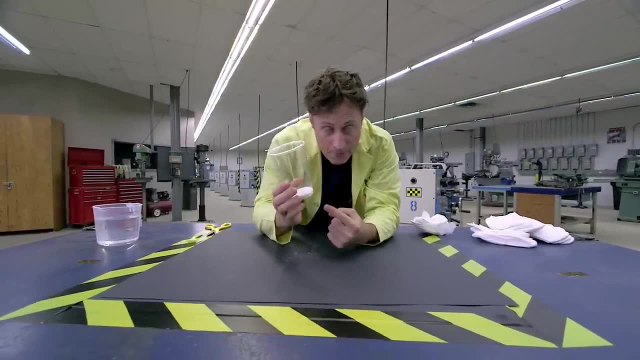 And you carefully pour it into a plastic cup like that. Now you can see I have already done it with a number of diapers. It's important to use a plastic cup because it's a little messy, although it's non-toxic- it's totally safe- but it's still easier to clean up. 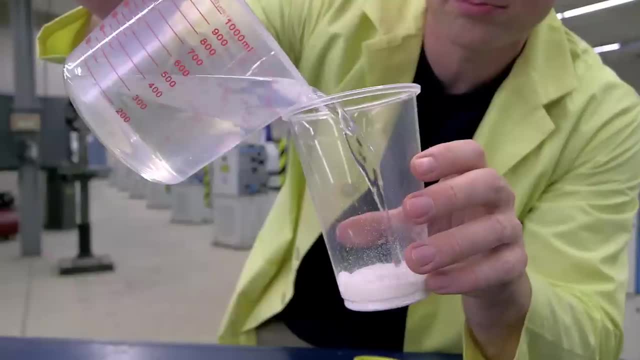 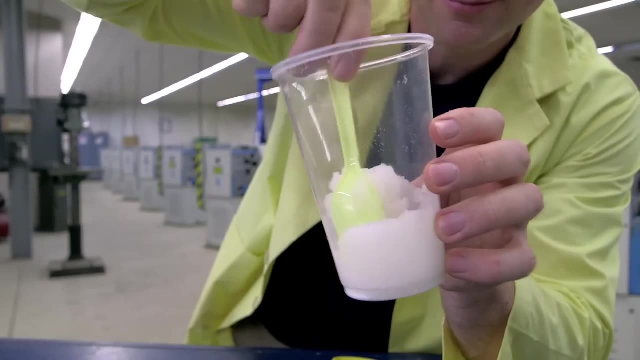 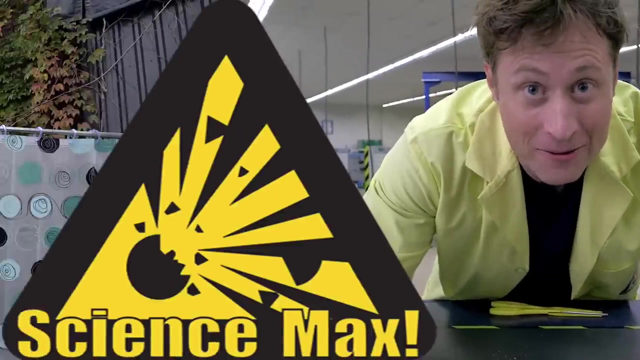 by just throwing the cup away. Now add some water and what happens is this super absorbent gel absorbs the water and turns very quickly into a paste. Look at that. Now let's max it out: Five kilograms of super absorbent gel. 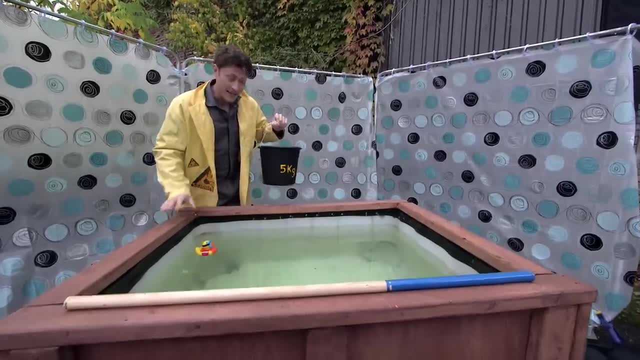 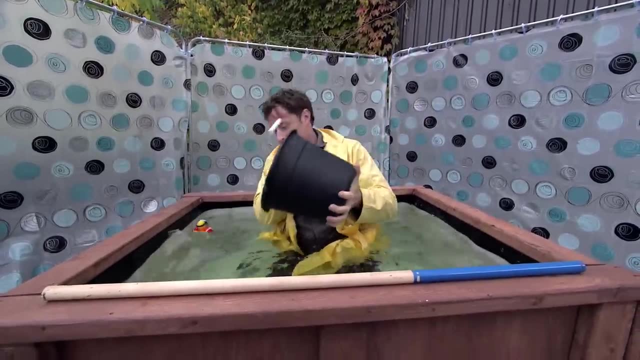 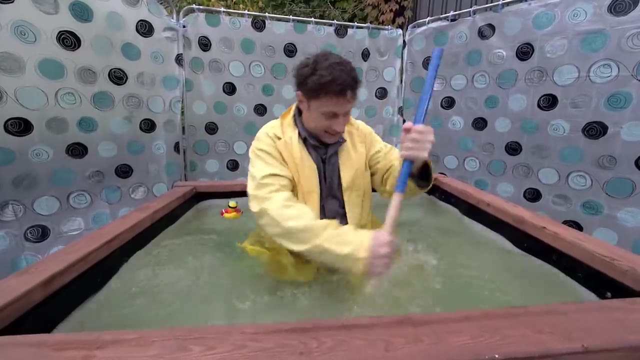 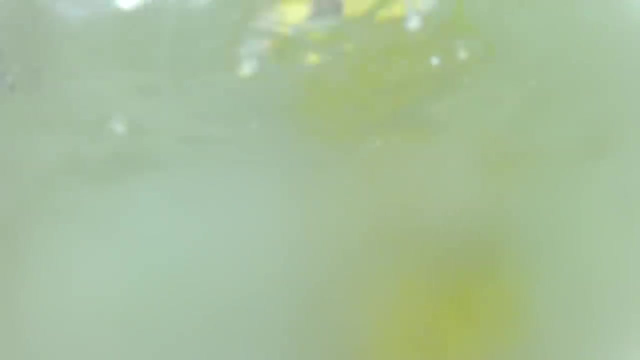 500 liters of water. now it is time to do science, And I have my own snur stick. Yep, definitely coming along. I'm not exactly sure if we're getting anything on this camera, but I want to make sure it's recording. 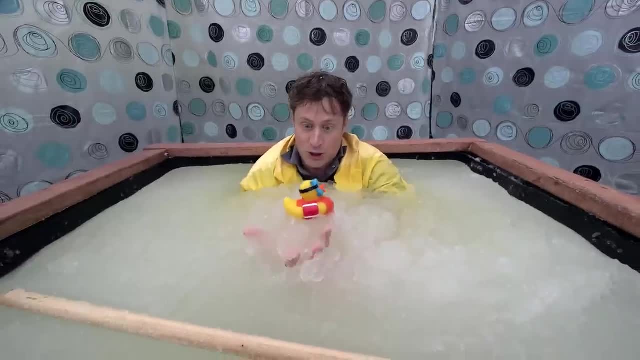 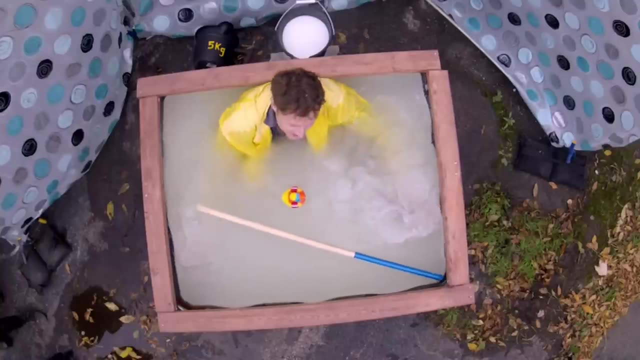 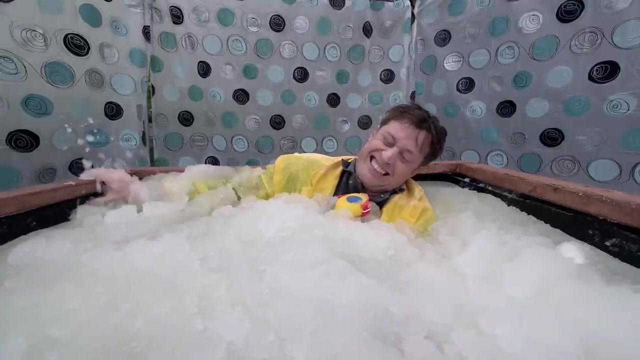 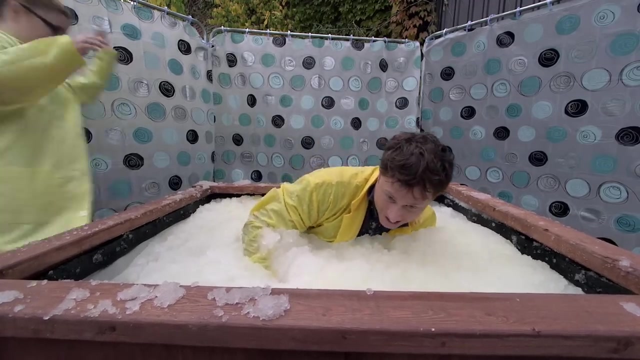 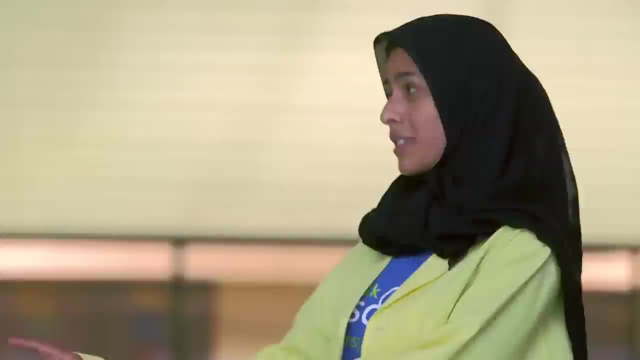 Yep, it's recording. Here we go. It is definitely turning solid. Well, there you go, The giant super absorbent gel experiment. What a really simple experiment, right? Corey Trevor Need some help getting out. How many outfits have I been through in this episode? 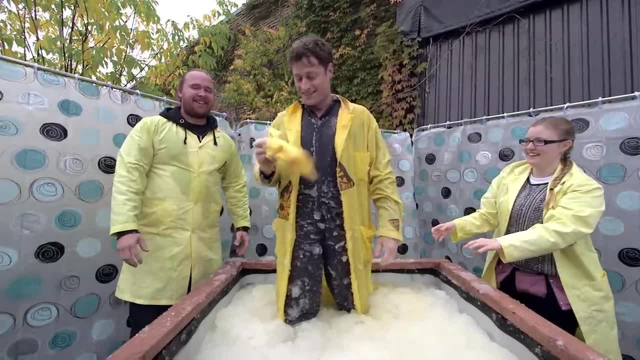 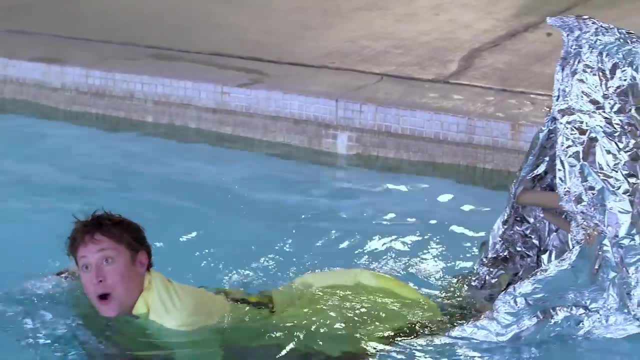 How many outfits have I been through in the episode? Anybody have a towel. There you go. Thanks, buddy, that's great. No, no, no, no. Busnea's idea of adding structure to the tinfoil boat was definitely right. 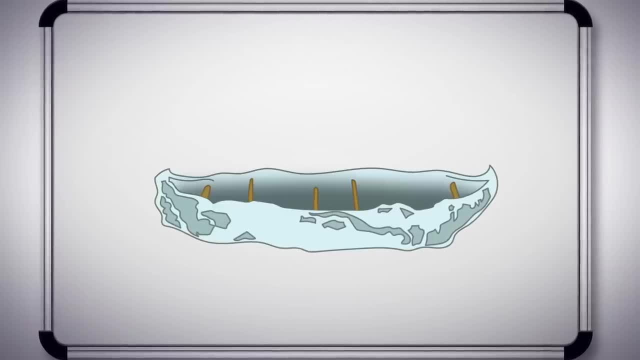 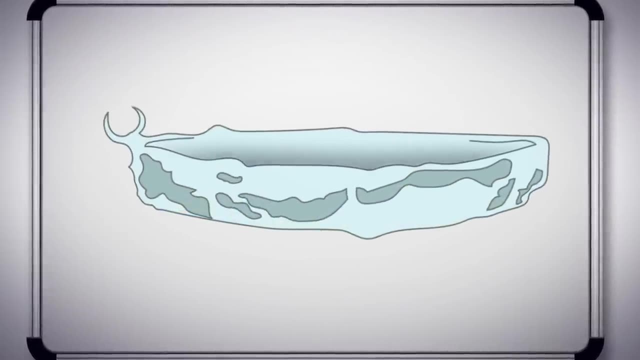 We just needed to go further, so we did it again. This time we made a much larger boat. We started with a sheet of cardboard, then wrapped the tinfoil around and added some metal supports taped to the cardboard across the boat this way to make ribs. 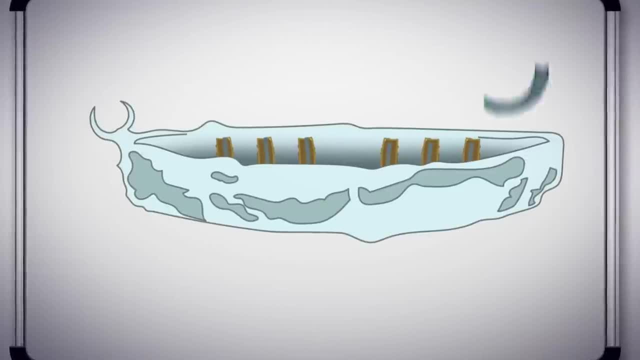 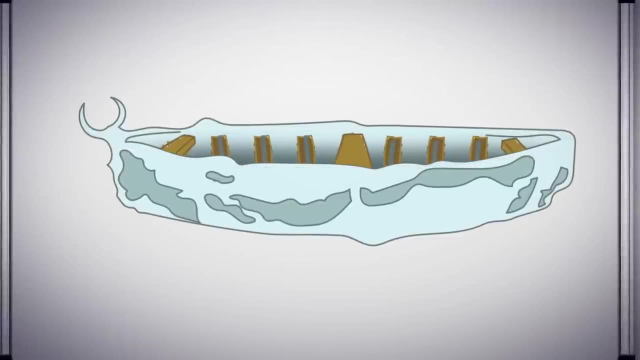 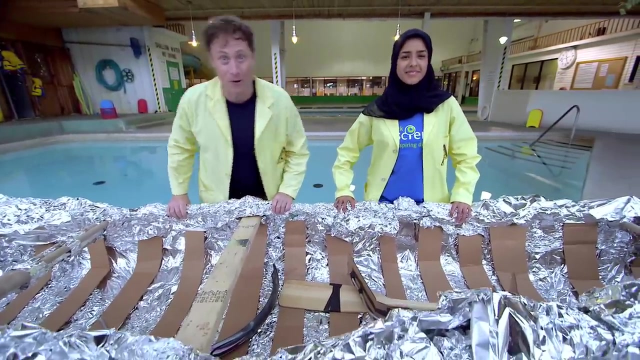 as well as some other supporting pieces in the front and the back, Then another metal rod all the way around the top and finally supports across the middle. All right, feel how strong it is. I'm really excited about this version of the tinfoil boat. 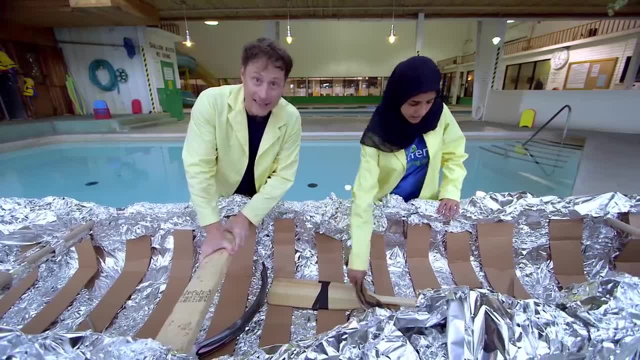 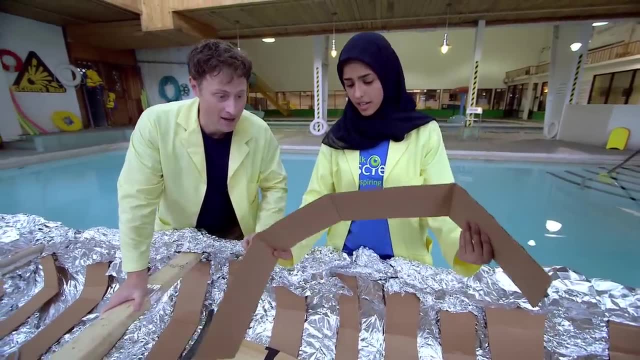 What we did is we used thwarts, big, hard pieces of wood. that we did last time, but this time we have ribs, Ribs right which are made of a cardboard and metal rod attached to it, and And shaped, and we did a whole bunch of them. 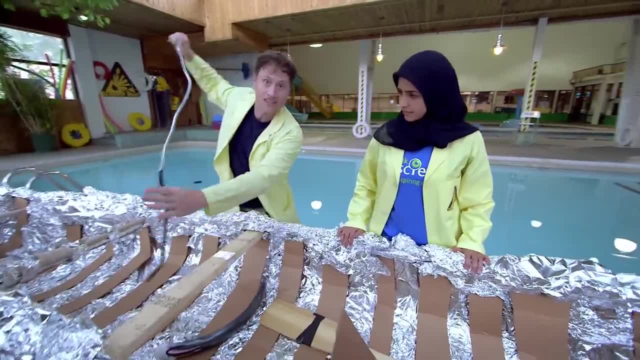 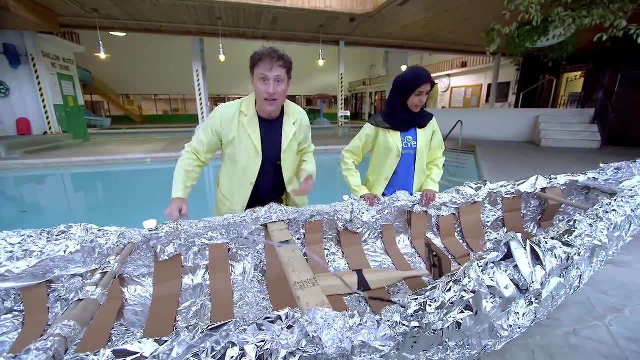 in the whole length of the boat, And then we used all of this bendable metal, which is very large, And we have one that runs all the way around the gunwales and a whole bunch that have run down the inside, And we even used bike fenders at the front. 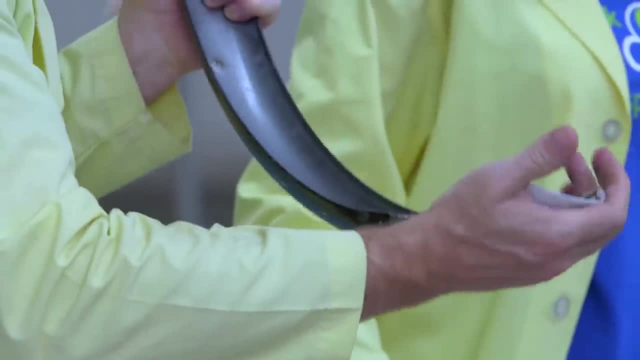 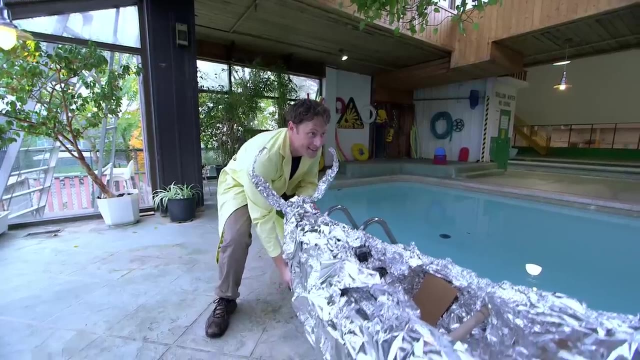 and the back of the boat to give it super rigidity so that it hopefully won't go like all of the other boats have done so far. Are you ready, humans? Let's do this. One, two, three lift. All right, let me get over. 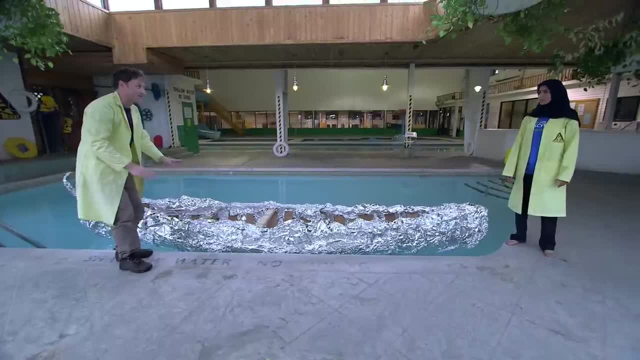 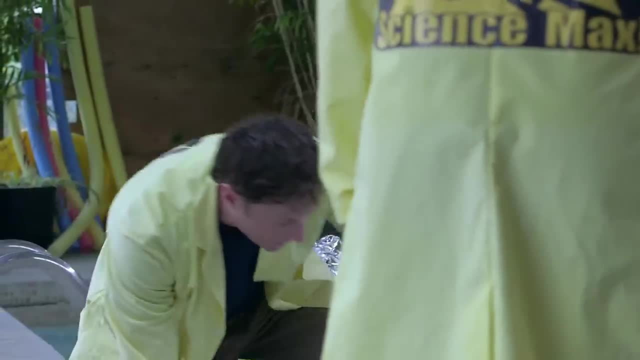 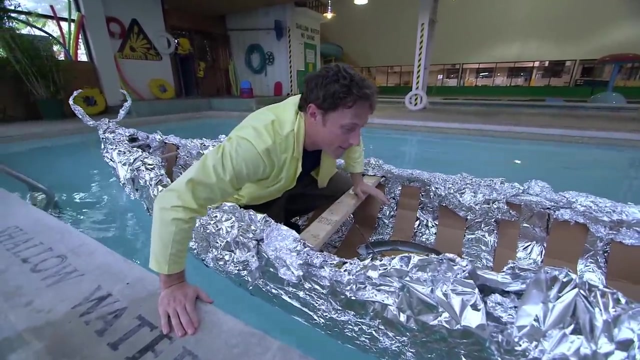 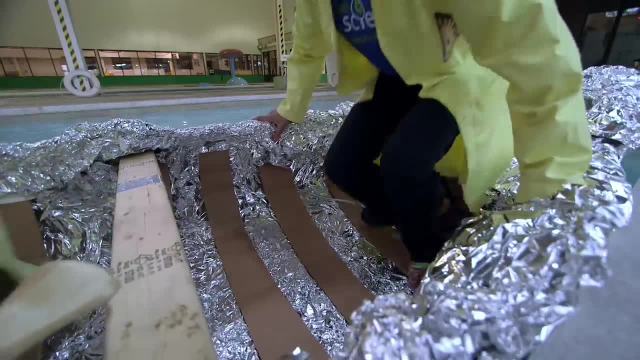 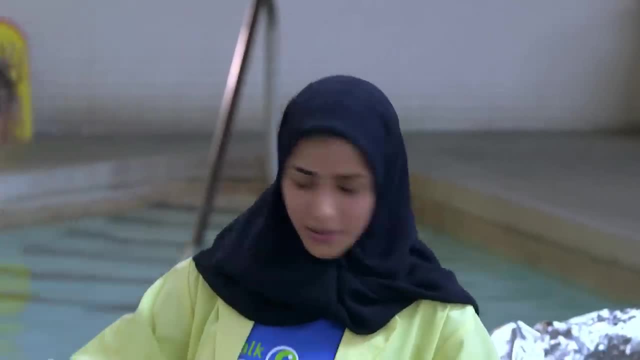 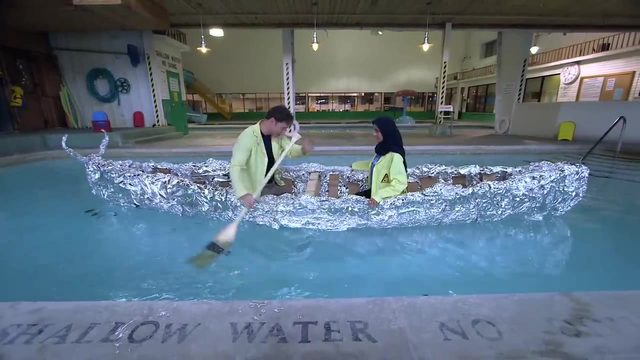 Hey, it works. Whoa All right. Oh, it's working. Ha ha ha ha. Look at that, It works perfectly. The tinfoil boat explodes. The tinfoil boat experiment has been done. Science Max experiments at large. 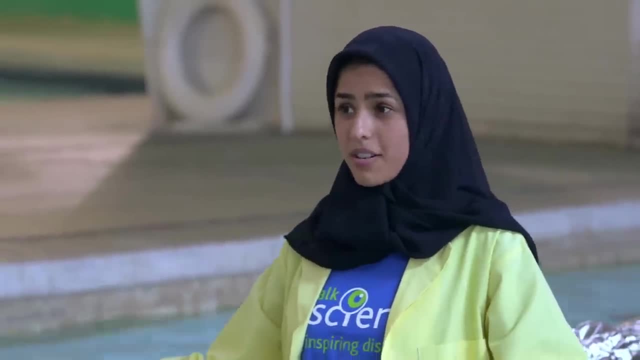 What do you think, Ms Nia? The only reason I got into this boat is because I knew it was going to work Really, Oh yeah, So you knew you would never get wet. See, I don't think that's fair. 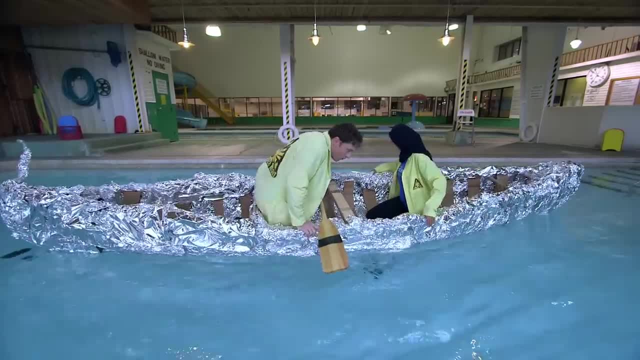 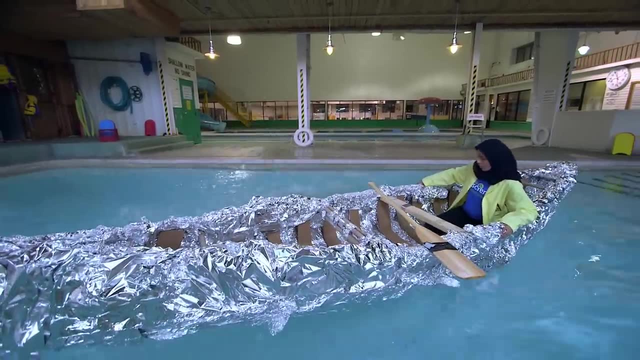 I think it's time that you, that you got wet. What are you doing? I think we should go. I think you and I should just get wet right now. Ha ha, ha, ha ha. Someone help? Whoa. 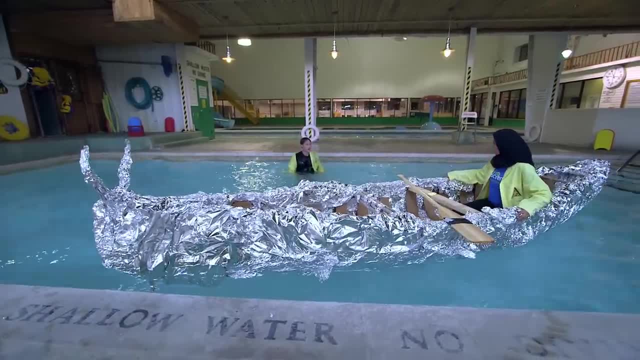 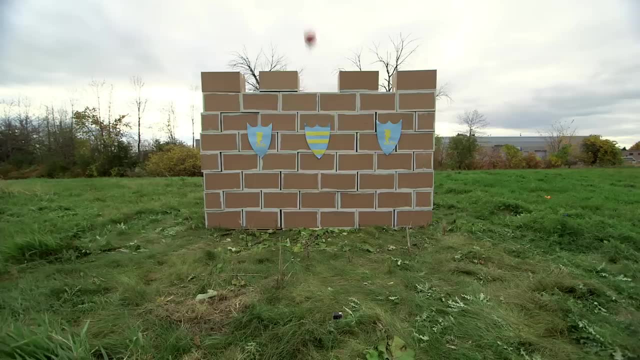 Whoa, You're still dry, aren't you? That is so unfair. Science Max is a show where we take small experiments and do them big. If you want to try these experiments yourself, go to our website for instructions, But not all the experiments on Science Max. 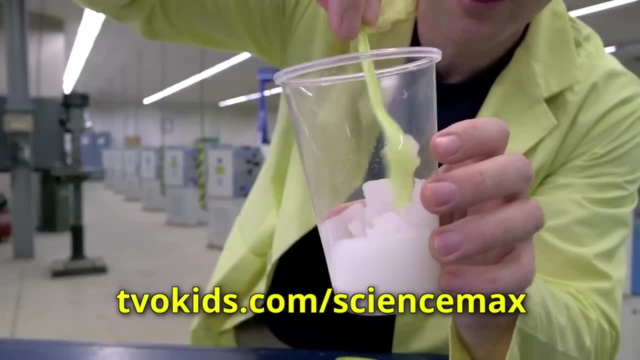 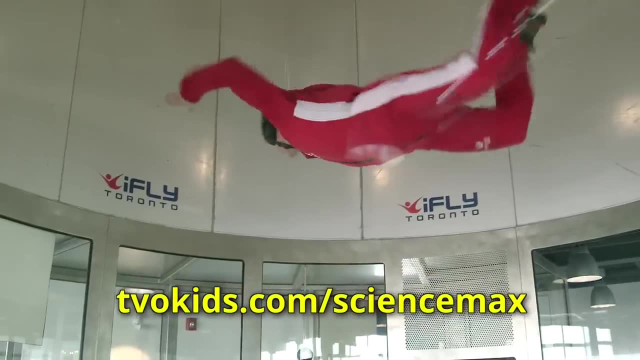 are the kind you should try at home. This one, yes, This, no. Try this, don't try this. A big yes, a big no. I I don't know how you could possibly do this one at home. And remember, if you're ever not sure, ask an adult. 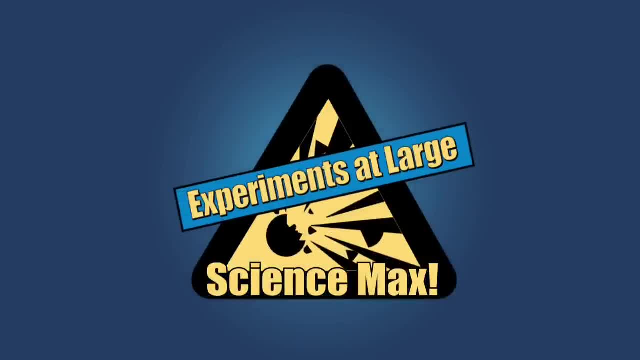 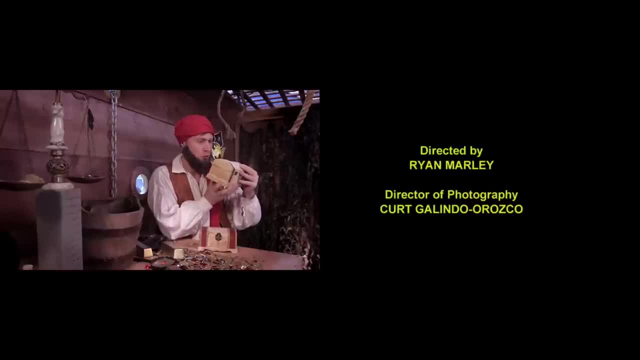 Thanks for watching Science Max Experiments. Science Max Experiments at Large Science. I don't know what you're saying. I don't speak treasure chest. The one thing I'm really trying not to think about is that this is the stuff that's in diapers. 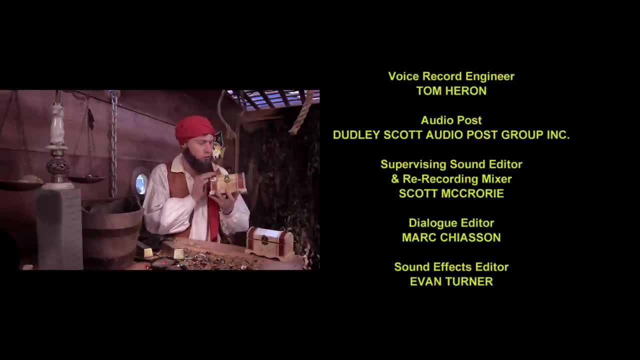 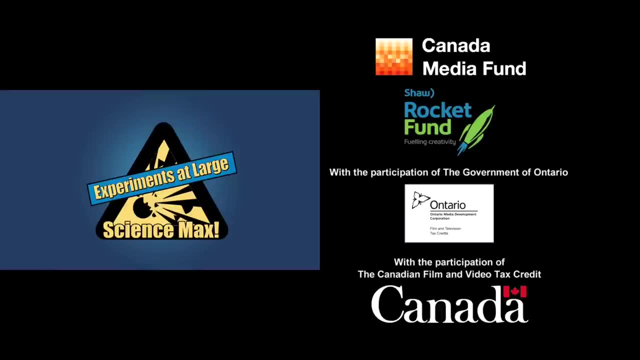 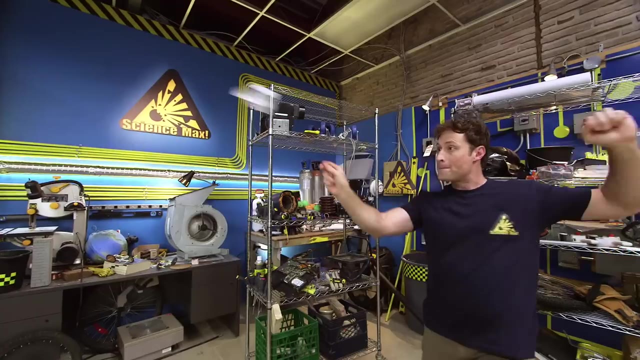 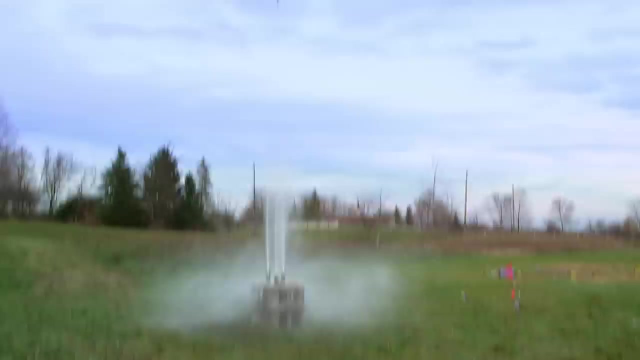 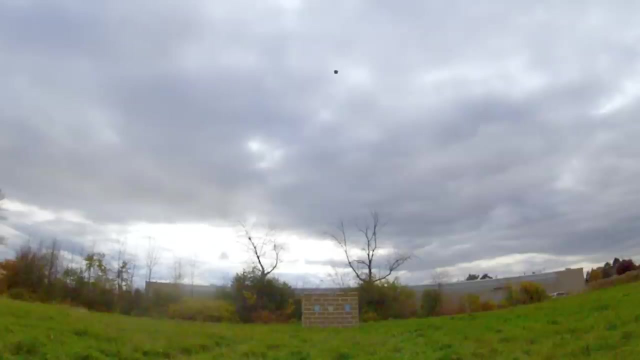 Let me talk to your brother. Whoa, whoa, whoa whoa. Don't talk with your mouth full. Have you ever done a science experiment and wondered what it'd be like if you did it big? I have, Yeah. 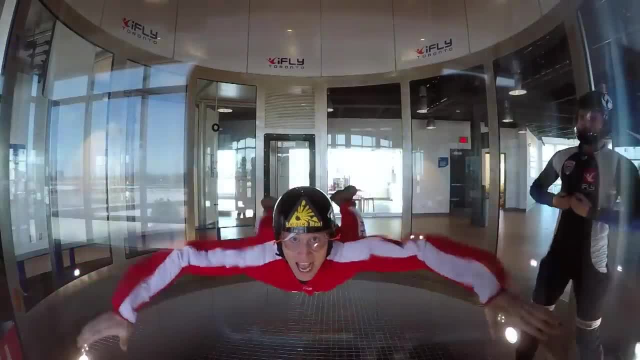 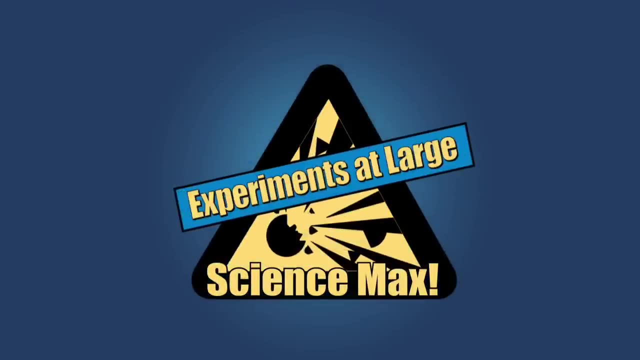 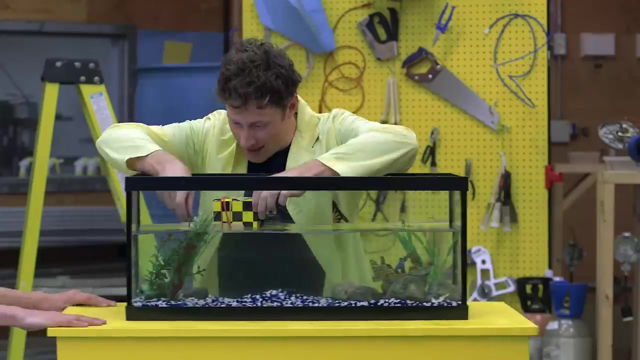 My name is Phil and I take your everyday science experiments and do them big. This is Science Max Experiments- Experiments at Large, Science Max. This episode of Science Max is all about elastic energy. We use it to build a catapult and a paddle wheel boat. 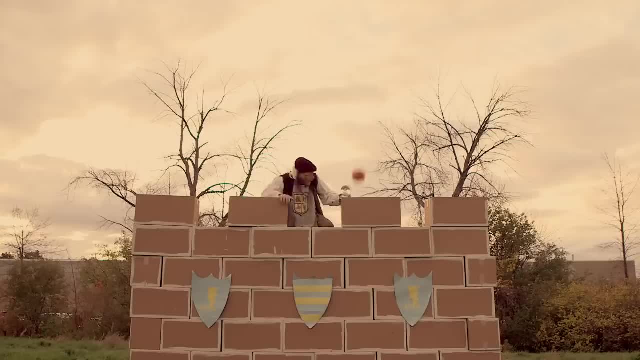 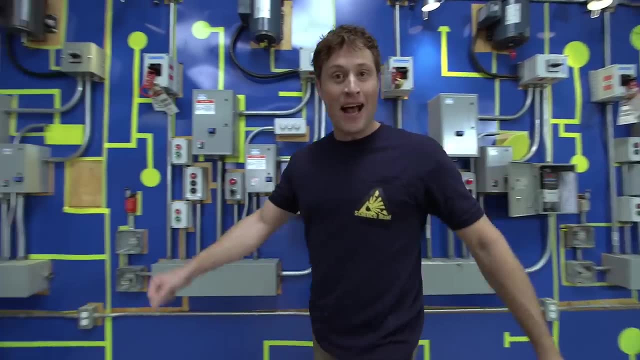 and then we max them out. We even learned some history. Elastic energy Today. on Science Max Experiments at Large. Welcome to Science Max Experiments at Large. I'm Phil McCordick and today we're going to be building one of the most devastating 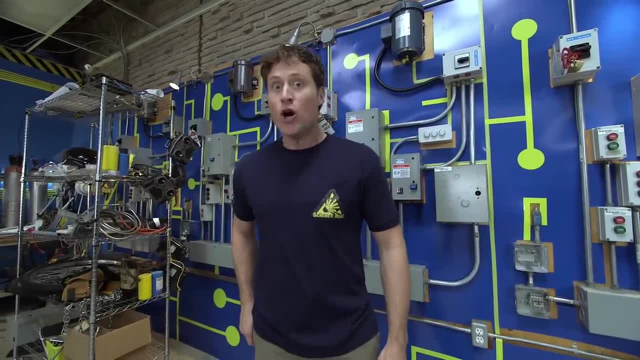 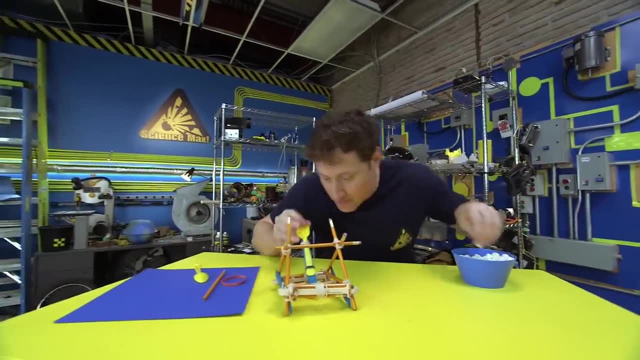 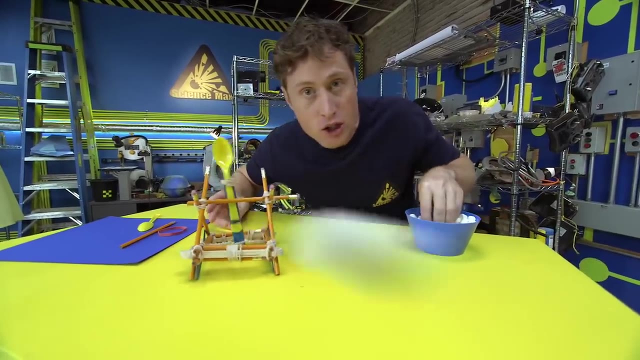 one of the most powerful machines known to medieval man, using a plastic spoon, among other things. We're going to be building a catapult. Catapults were used throughout history for all kinds of reasons to throw all kinds of things, but mostly big stone blocks at castle walls. 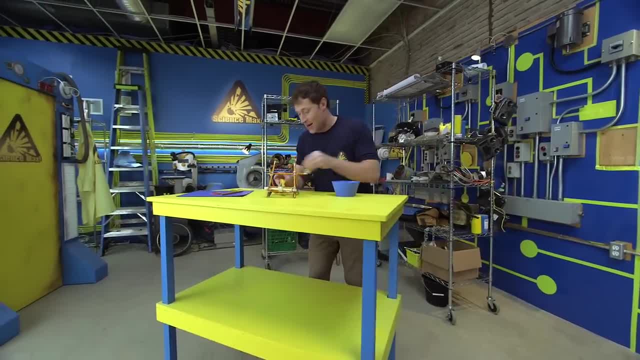 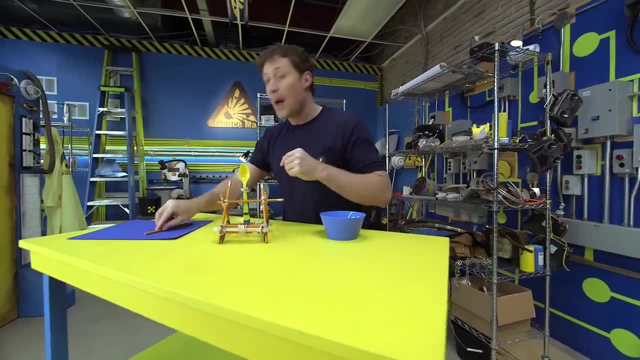 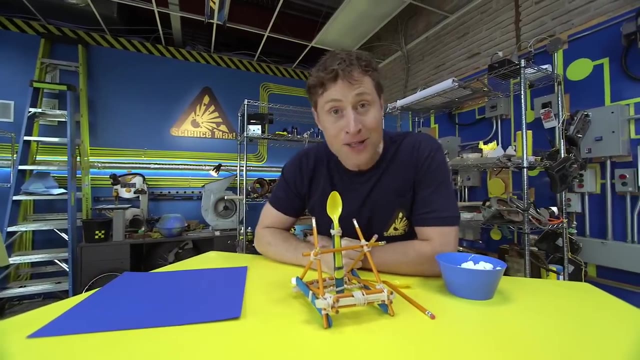 in order to knock them down. Here's what you need in order to build your own catapult: You need elastics- uh, pencils- un-sharpened is fine- plastic spoons, like I said, and popsicle sticks- Popsicle, popsicle sticks. 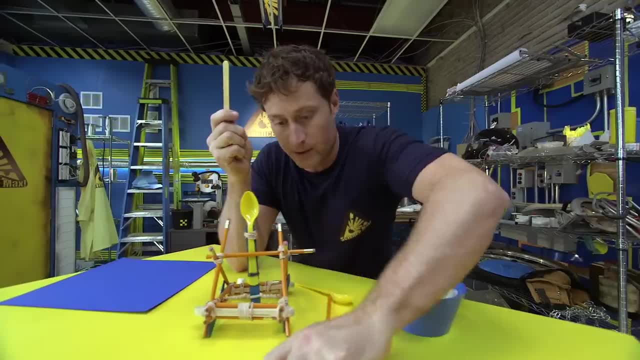 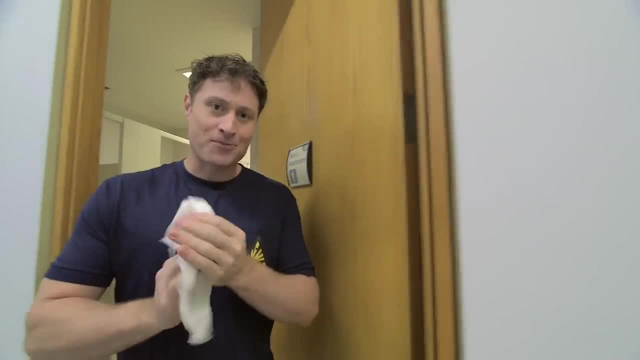 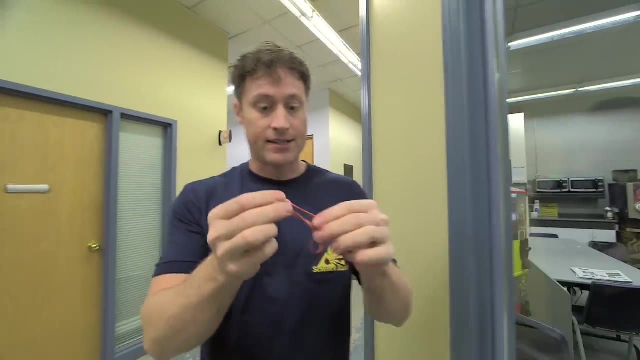 Popsicle sticks. Um, I'm going to go wash my hand. So here's the science behind what we're doing today. It's all about elastic force. Elasticity is a property of solid materials like this, elastic, and how much they tend to return to their original shape. 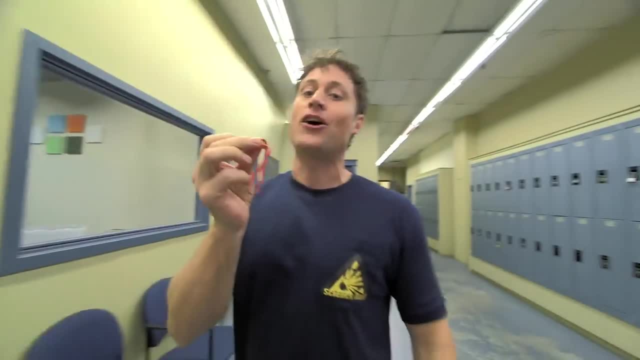 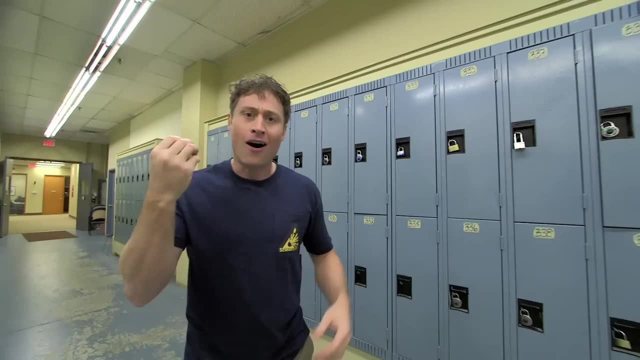 when deformed, like when I pull on it, Elastics are called elastics because they're great at doing just that: You can pull on it, and pull on it, and pull on it and it'll- ow, ow, ow- always return to its original shape. 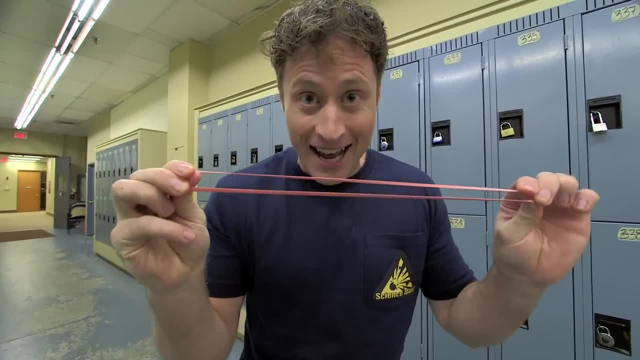 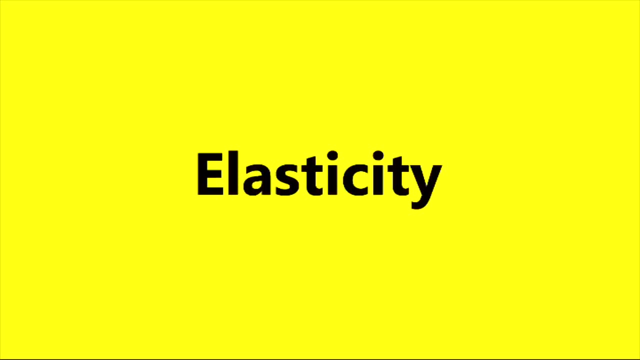 So we are using the power of elastic force today. Ow. Now it's time for a Science Max quiz. Elasticity is the ability for a material to return to its original shape when deformed like this or this. Which of these materials have elasticity? 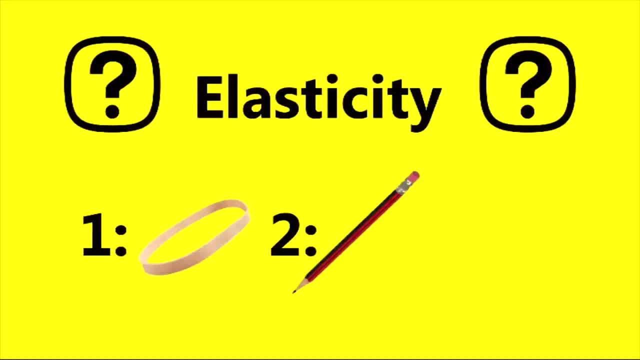 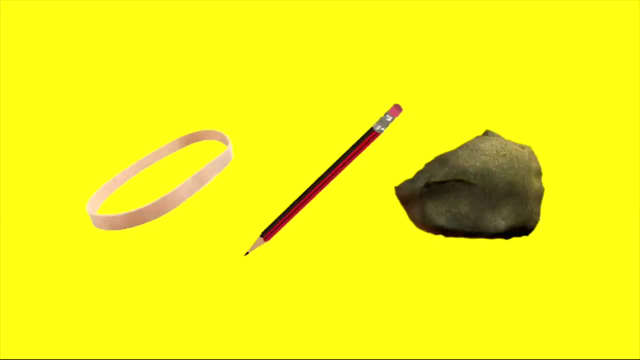 A rubber band, a pencil or a rock? Ha-ha, this is a trick question. The answer is: all three. Most solid materials have elasticity. Nearly everything will deform a little and still be able to return to its original shape. It all depends on how much. 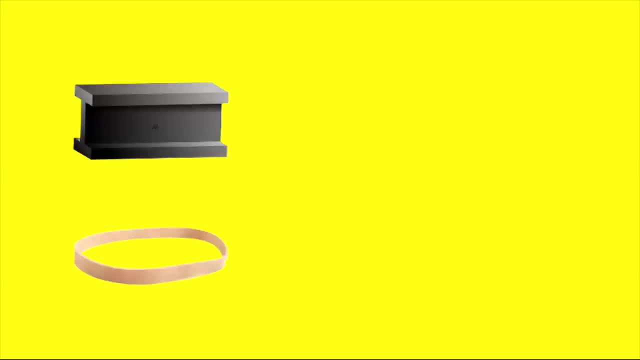 This is a steel bar, This is an elastic band And this is an ice cream sundae. We're not talking about ice cream sundaes now, though, so get that out of here. Good, Now: a steel bar and an elastic band. 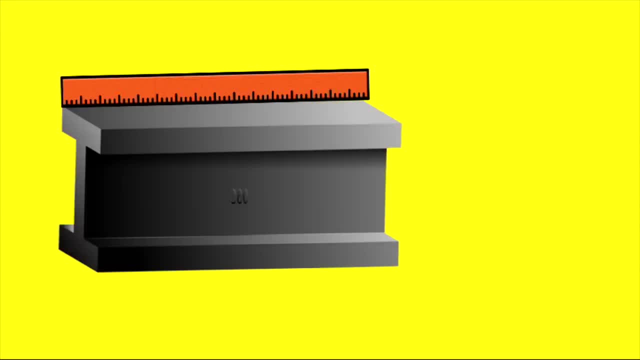 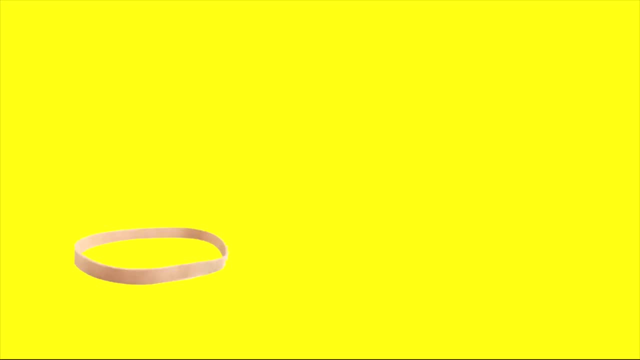 both have elasticity. A steel bar can be stretched to 1% of its length and still spring back. A rubber band can be stretched 300% or more. The difference between the two is why we make balls out of rubber and buildings out of steel. 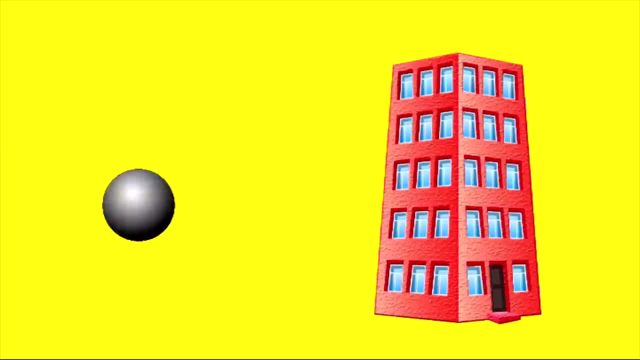 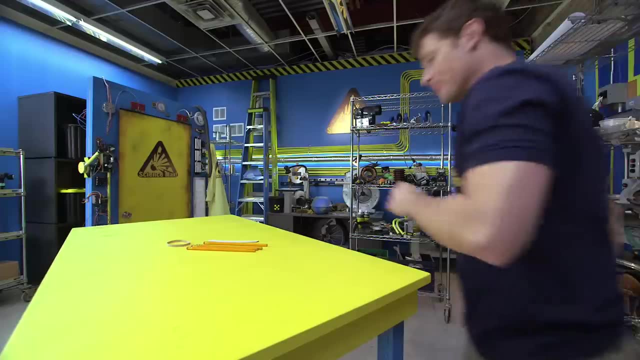 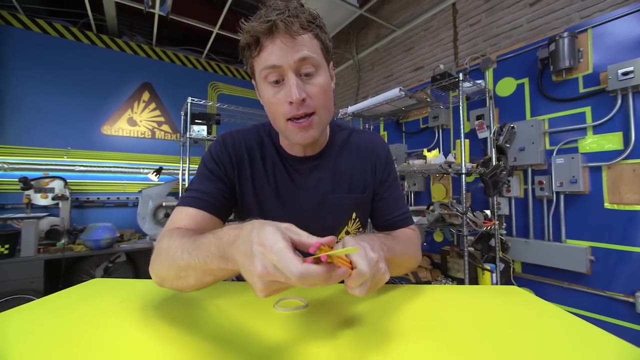 Because the other way around wouldn't be good for balls or buildings. This has been a Science Max quiz. All right, let's build our catapult. The first step: take four pencils and stick your popsicle stick in between, so you have two on the top and two on the bottom. 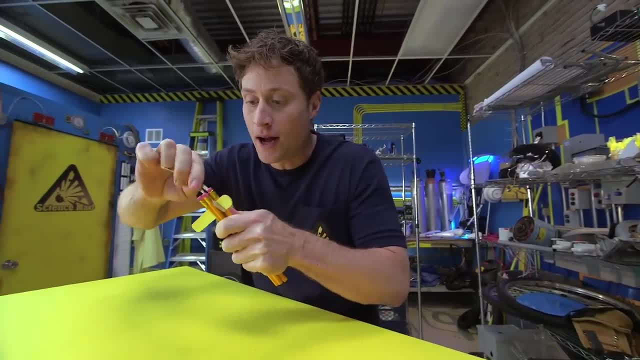 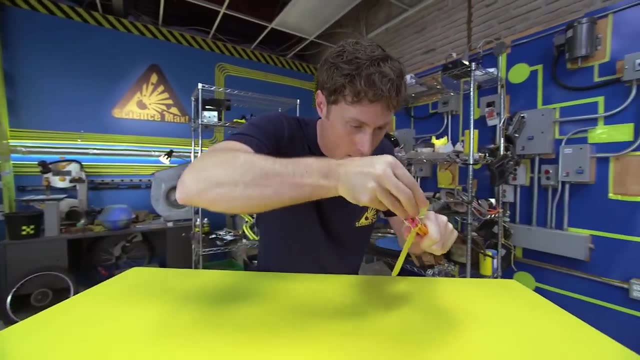 And then use your elastic to go around and around. That's why I like building things with elastics: because it makes it very fast to tie things together, because once you go around and you have it nice and tight, you just pop it over the end. 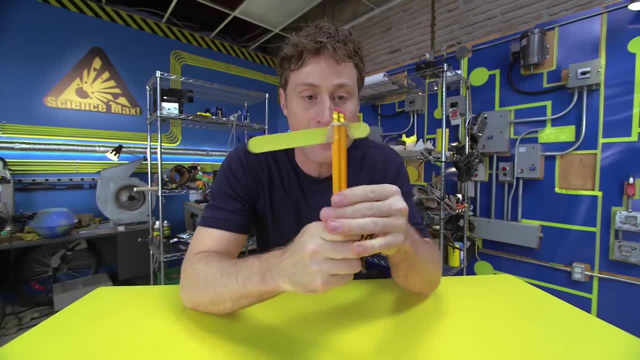 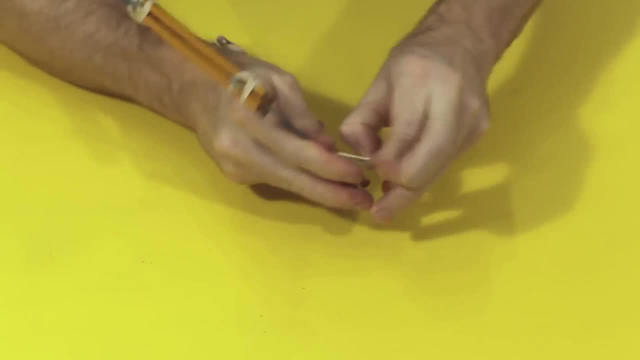 and voila, it stays together, And that is how you start making your frame. Put more pencils on that side and another popsicle stick on the other end, held on at the corners with more elastics. Then take even more elastics and put them right around the middle. 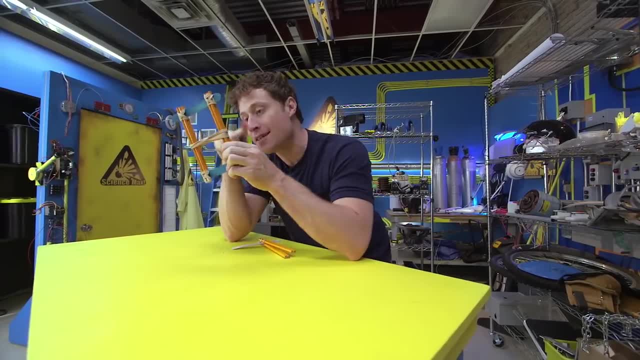 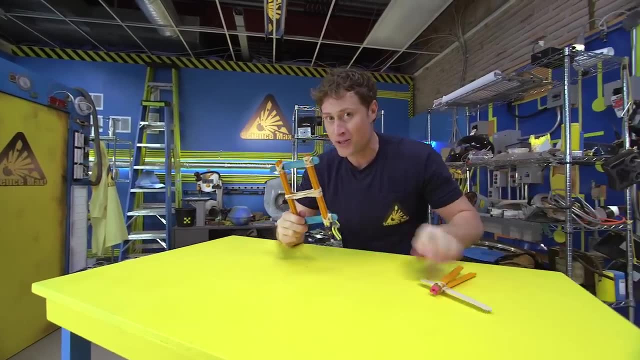 until you get this, I've added a few more elastics around the middle here, and that is where we're going to get all of our elastic force. I think I have six. The more you use, the better it's going to work. 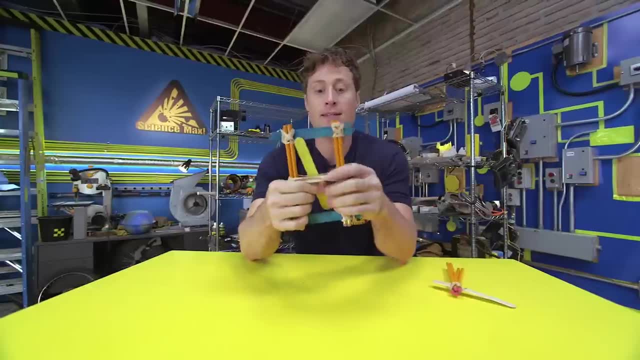 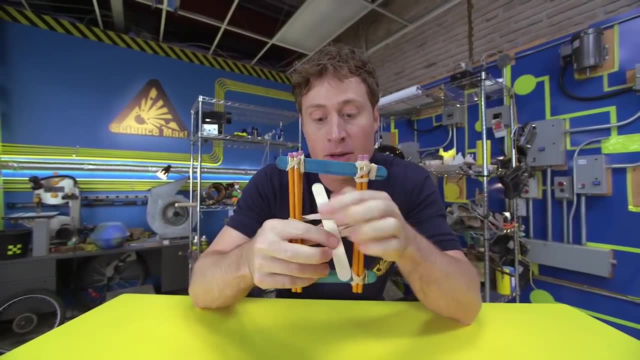 Take your popsicle stick, stick it in between the elastics and then start spinning it around. Here's the reason I use pencils and popsicle sticks is because the pencils are a little bit longer, which allows you to twist the popsicle stick. 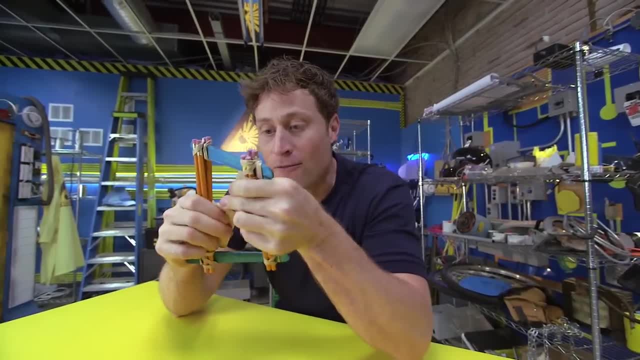 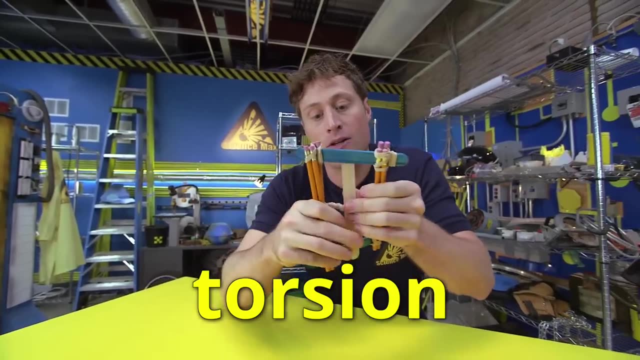 around in the middle and build up the elastic force. Now, because I'm twisting, the elastic force we're using here is called torsion or twisting force. When you feel you have enough torsion, pull your popsicle, stick down a little bit. 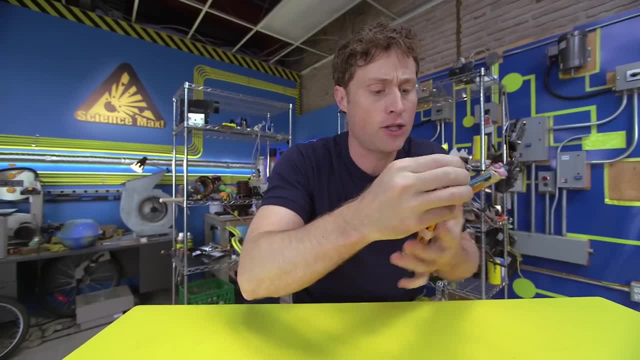 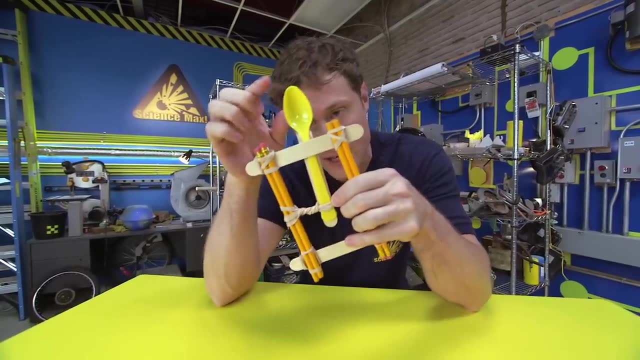 so it won't unwind on you and you'll see that you have all kinds of elastic energy. Then take your spoon and stick it on the popsicle stick, and you can also break off the popsicle stick if you want to make sure it's the right length. 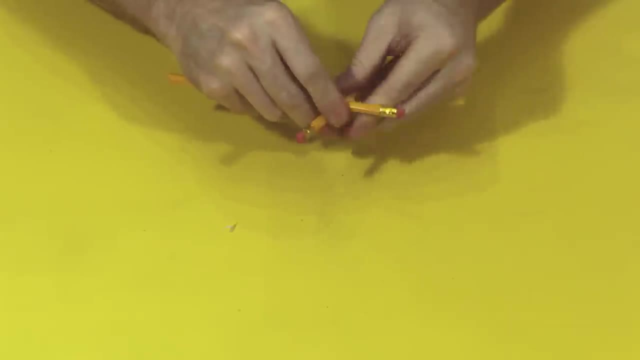 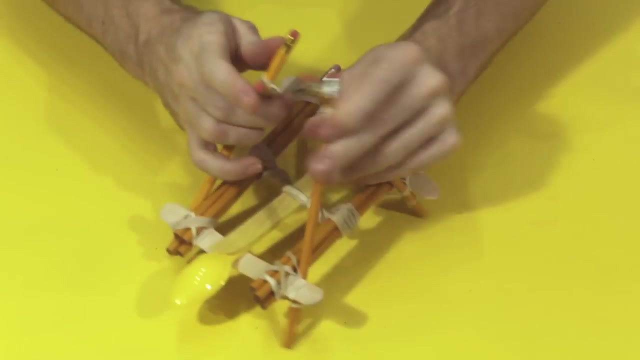 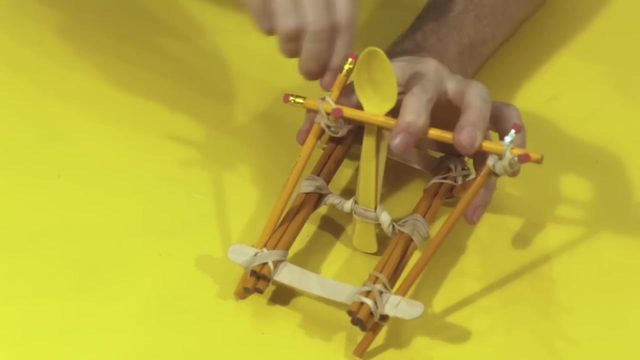 And it works like that. To make the frame, you just need more pencils and elastics. The trick is to make a triangle with two pencils attached to your frame. They should stick up right where your catapult arm would be fully upright. Then take a final pencil and put it across the top. 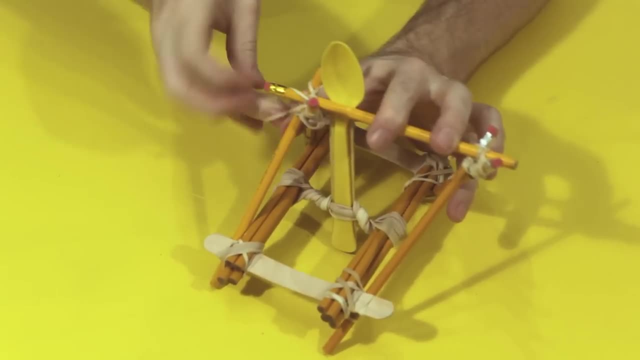 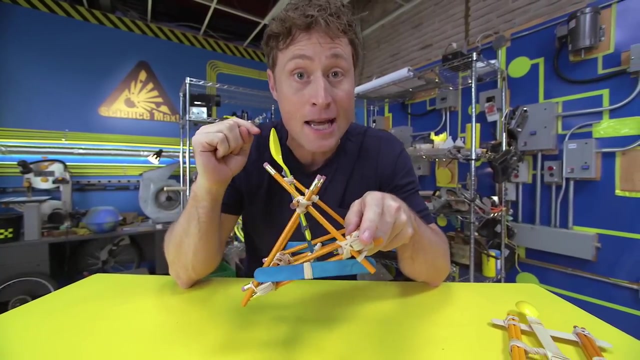 Don't forget to pull the arm back before you put the pencil across, otherwise it'll end up on the wrong side. Now this is very complicated and I went pretty fast, so if you want the step-by-step instructions on exactly how to build this, 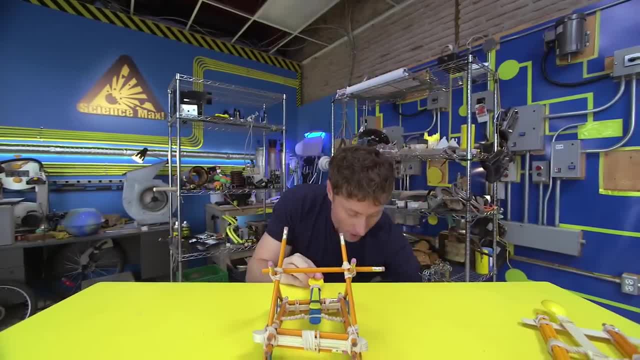 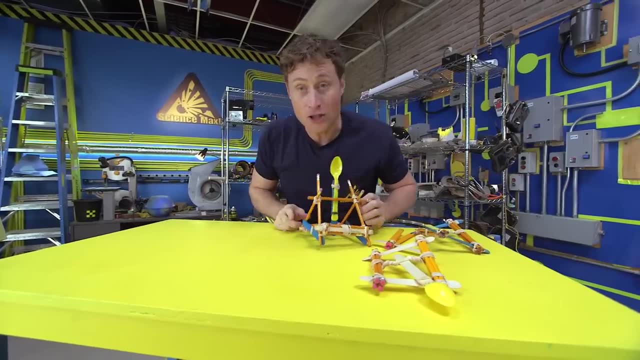 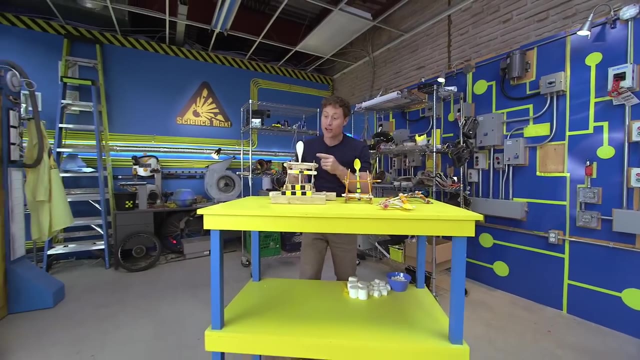 go to our website And there you go- a catapult of your very own that you can use to knock down very small castle walls. I've also built a larger catapult using all of the same principles. Pretty good, huh, It's got a longer arm. 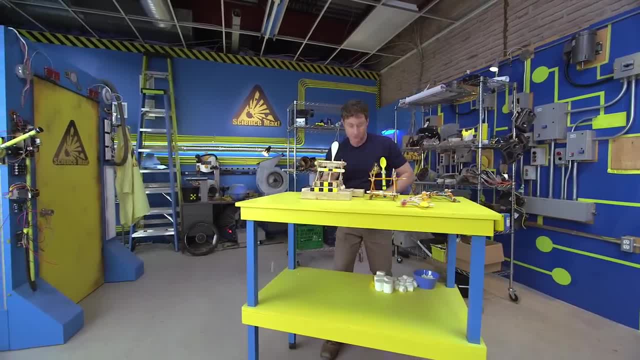 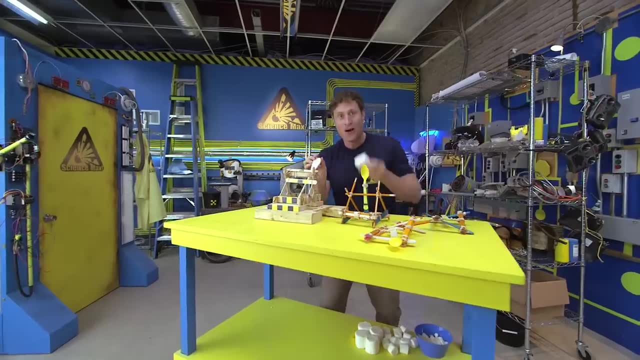 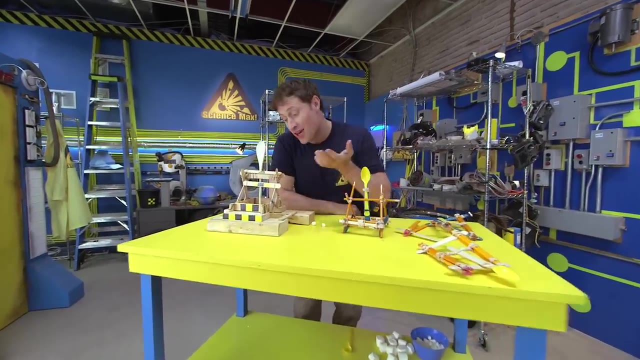 which means I can throw marshmallows even further. Whoa, Or I can throw larger marshmallows, or I can throw very large marshmallows. Now I know what you're thinking. You're thinking: well, is that the largest catapult you're gonna make? 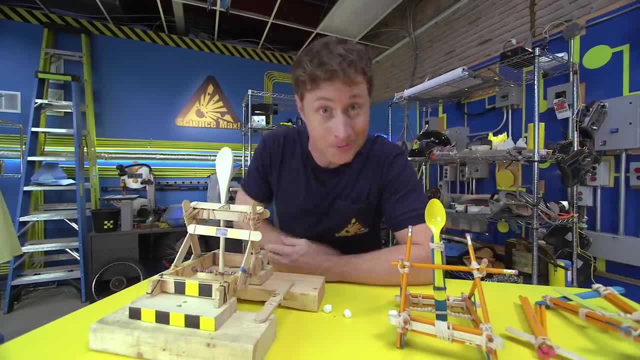 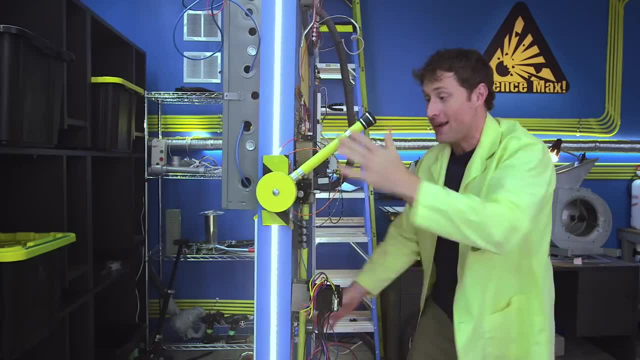 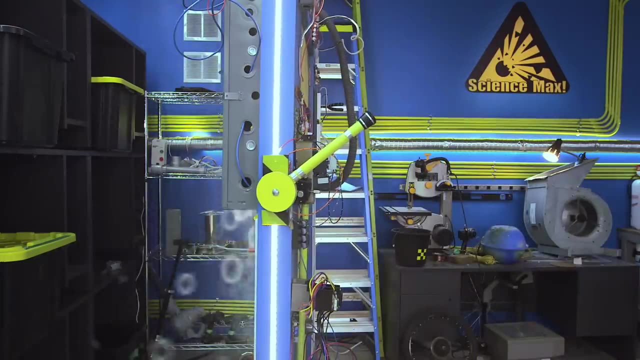 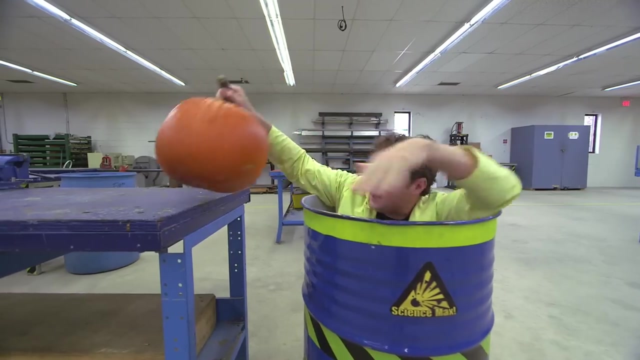 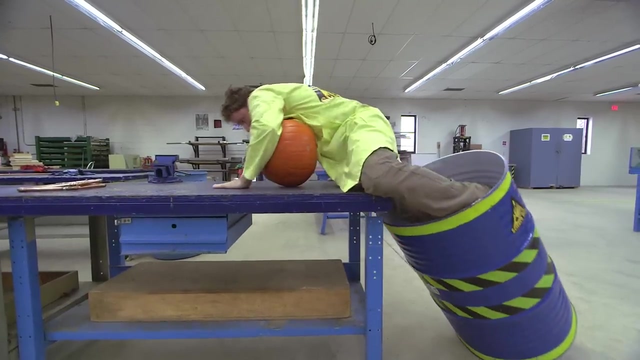 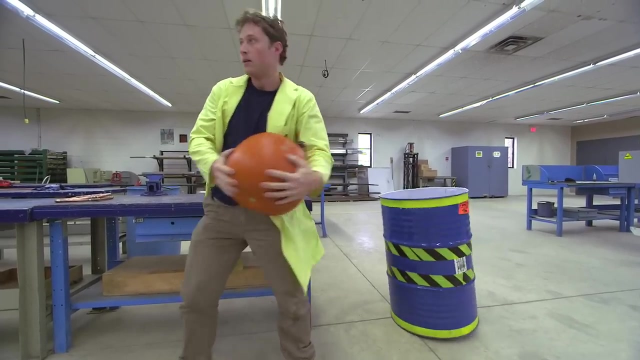 Well, of course not. This is Science. Max experiments at large. I'm headed to the Center for Skills Development and Training and we're gonna max out the catapult so that it's big enough to throw one of these. Hey, Zach. 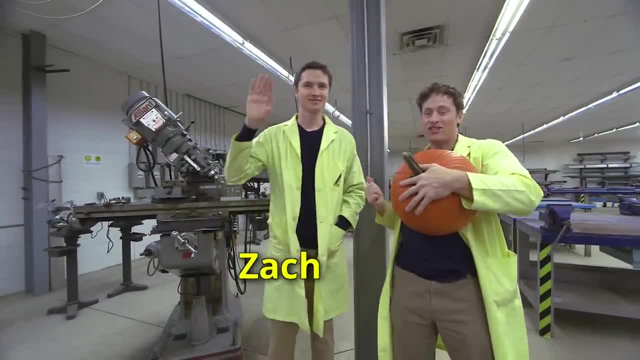 Hey Phil, How you doing? All right, This is Zach. He's a mechanical engineer. You build machines for a living, right. That's right Great, because I need help building a catapult. Okay, but what's with the pumpkin? 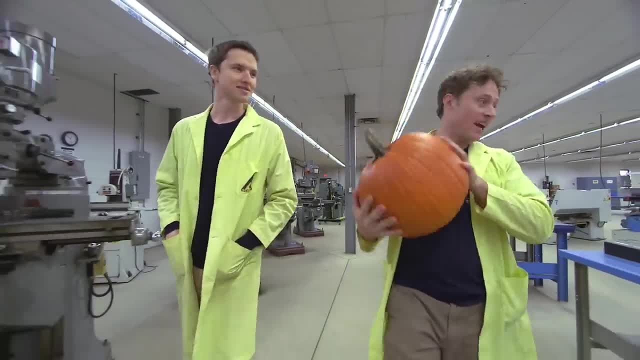 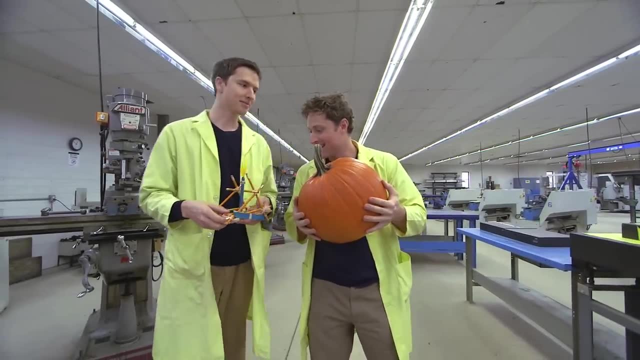 The pumpkin is what I want to throw out of the catapult. See, I figure we just take the small design and we just make it so that we can throw one of these. What do you think You're gonna need a really big catapult. 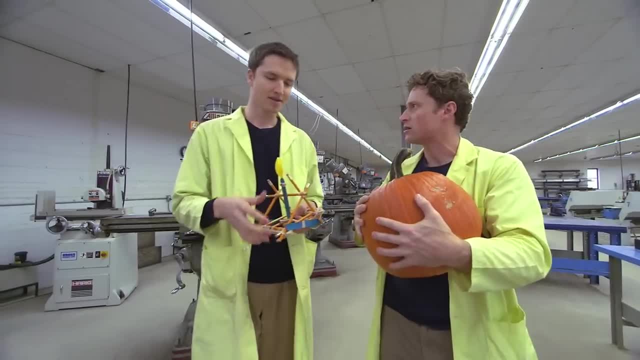 Yeah, and I'm also gonna need some really big elastics. Where do you get those? Well, in medieval times, they used rope to make large catapults. Oh, okay. Well, rope is a lot easier to get and that would be fine. 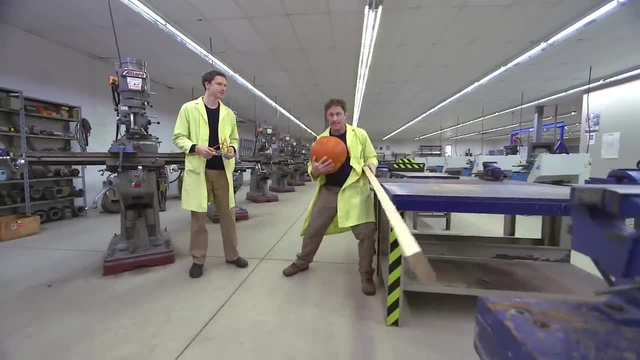 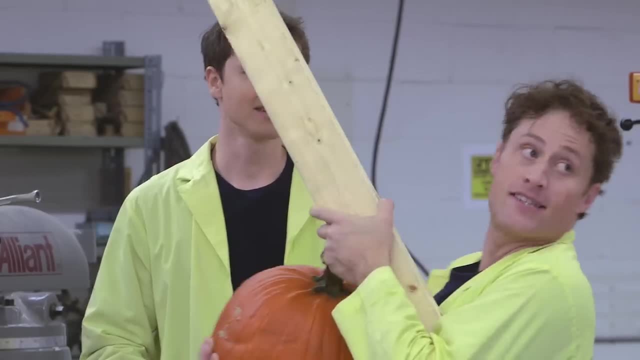 And I want to make this arm as long as this piece of wood here. This is gonna be a huge catapult. It's a huge catapult. I guess we should build it outside, though. huh, Let's do it. Okay, it's over that way. 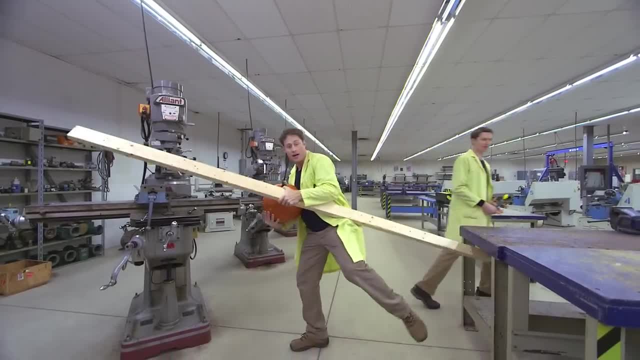 Okay, I'll follow you. Are you okay with that? No, no, I'm fine, You go ahead and I'll just. Maybe, if you hold the door open for me, I could Just hold. No, it's. 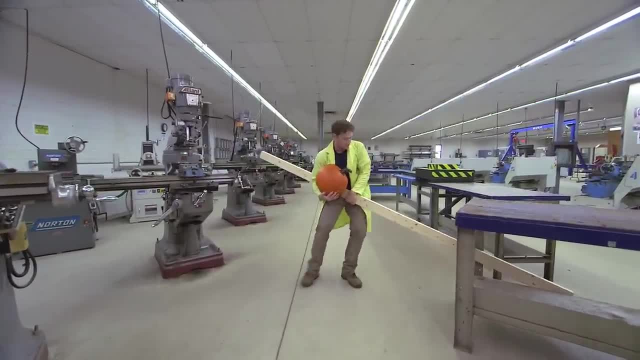 You know what You go and I'll meet you. Make sure you're good. Our full-sized catapult is going to look a lot like the popsicle stick version. We start with a four-sided frame and add some legs on the bottom. 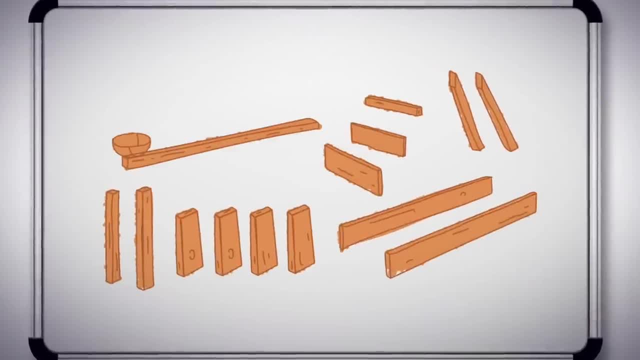 Our spoon is going to be replaced by a long throwing arm with a basket on the end, Then we need a really strong cross brace at the top so that we can put the catapult on the top of the catapult. Now we're gonna need a really strong cross brace. 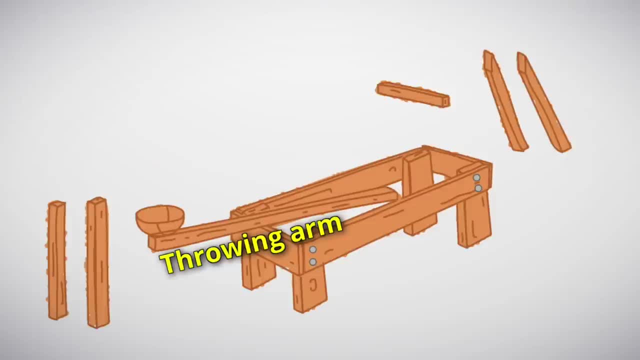 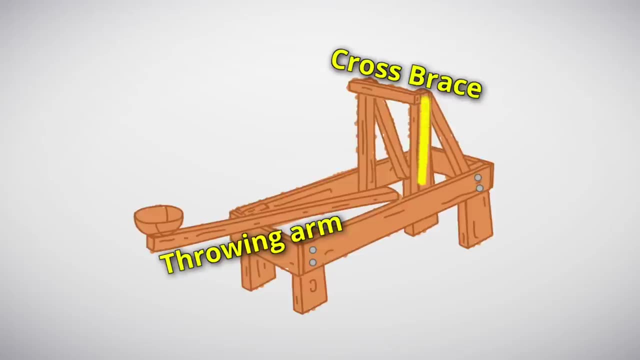 at the top so that we can put the catapult up to stop the arm, Just like in the small version. using a triangle shape is the best, because triangles are very strong. Finally, we need something to wind around and around which is going to give us. 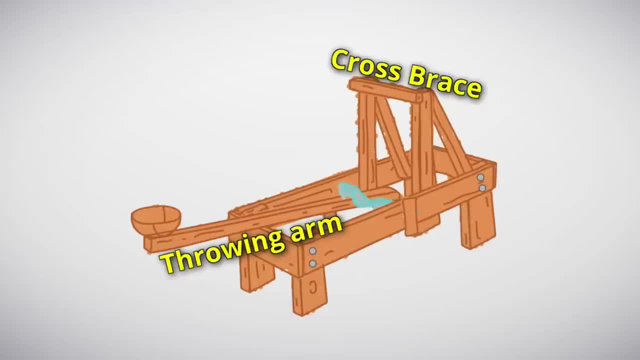 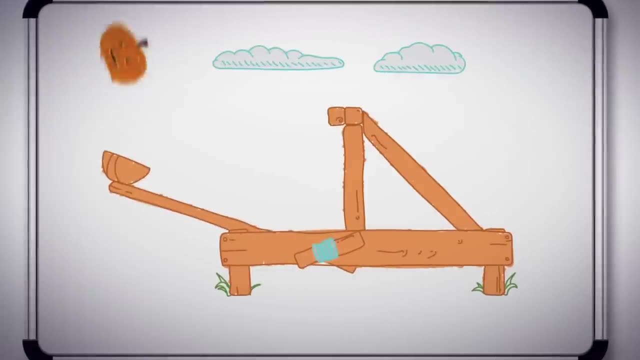 our elastic force. Instead of elastics, we're gonna be using rope for our catapult, because rope has just the right amount of elasticity, But, unlike medieval times, we're gonna be catapulting pumpkins. Once Zach and I got it all put together, 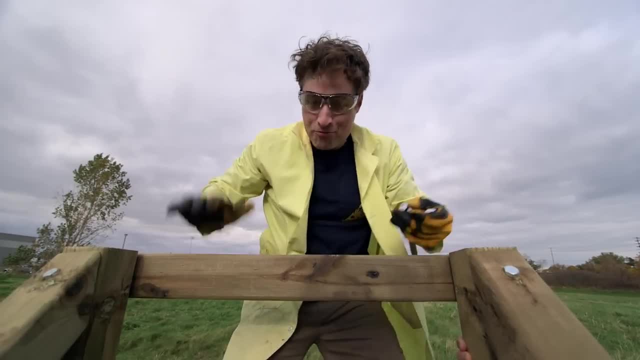 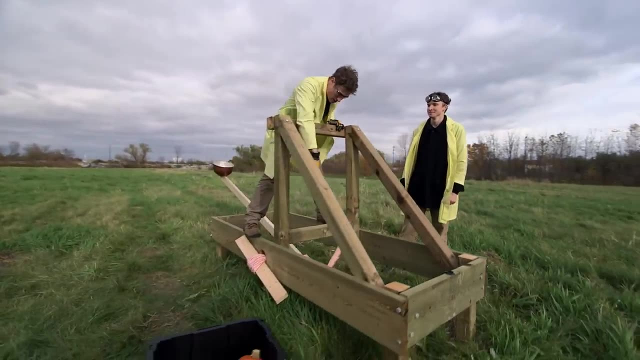 it looked like this: Okay, We have built a catapult. Check it out. It's pretty solid and I think it's pretty amazing. And, just like in the small catapult, we have our elastic force, but this time we're using rope. 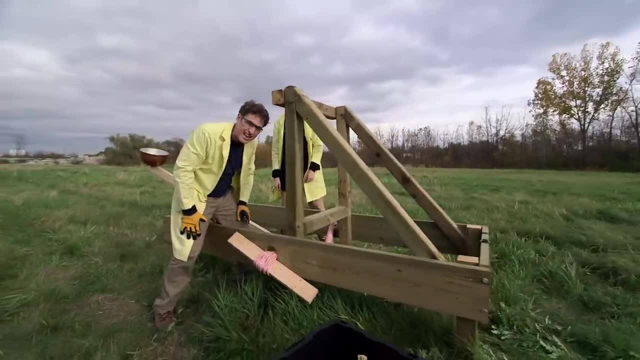 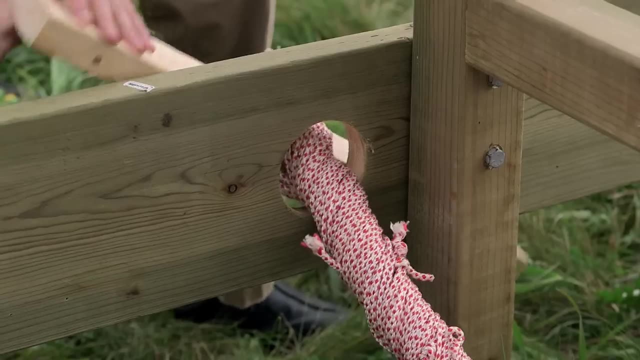 Right, Zach. Yes, Okay, and rope will work as well as the elastic did in the small one. Yeah, All right, great. So what do we do? It's really loose. now We need to wind this up so that we put some tension into it. 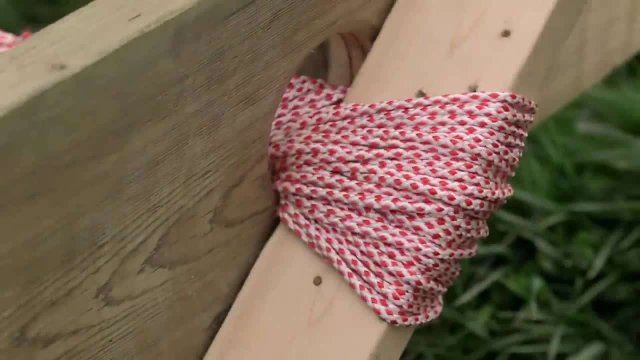 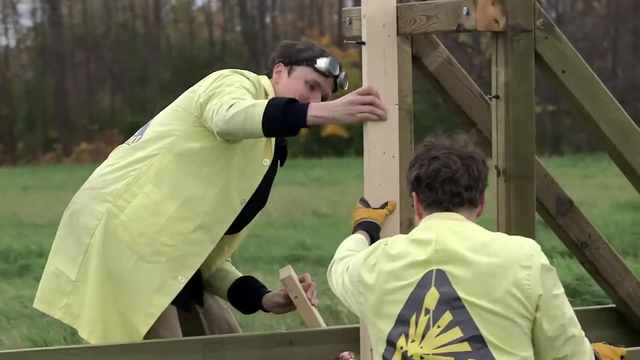 Go. The reason a catapult works is because the rope is twisted. The elasticity in the rope wants to unwind, which gives the catapult its power. Just like the small catapult, the more you wind it, the better it works. Good, Usually in medieval days. 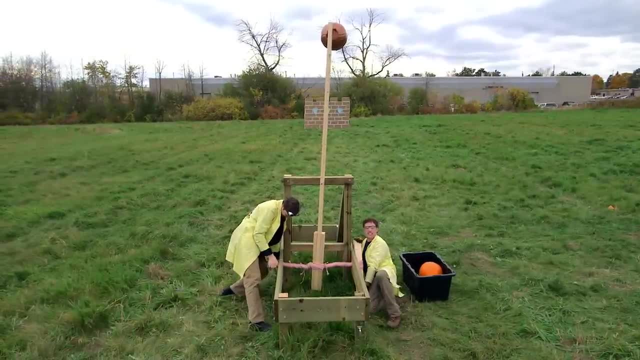 they had whole teams of people doing this job, but it's just me and Zach. now, How are you doing, Zach? All right, Okay, And then we clamp it on here so the thing doesn't unwind, right, Yeah, Good. 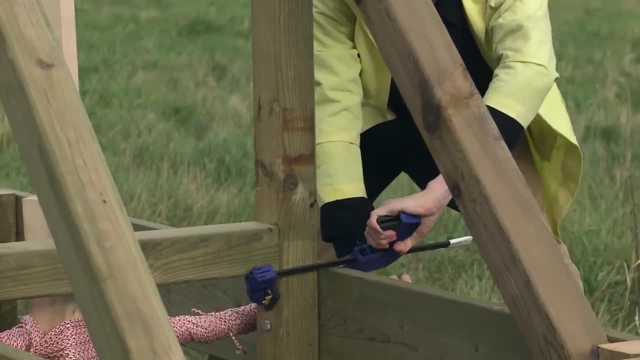 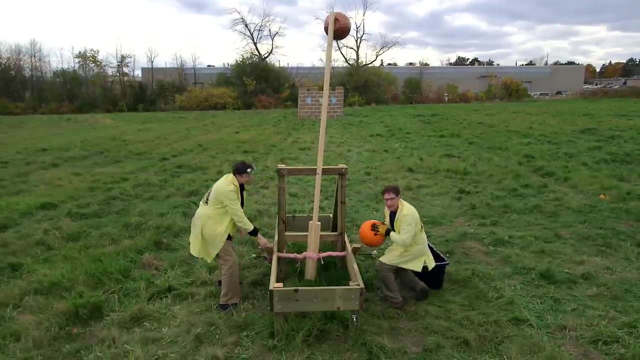 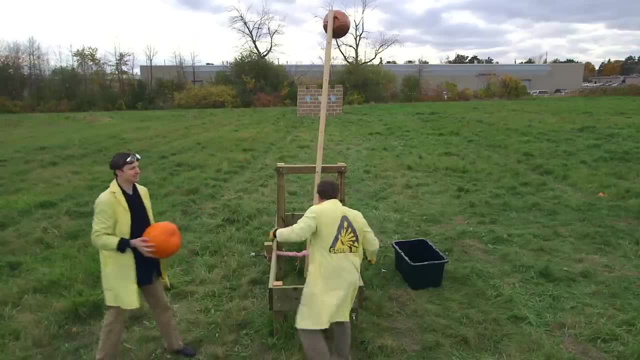 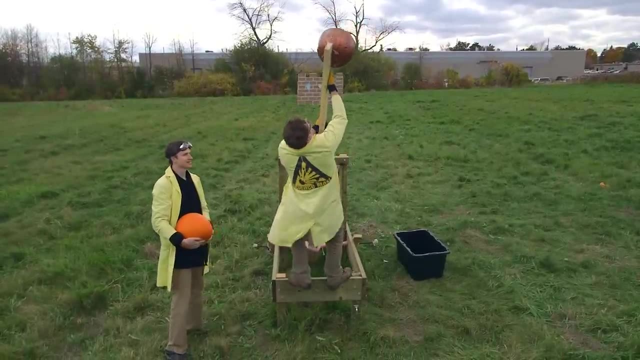 our little wall which is made out of cardboard boxes. over there, Pumpkin, All right, Here we go Pulling the arm back. Oh, Oh, That elastic force is pretty strong. Okay, How do you think we're? You think that pumpkin's? 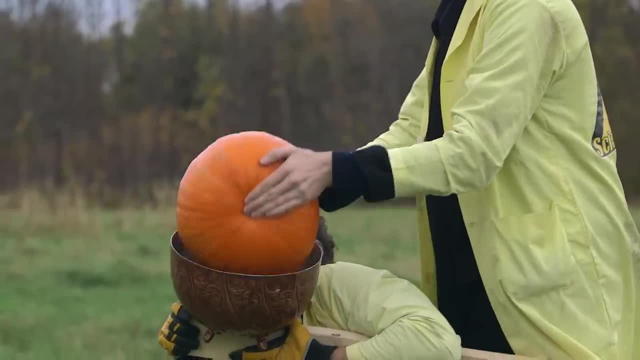 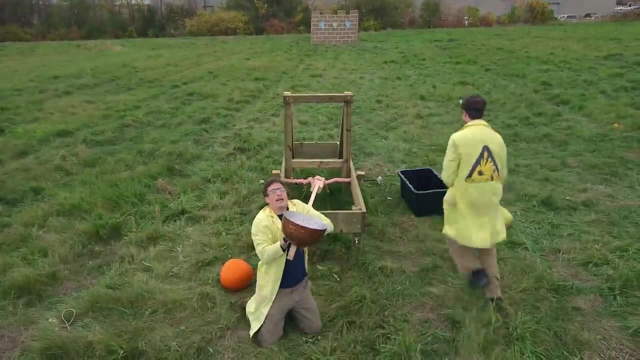 a good size. Oh, it's pretty big. You think A little too big. It's too big for our basket. Smaller pumpkin, Smaller pumpkin. I'll hold this. No rush, Zach, No rush, Okay, Rush Zach. 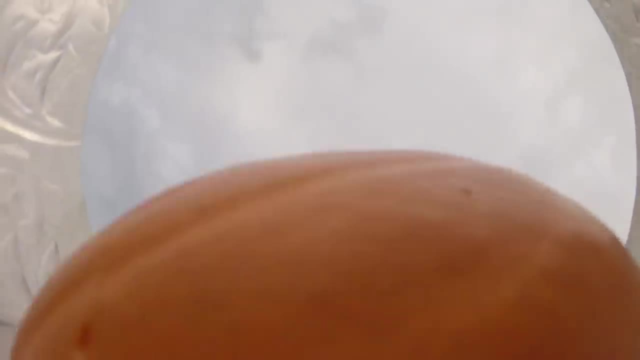 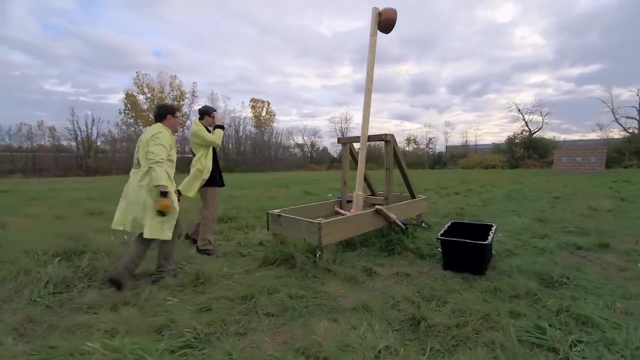 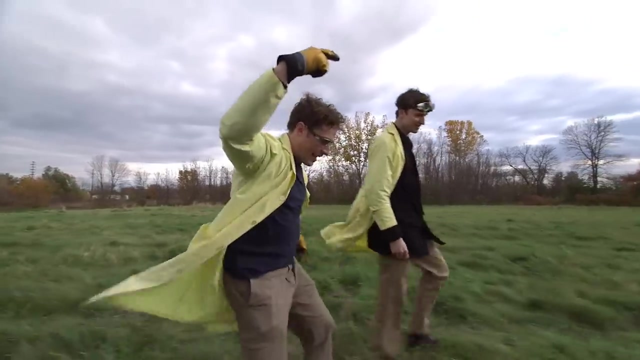 Can't hold. Oh yeah, Can't hold the arm. Okay, Ready, One, two, three. It didn't work that well. No, not quite that well, We'll see. Yeah, so it went and it flew and it landed here. 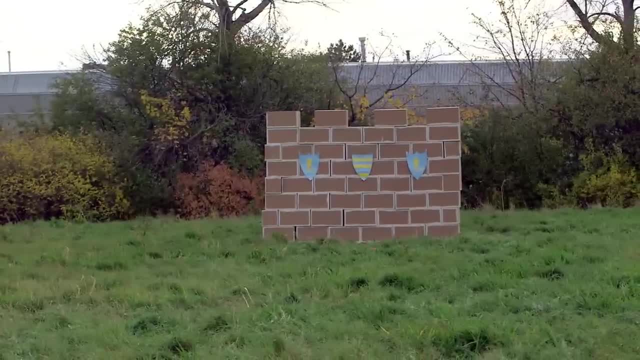 which is a little farther away from the wall than I'd like it to be. We're a little bit short One-third of the way to the wall. I don't know if that's enough. What do we do to make it better? 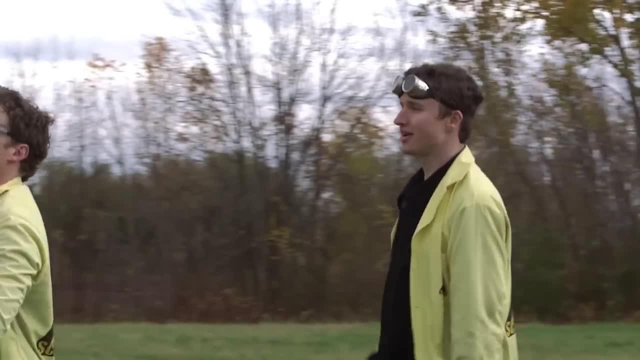 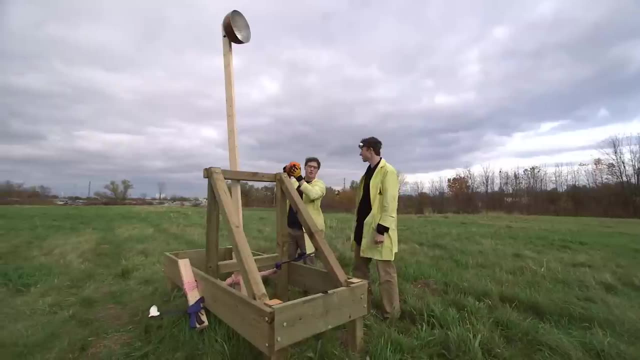 Well, the way we're throwing it right now, we just have the pumpkin at the end of the arm. So if we make some kind of a sling so that we fling it as we're bringing it up, We make a sling. Yes. 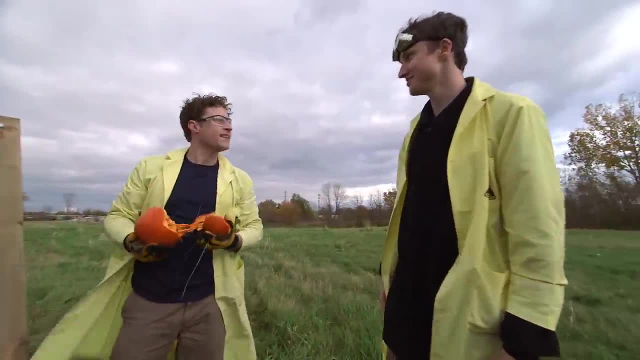 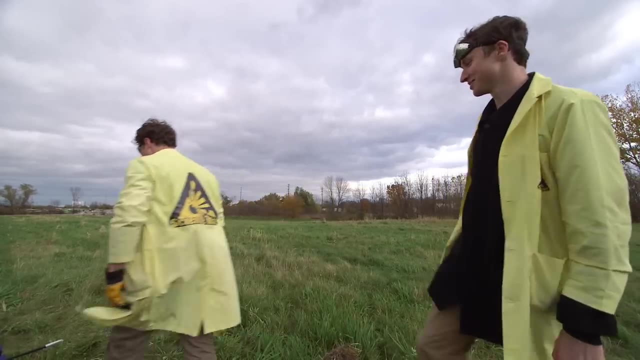 All right, I don't know how to make a sling, but you know how Sure. All right, We'll make it, and then you can explain how it works. Yeah, All right. good, Let's put the pumpkin over here. 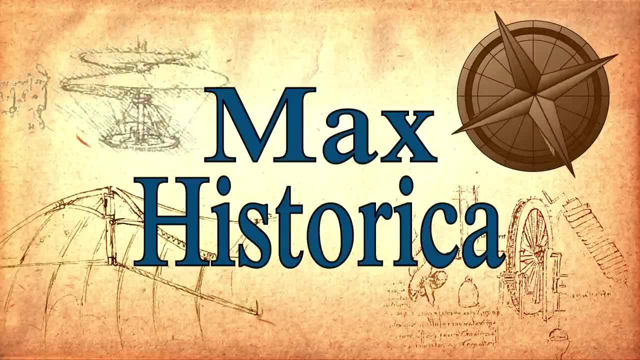 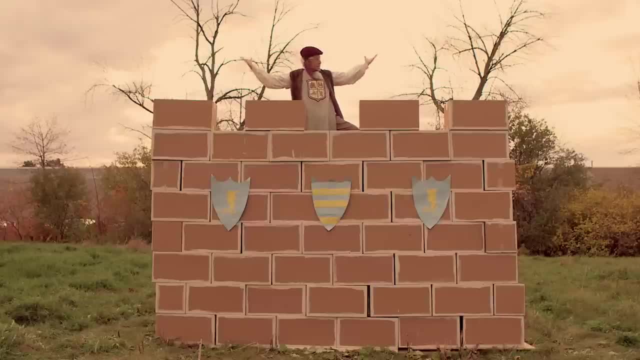 We'll recycle it later. Max Historica. Good morrow to you. I am Lord Fillington the Great. Good morning everybody. I am Lord Fillington the Third, and welcome to my medieval castle. Throughout history, lords and kings have built castles. 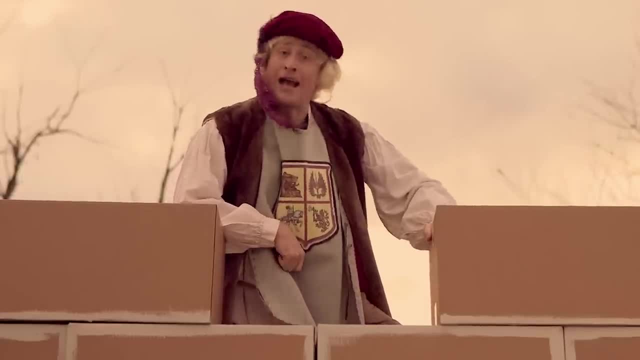 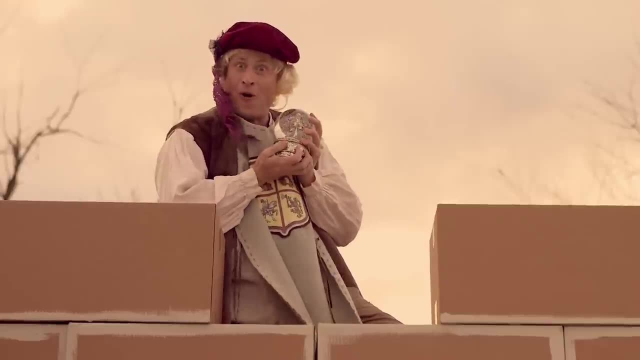 and walls to keep people out. I built my castle to protect my prize collection of snow globes. I have so very many and they're all mine, Ha-ha. Oh, hello You down there. You can't come in. 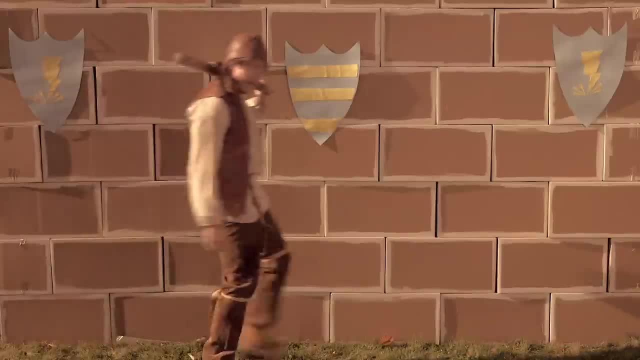 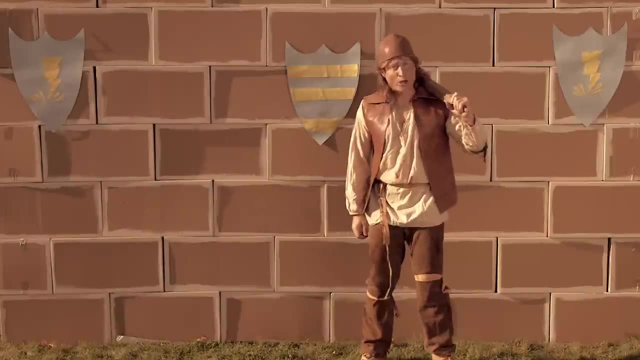 This is my castle And throughout history there have been people who've been wanting to get into those castles because Lord Fillington has been hogging all the snow globes and I Well, I'd like to look at them. But the odd part. 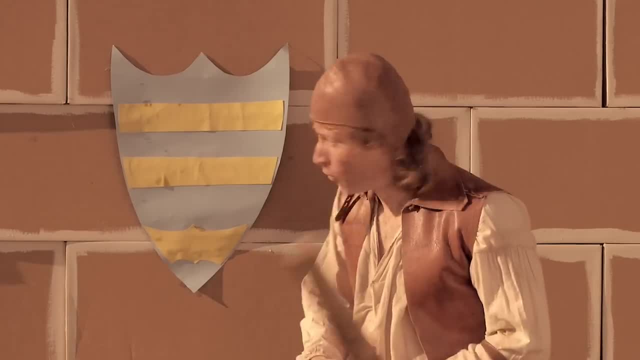 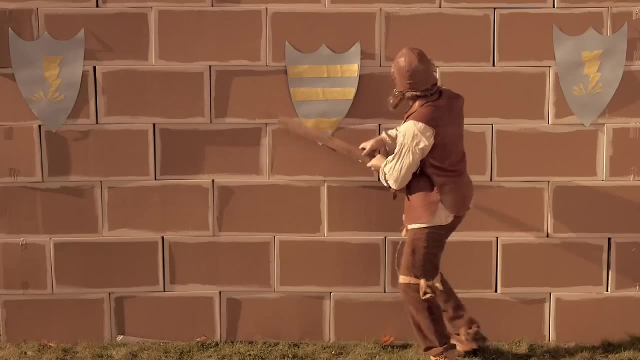 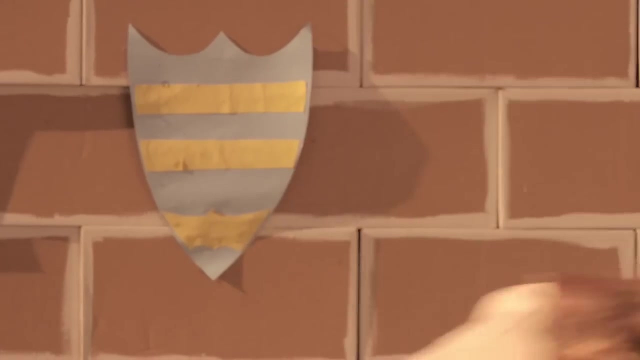 is figuring out how to get into the castle, because I can't just come up to the wall and start hammering on it. Huh, Taste the wrath of my water balloon. Because, Because if I get too close to the castle, he can get me. 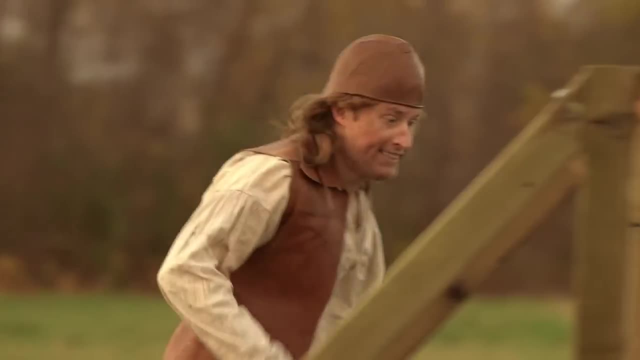 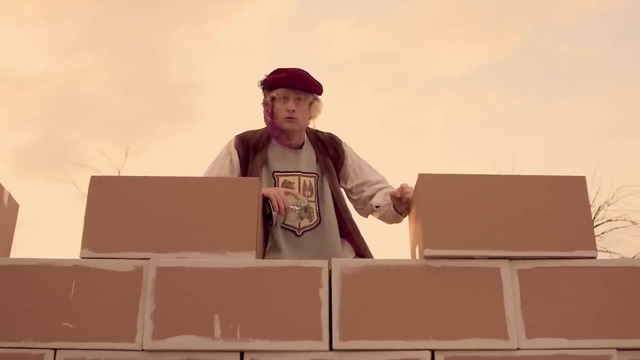 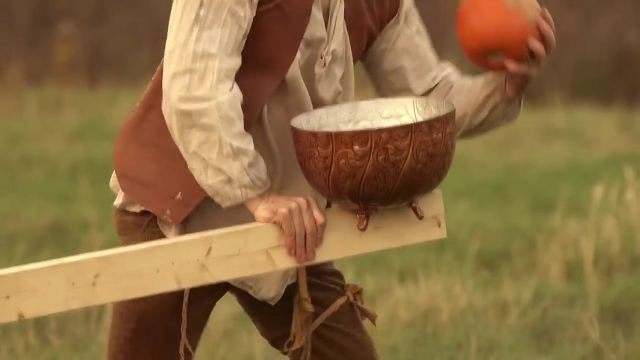 Ha-ha-ha-ha. Fortunately there's this thing called a catapult. Oh, fiddlesticks, They have a catapult. What you do is you put something heavy in the end here and the catapult fires it at the walls of the castle. 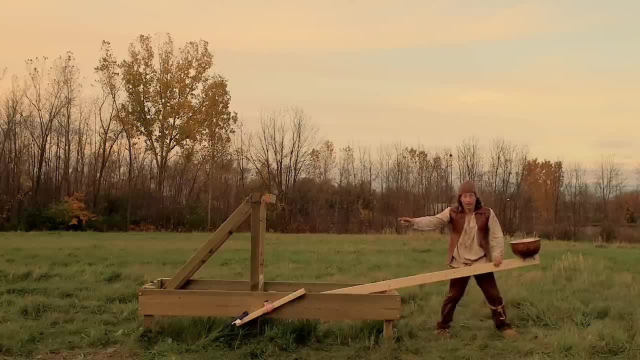 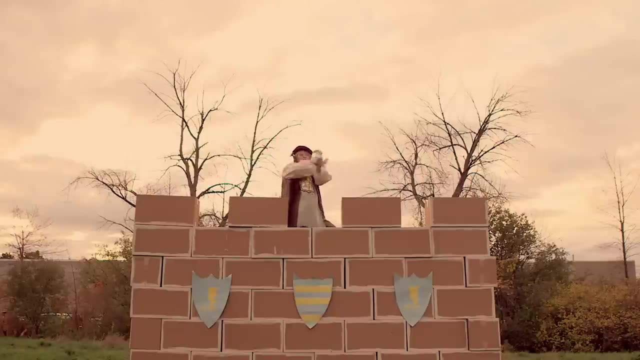 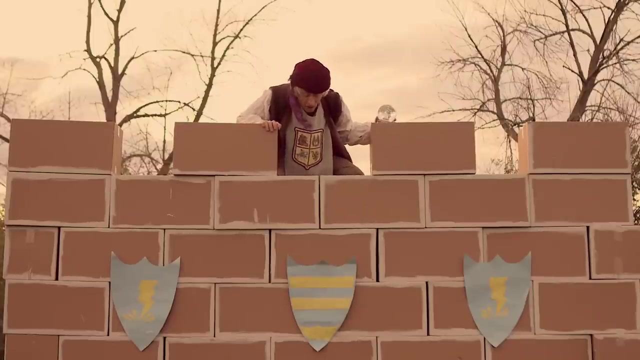 knocks them down, all from far enough away that the people in the castle can't get to you. Ha-ha, Oh, I surrender. Don't knock my walls down. It'll take me all week to fix them. Oh, All right, all right. 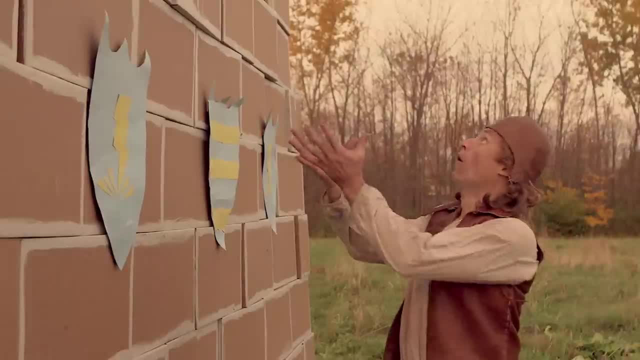 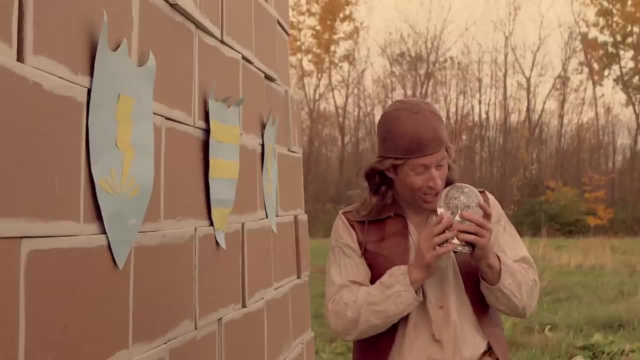 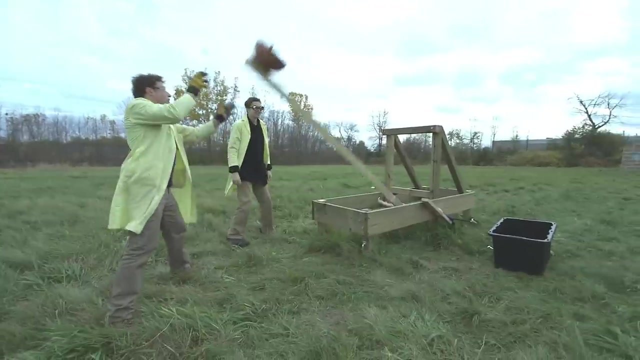 you can have a snow globe. Ha-ha-ha. And that's how catapults were used in history. Oh, so beautiful. Back to our maxed-out catapult. Our first design threw a pumpkin, just like it was supposed to, except it only threw it. 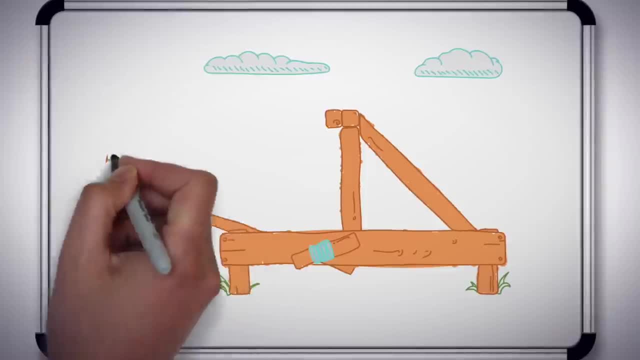 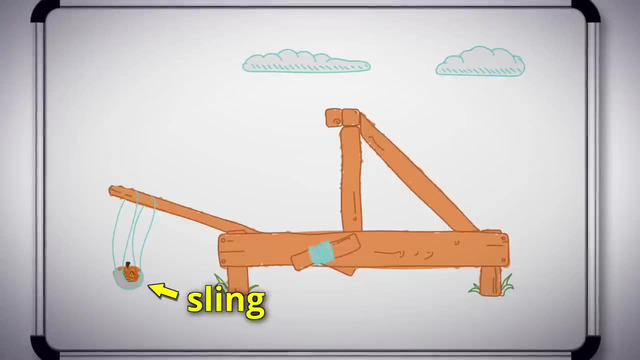 one third of the way to the wall. Now Zach and I are planning to outfit the catapult with a sling. The sling attaches to the end of the throwing arm and gives the pumpkin a lot more distance to travel, Because the pumpkin is traveling a longer distance. 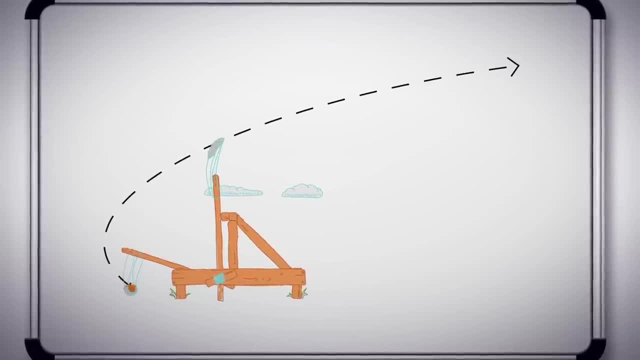 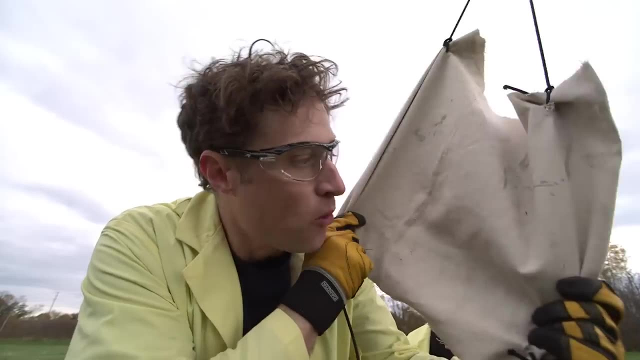 in the same amount of time. it will be going faster, which will hopefully get it to the wall, or at least a lot farther than before. So we built this sling. How does this work, Zach? Well, we've got one end tied here. 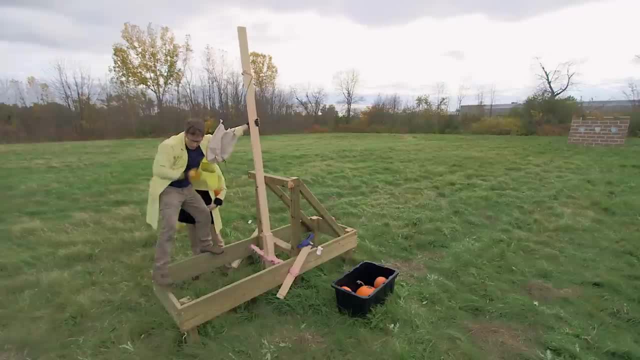 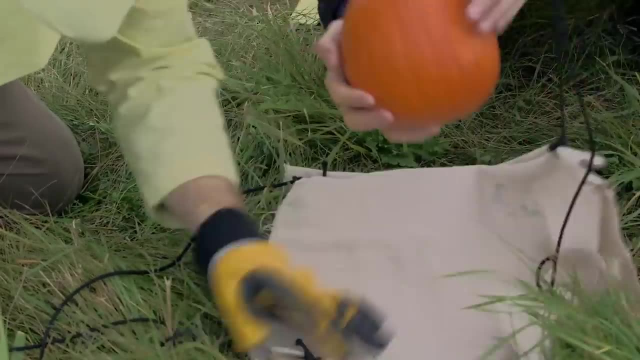 Yeah, And then we put the pumpkin in here. Wait, wait, Okay, pulling arm down. Pulling arm down, Okay, yeah, now, what? Now we put the pumpkin in here. Put the pumpkin in there, Yeah, Then we loop this. 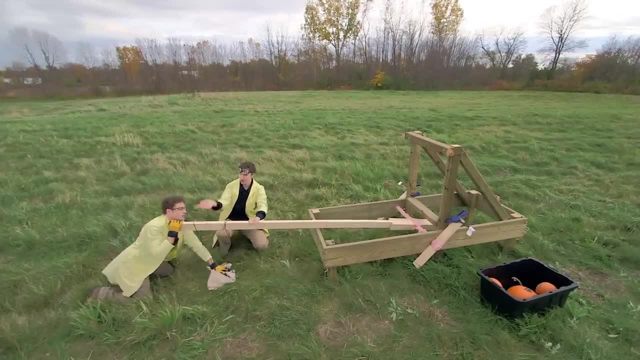 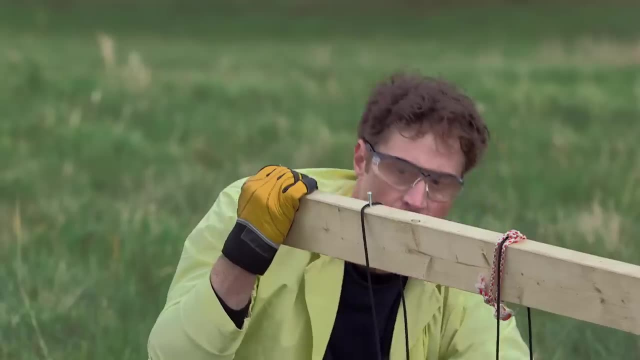 over the back of the Oh, Over that, As the throwing arm goes up, this will slide off the back of the throwing arm and it will release the pumpkin. All right, You're the expert, I believe you. Let's try it out. 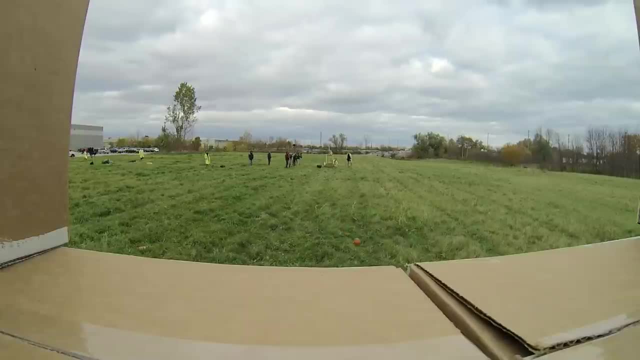 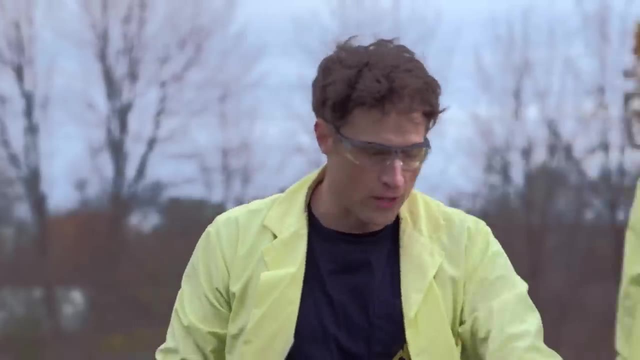 Three, two, one, Oh Whoa. Okay, That works really well. You know what the problem is, though: We don't have enough oomph. Yeah, it needs more power. So what do we do? I don't know if we can. 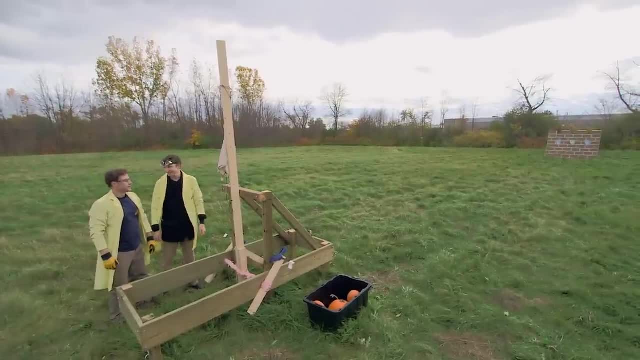 crank that rope anymore. I think we're at the limit of our rope power. but if we added some more elastic, I thought we weren't going to use elastic. Well, we used elastics in our small demo models. What if we used some more? 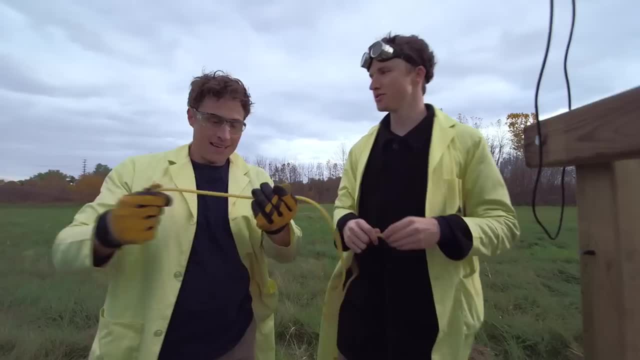 Do we have elastics? I don't know if we have. Yeah, brought some in here just in case. What's this? It's surgical tubing. It's like a giant elastic Mm-hmm. Well, I guess this is elastic force. 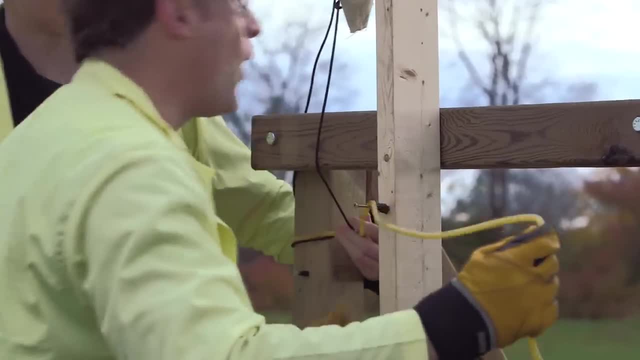 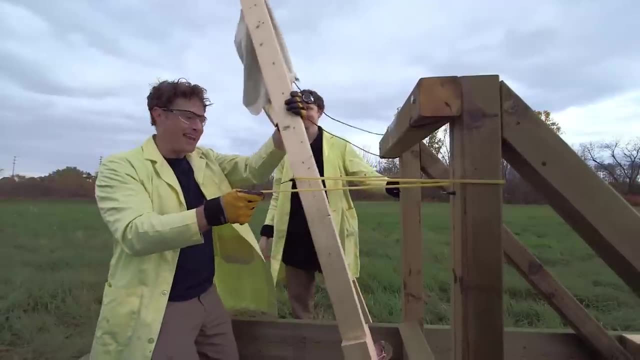 so do we twist it around at the bottom there? Well, we just wrap it around the throwing arm like this: Yeah, we just need a lot more, and then, And then we pull this and it would be: Oh, yeah, Yeah. 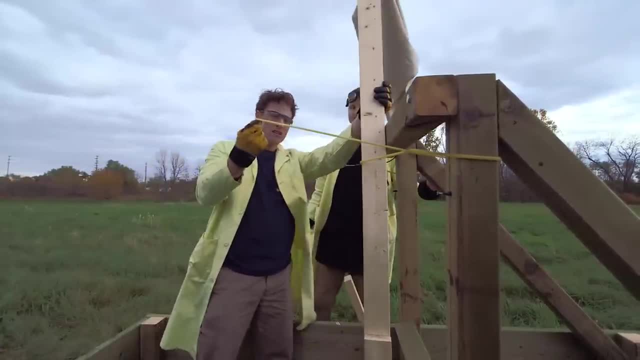 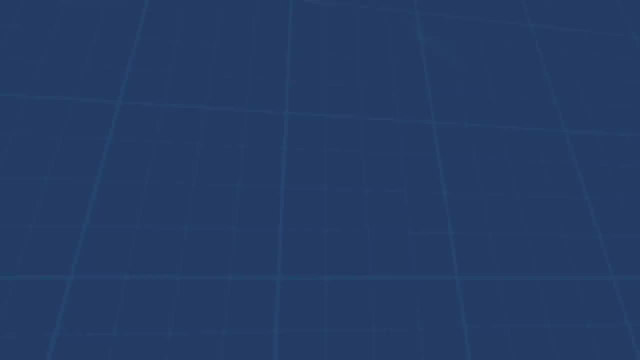 That would make a lot more. So we just need a lot more of this elastic. What is this again? Surgical tubing, Surgical tubing. It's like a giant elastic. Fantastic, All right. Goggles on, Goggles on, Yes. 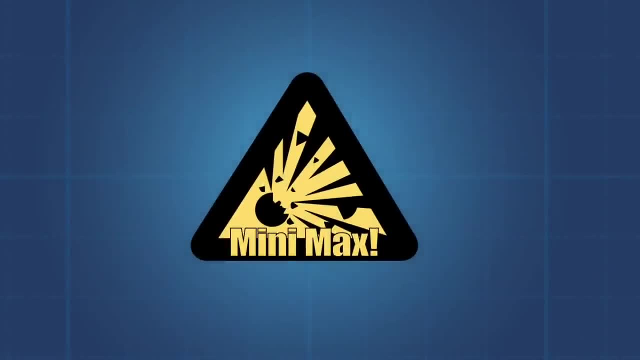 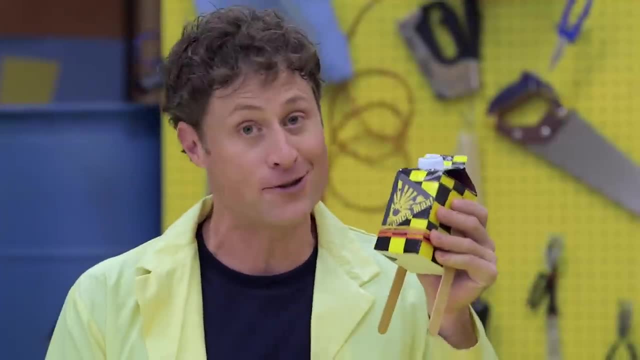 Yes, Here's another fun way you can play with elastic force. Take a milk carton. I prefer Science Max milk because it's the creamiest milk carton in the world. It's made by a chemist- 2% cream. 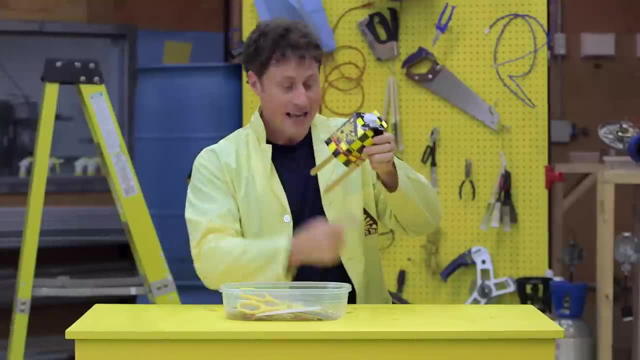 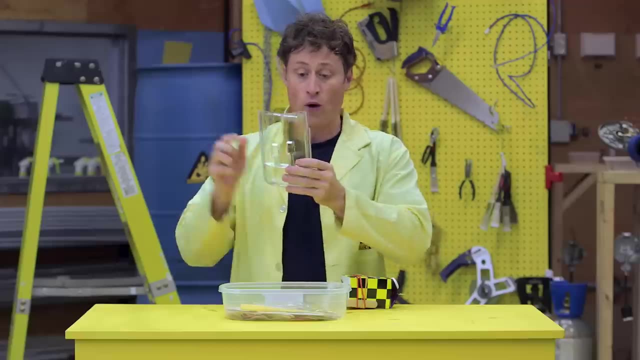 100% science. Wrap some elastic bands around it with some popsicle sticks on the bottom, sort of like feet. Then take some clamshell packaging, which wraps just about anything you buy nowadays, and cut out a square or a rectangle. Then wrap some tape. 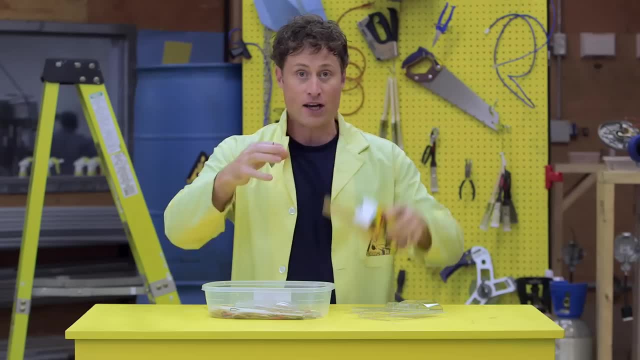 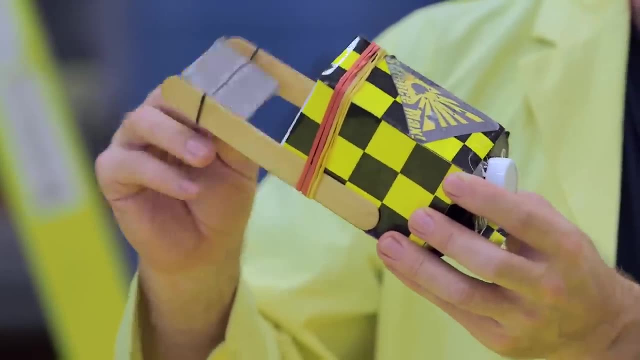 around that square with an elastic in it and put the elastic on the feet of your milk carton, Then wind it around and make sure you go backwards so your paddlewheel boat will go forwards when you put it in the water. And there you go. 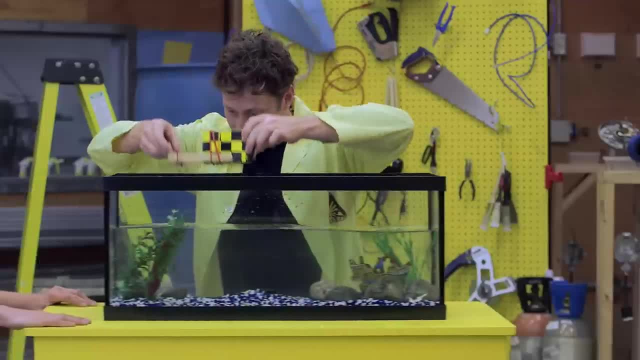 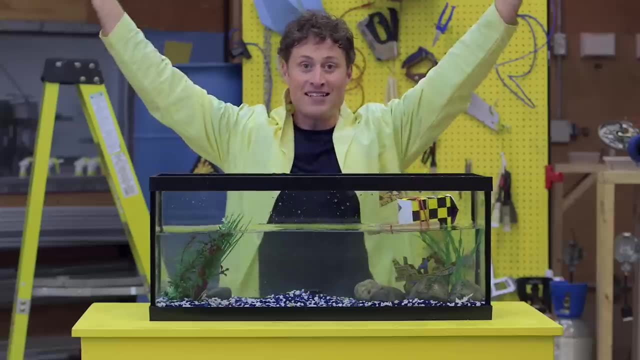 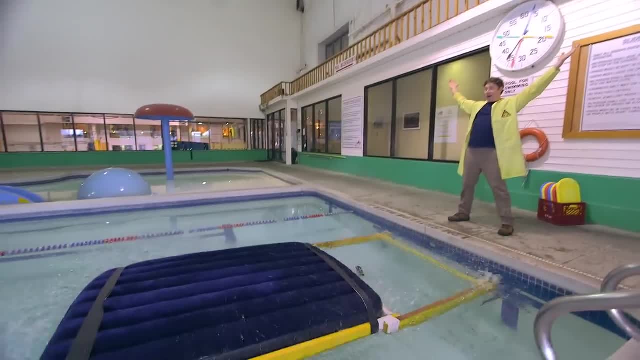 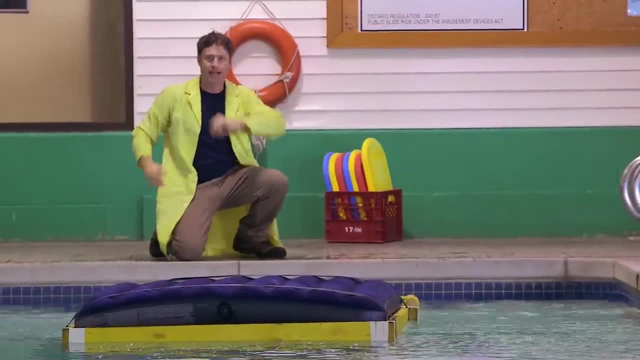 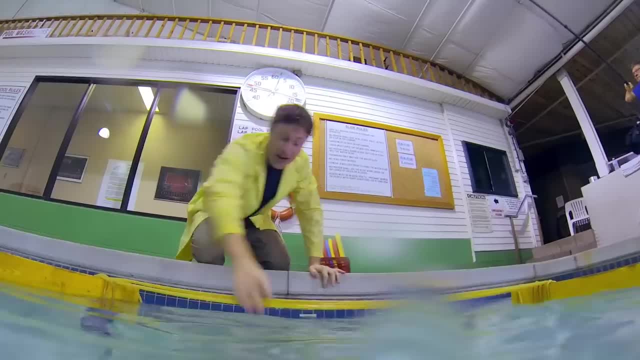 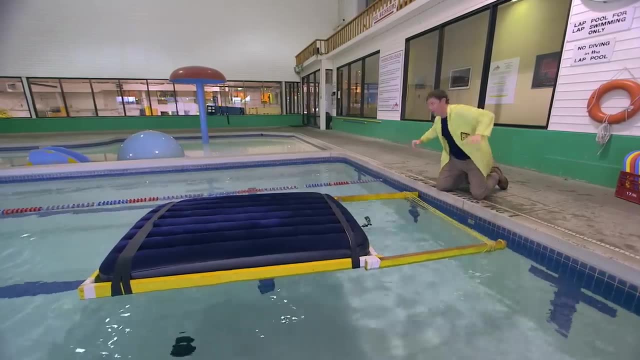 a giant paddlewheel boat that will work on elastic force, because I've got surgical tubing as my elastics and that's an air mattress, and then I use some lumber to hold it all together and of course, I need a paddlewheel. and what better thing to use in a pool? 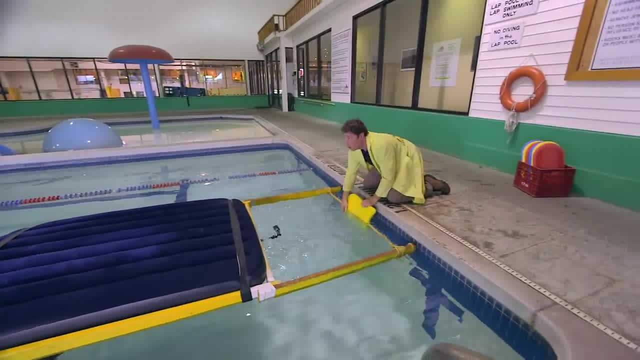 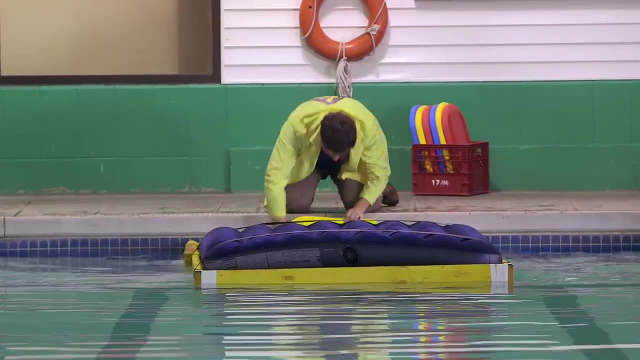 than a flutter board. OK, Here we go. So normally you're not allowed to wear your clothes and your shoes in the pool, but I got special permissions. Besides, I'm not worried at all, so I didn't wear my swimming outfit because I figure I 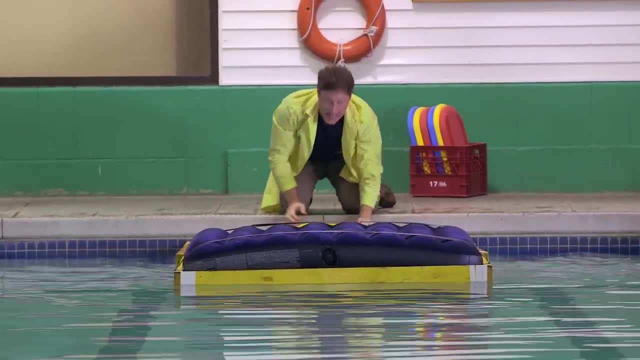 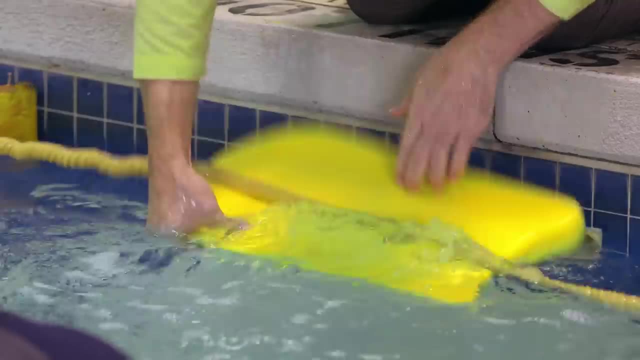 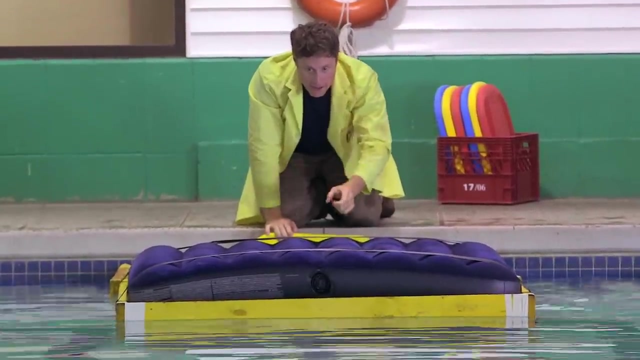 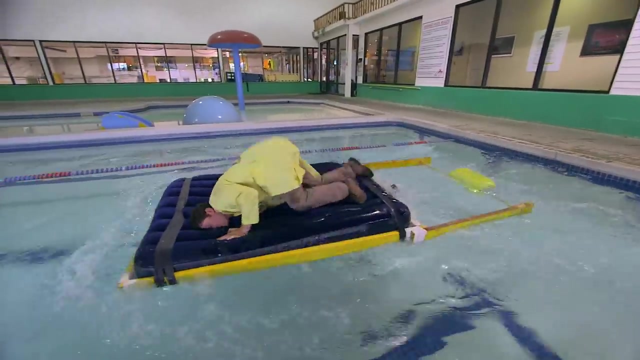 can totally do this entire experiment without even getting wet. That is how confident I am. Alright, now the tricky part. we'll be getting on to the mattress. Okay, here we go. Haha, Haha, The SS Science. 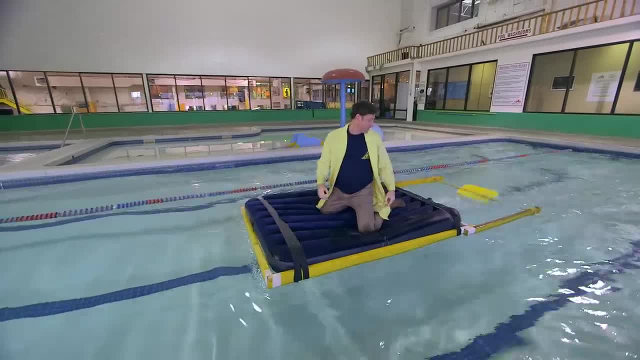 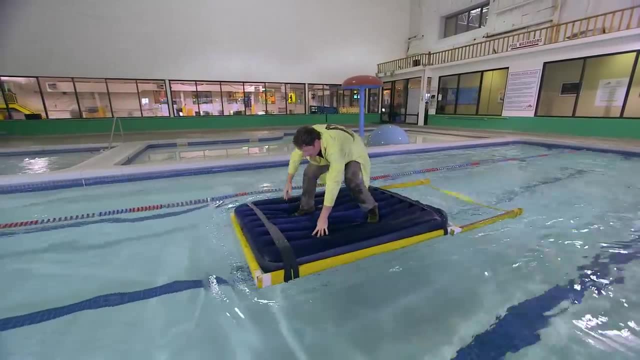 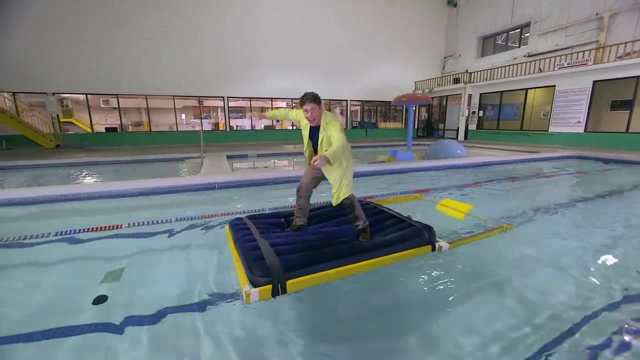 Hey, SS Science, that's a great name for this. Look, it works great and I managed to stay totally dry. Huh, Well, almost Haha. you thought I was going to fall in the pool, but I didn't. 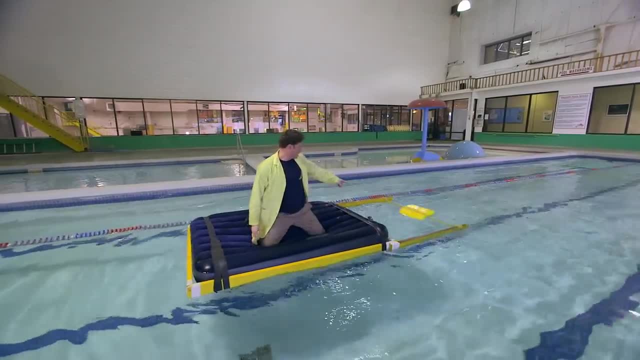 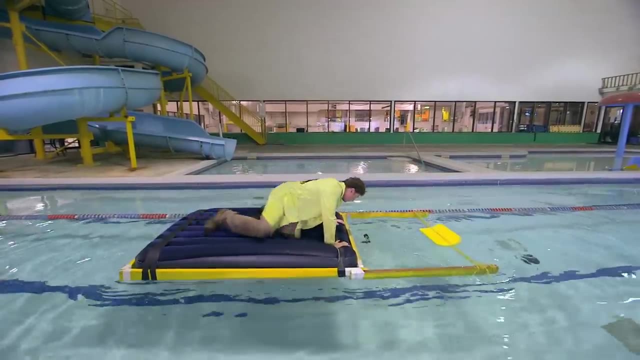 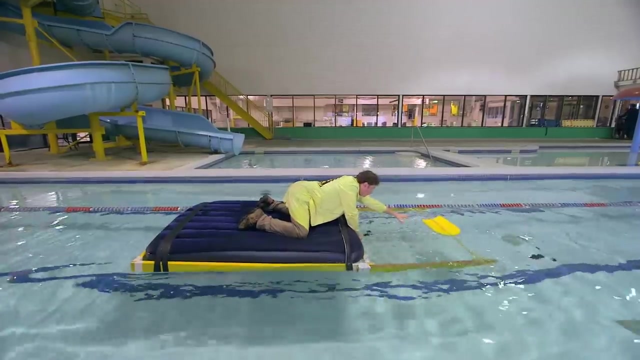 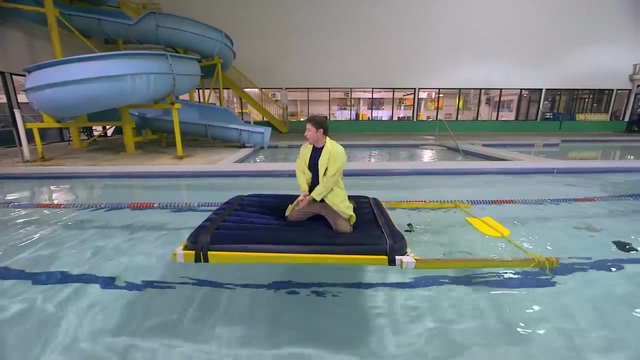 Uh-oh, My flutter board has stopped moving and I'm in the middle of the pool Almost. Yeah, Didn't think this through. No, No, No, No, that's not going to work. Maybe I'll, Maybe I'll wait. 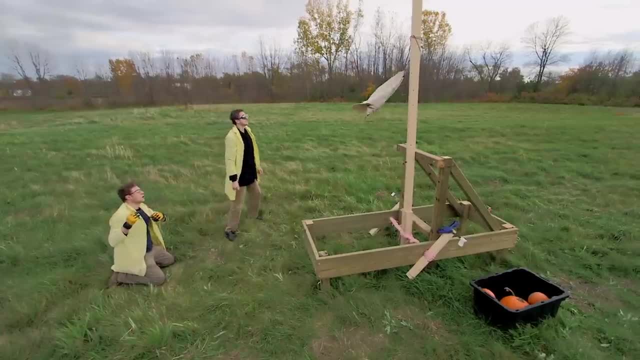 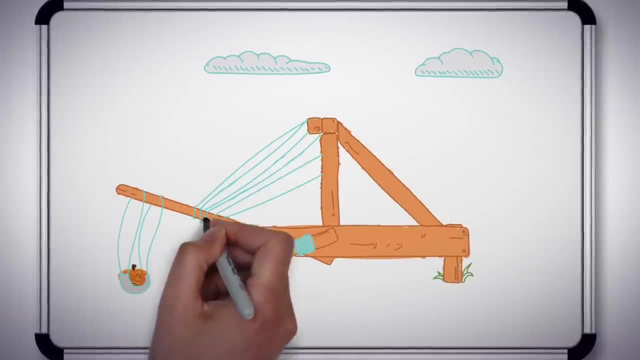 Our maxed out catapult was working well with the sling we attached to it, but it still didn't make it all the way to the wall. Zach's idea is to attach a bunch of surgical tubing to the cross piece of the catapult. Surgical tubing is pretty much big elastics. 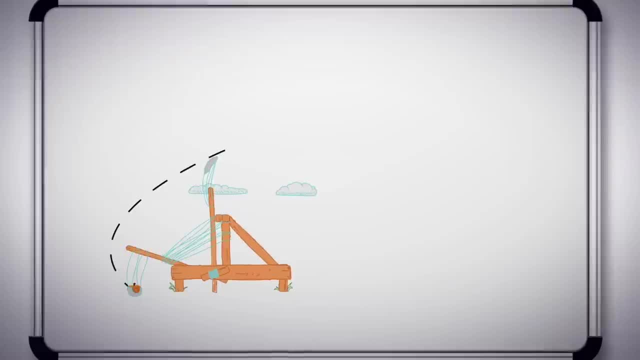 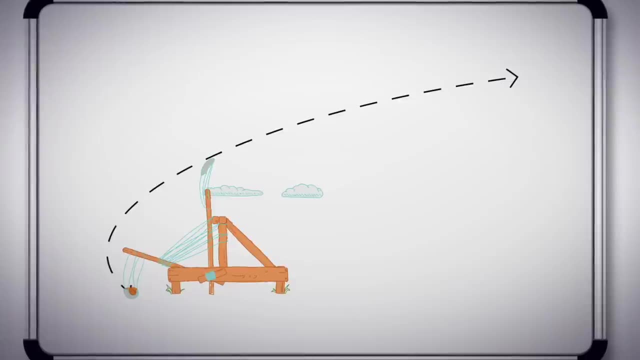 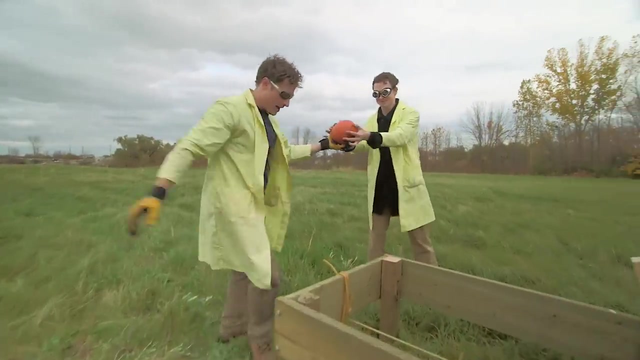 so we'll have two places. we're getting elastic force from the rope and the surgical tubing. Hopefully this design is enough to help our catapult fling a pumpkin far enough to hit the castle wall. All right, here we go. Uh, you hold that. 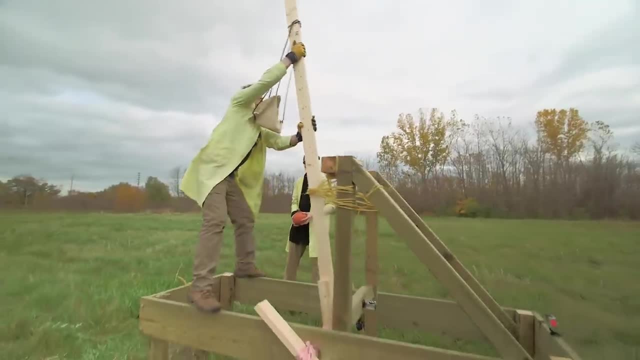 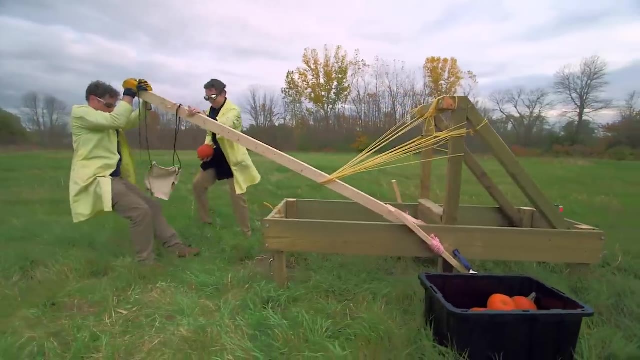 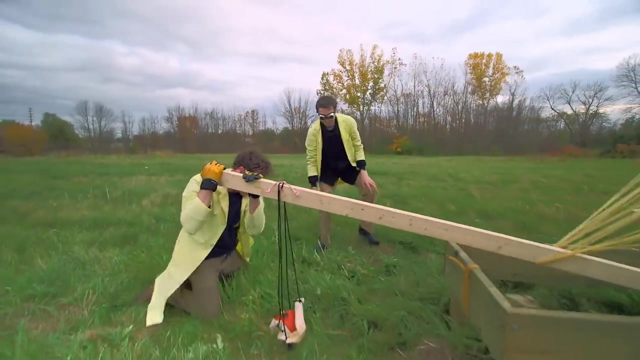 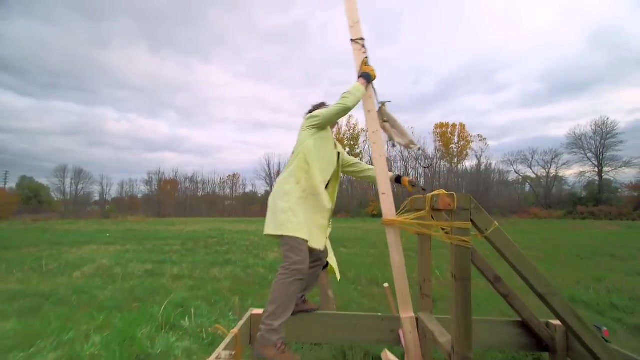 I get this. We got our system down. now, Okay, This goes up to there. Okay, Okay, Three, two, one, Nope, Hahaha, Huh, Nice one, Zach. We did it, We did it, We did it. 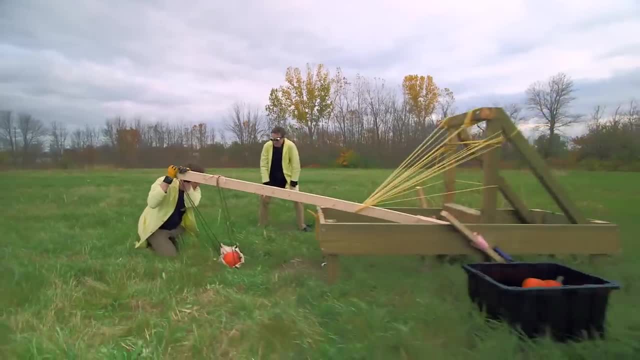 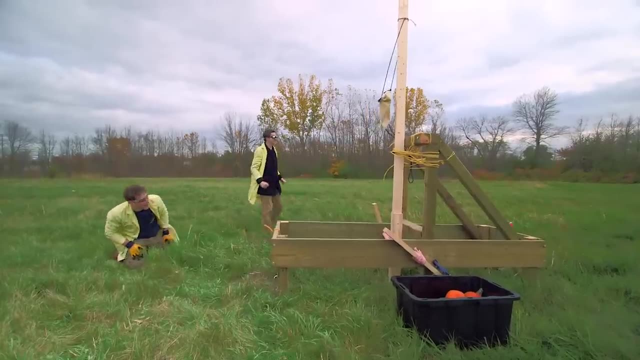 All right, Let's go. One, two, three. One, two, three. It went too far. It went too far. That's so good, Oh man, All right, Okay, So all we got to do is move the catapult back. 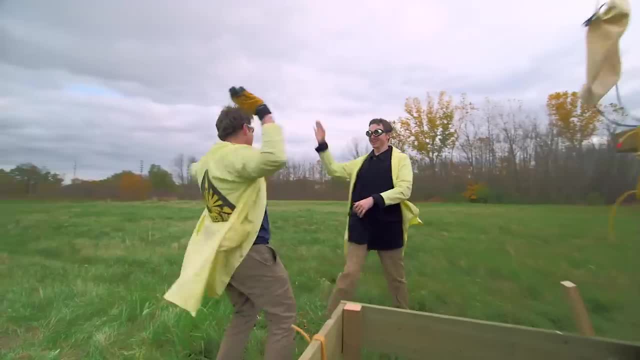 So you get that side, I'll get this side And we'll move the catapult. See, now, our catapult is too good, We've got to back it away from the castle. All right, Let's go. All right, Let's go. 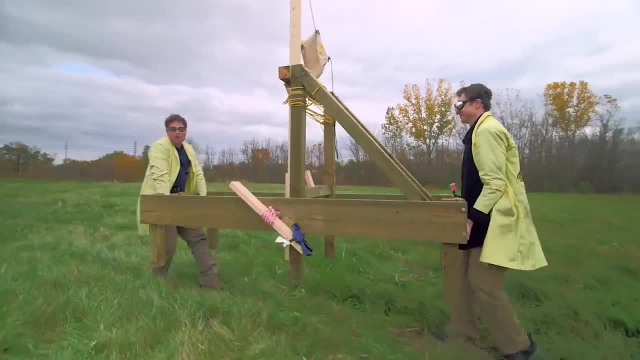 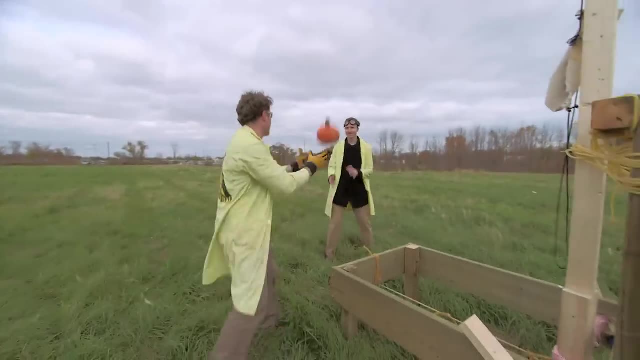 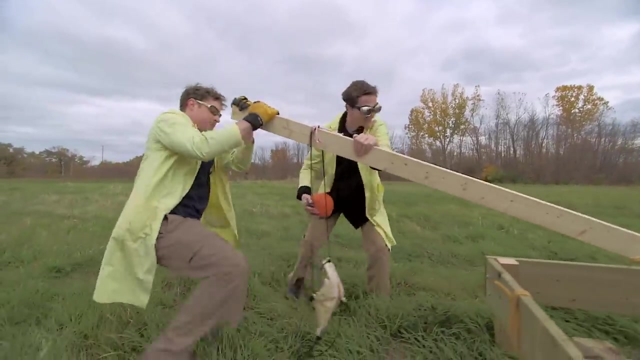 All right, All right, All right, Let's go. All right, All right, let's go again. Pumpkin, Pumpkin, Pulling arm back, Pulling arm back, Grunting Loading. pumpkin Hooking rope on arm, Hooking rope on arm. 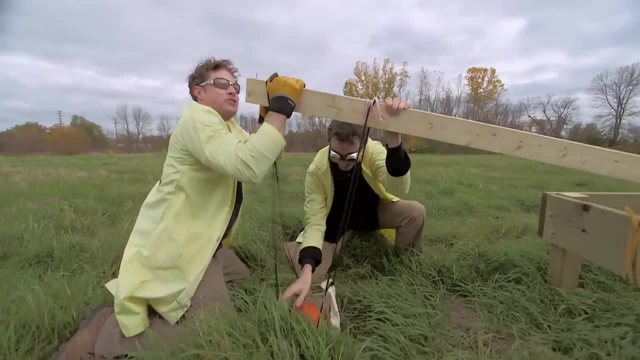 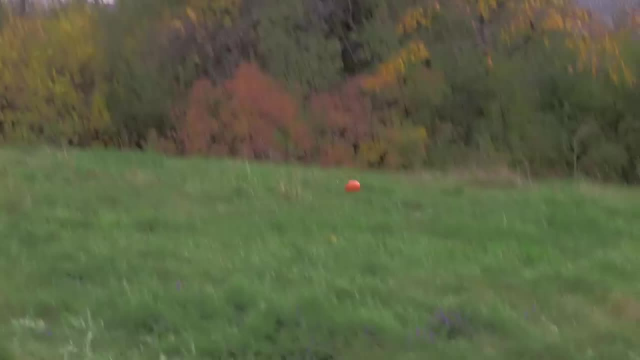 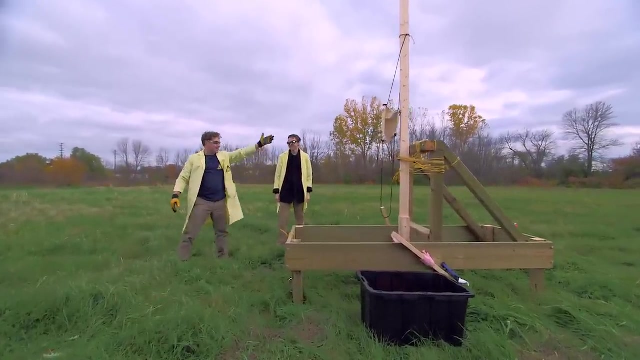 More grunting, More grunting, Pulling back strongly, One, two, three, Oh Oh, Oh wow, Whoo, Whoo, We're inside the castle. We're still inside the castle. Oh man, That's an excellent shot, though. 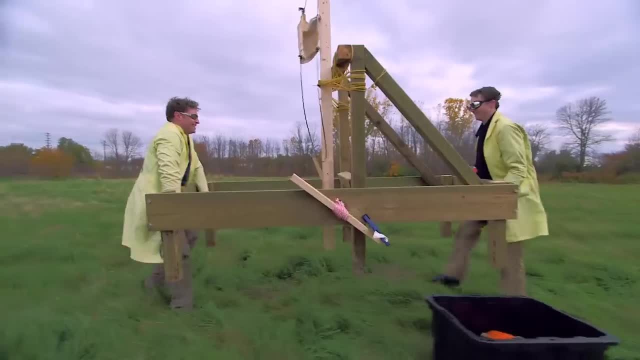 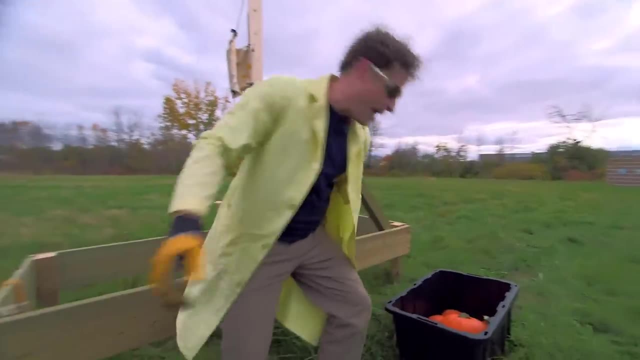 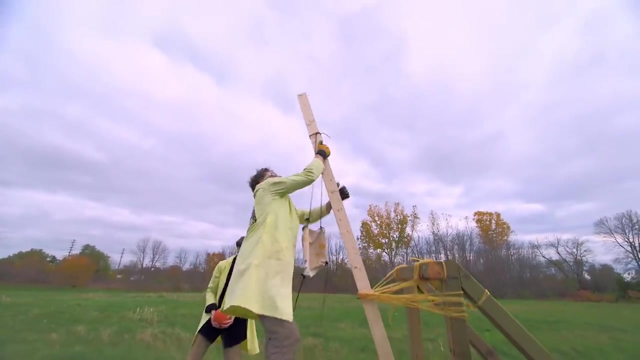 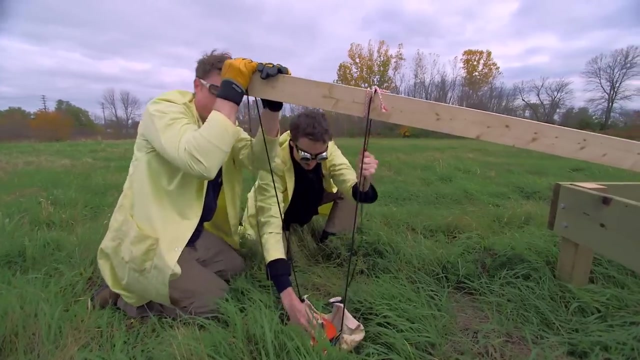 So what do we do? Move the catapult back. Yeah, Move the catapult back. What about here, Here? Here we go again. Pumpkin, Pumpkin, Loading, arm, Loading, arm Beautiful. All right, You ready, You think it's going to work? 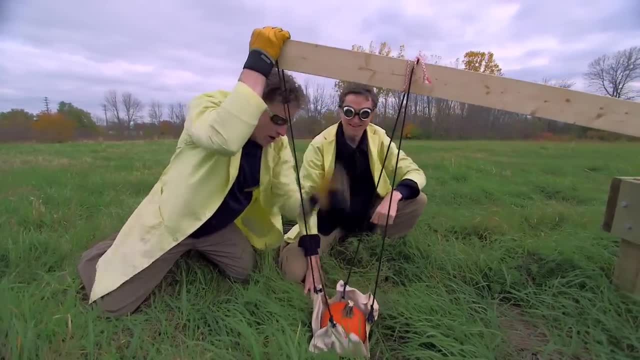 We've got every modification we can possibly do, So you think it's going to work this time. We did it. It's going to work. Okay, here we go. I'm excited, All right, Ready, Ready. One, two, three. 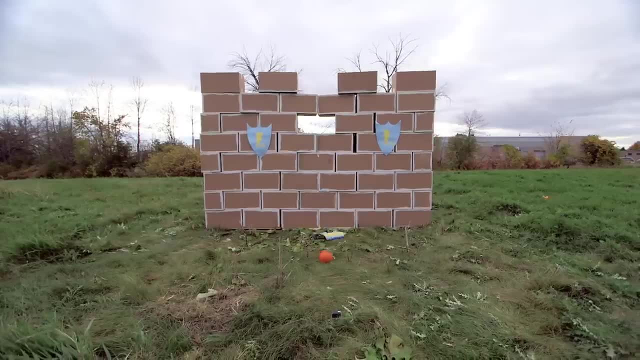 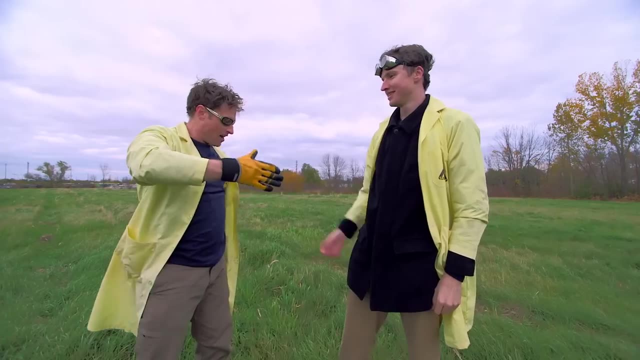 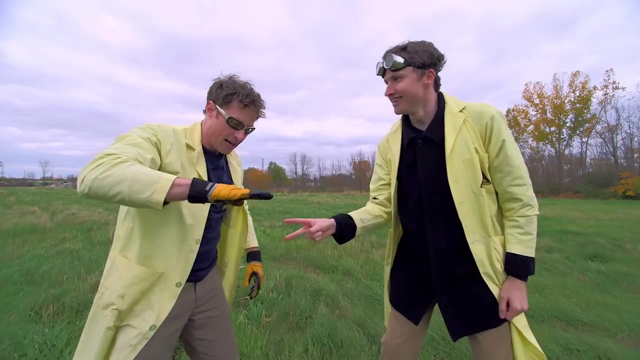 Whoa, Yeah, Whoo-hoo, High fives. Well, there you have it, Awesome job. Now we need you to throw fingers to see who gets to rebuild the castle. Okay, One, two, three, Oh. Thanks very much for joining us. 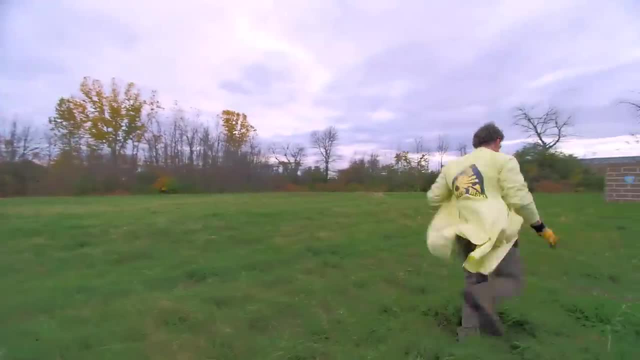 Just take a break. I'll rebuild the castle. You see, this is exactly how catapults used to work. They'd hit the same part of the wall over and over until they made a big hole, and that would weaken the wall. Fortunately for me, it's really easy to fix. 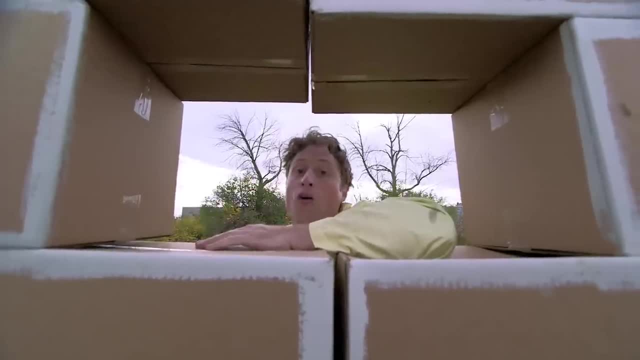 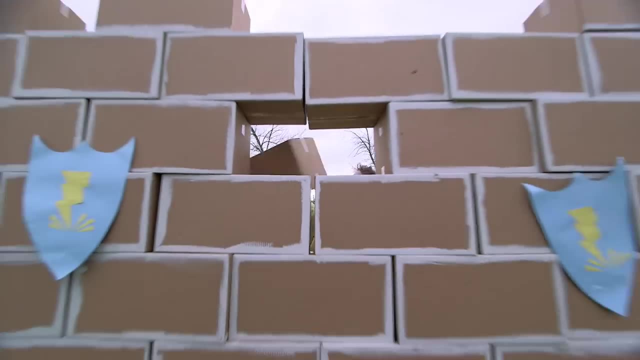